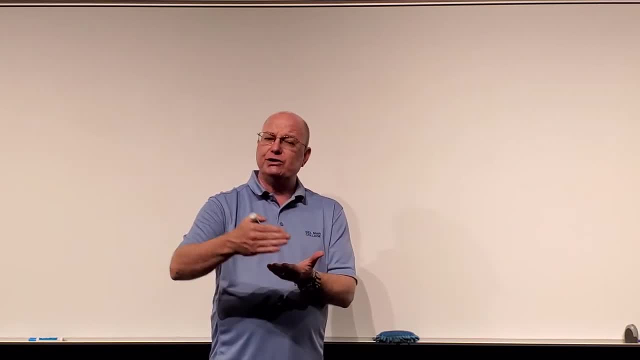 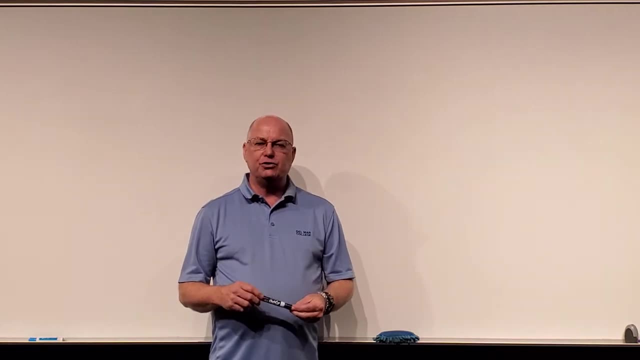 number of didactic or classroom learning and certain number of hours in clinical, And when you add all that up plus the prerequisites, it would require about 72 hours or more. And those prerequisites very often are necessary to help you understand the information that. they're going to be going over in the program. Well, politicians decided: well, you guys are getting rich, making them take extra hours, cut it to 60.. But technically and legally they can't cut the hours of the program, so they started cutting prerequisites. 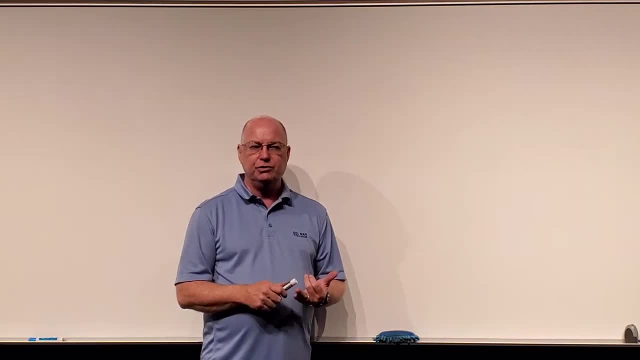 And so now it's not even required that you have some freshman biology one and two, and they're trying to even strip freshman chemistry as a prerequisite, which hurts the learning in microbiology. Now, many of you may have had some biology before or some in high school, but a lot of our students 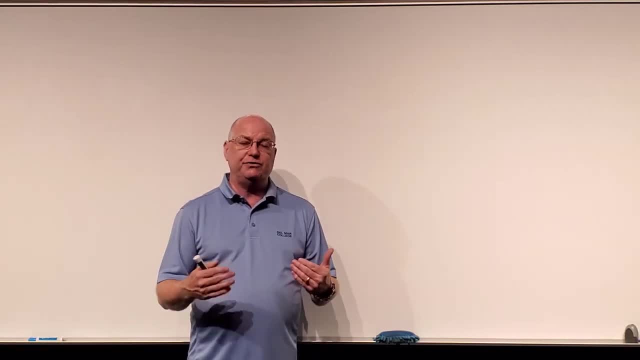 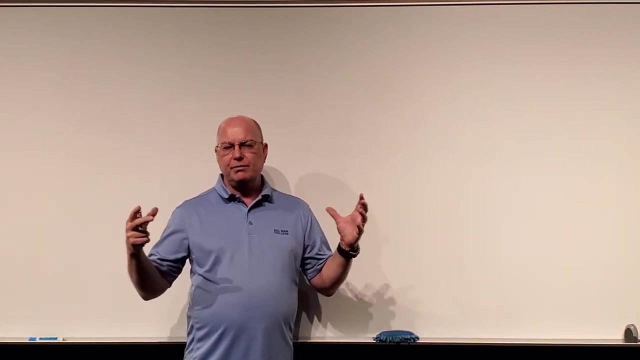 especially at the community college level, are coming in to sometimes 5,, 10,, 15,, 20 years after high school, and now they're not required to have these other biology courses, And so I have to step back in order to understand microbiology. so we're 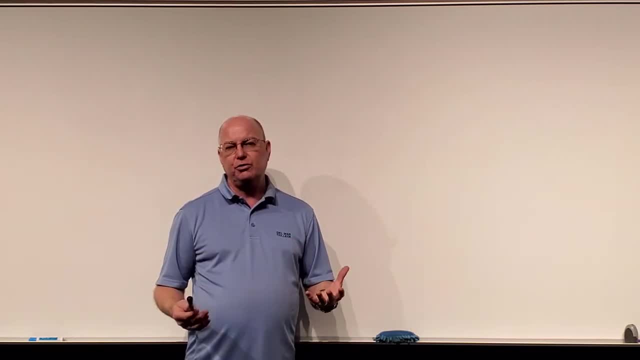 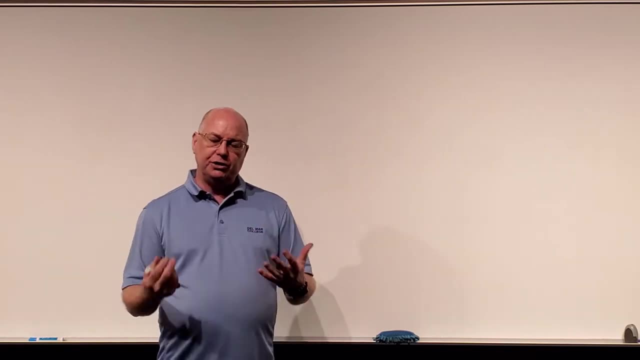 going to take a step back into some freshman biology. we're going to do a lot of terminology as we go through this first lecture. So microbiology is a subtopic under the, the super topic or the subject of biology. so if I 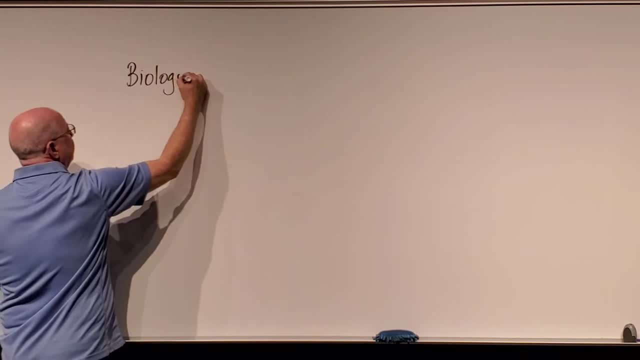 look at the term biology and I'm a big word nerd. I like to break down words and knowing roots and suffixes and prefixes over a possessions, because the seeds are over there. But I'm a big word nerd. I use the absolute quotes for tools if they're only words ovals, they are only words ops. So I can diction pot an attribute. something gives theongo lots of focus and it's not like you're EXPlainnotes. you aren't so in the specialty, Anakin Gates is trying to explain a word and that it might help back some lessons you do. 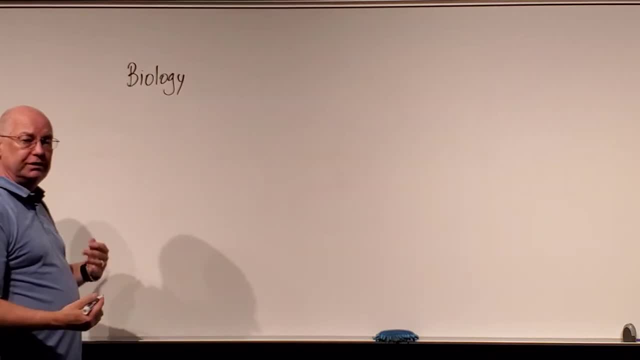 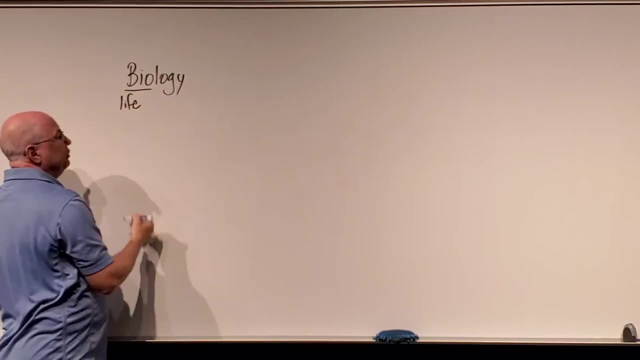 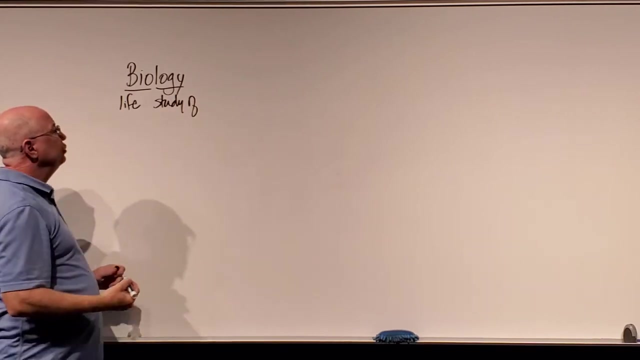 helps you sometimes answer questions and understand material. it's really a lot of language. it's a lot of vocabulary. bio literally comes from the word bios, which means life, and logos or ology means the study of or the logic of. so biology is the study of life, the study of life processes and all everything associated. 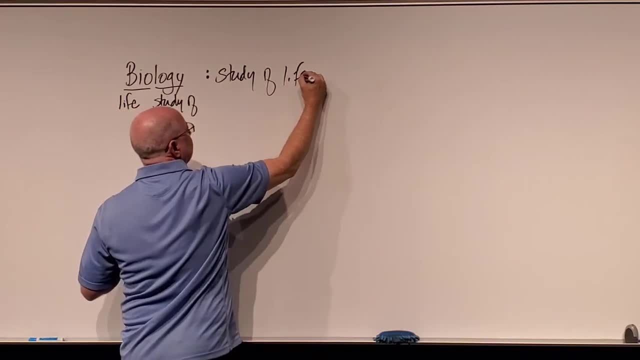 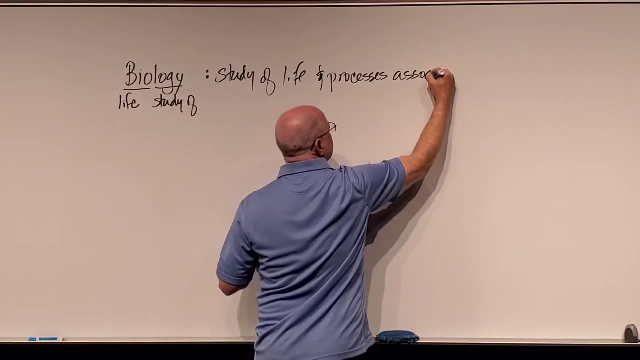 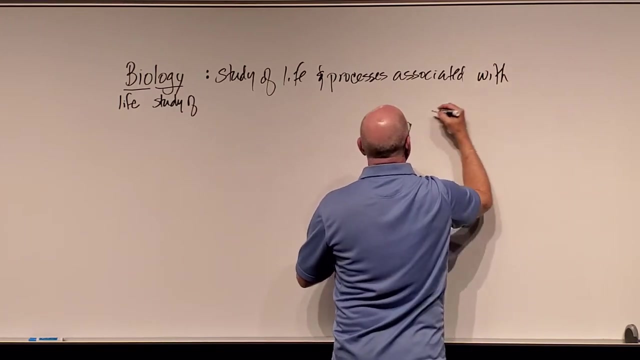 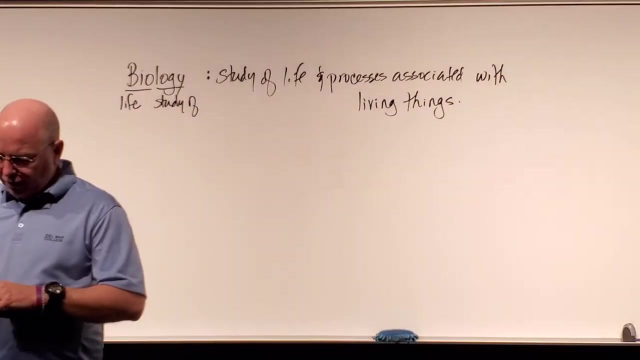 with life. it's the study of life and the processes associated with living beings. okay, that's kind of a broad, general, general definition, but it is a good one. okay, so that's what biology is. microbiology is a subtopic under biology which has a whole myriad of topics that we could study. 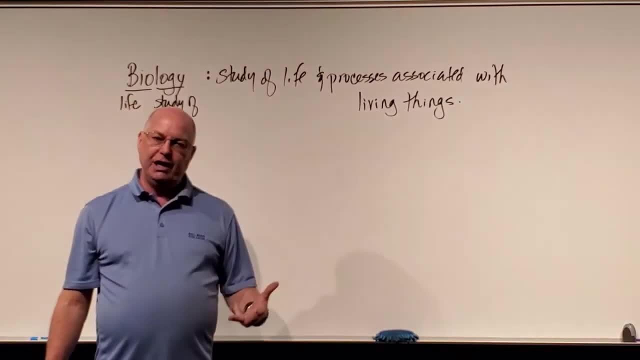 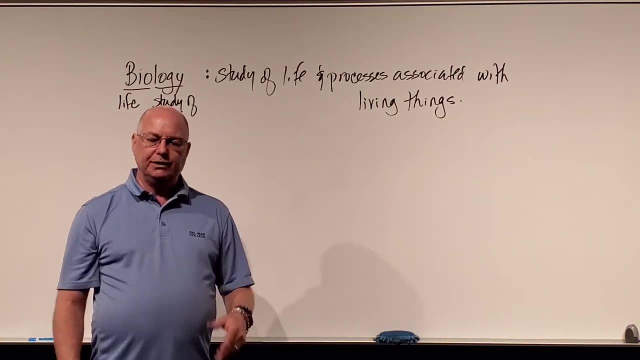 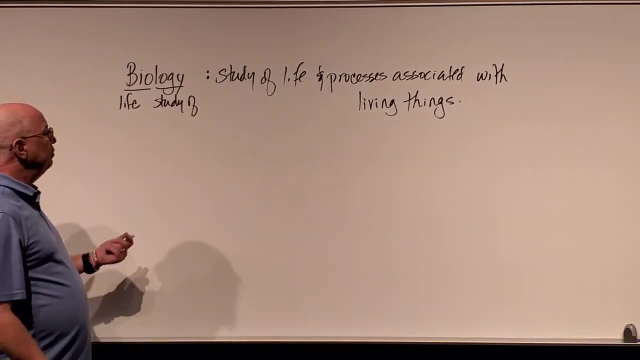 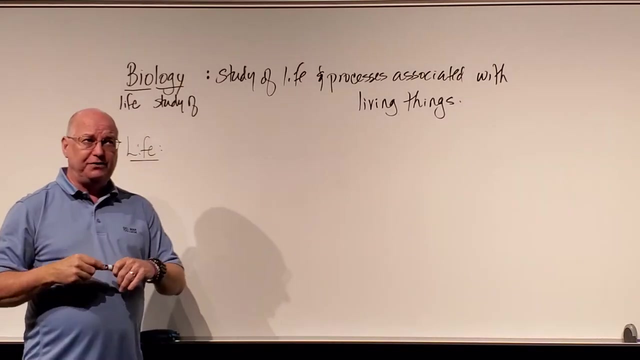 ideology, anatomy, physiology, genetics, biochemistry, microbiology, I said etiology, ornithology, you know all sort, all these ology so we can study. now, in order to understand all of this, we have to understand what is the definition of life. okay, now scientists have a very hard time defining life. I'm gonna read. 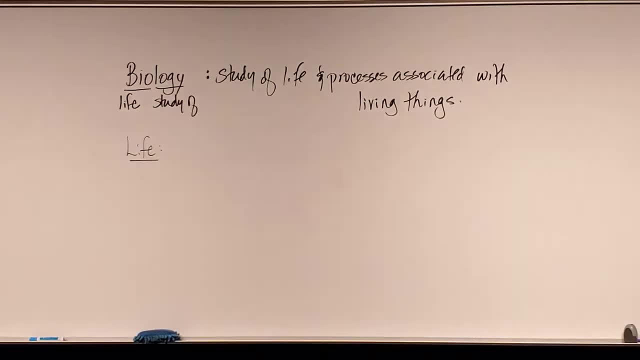 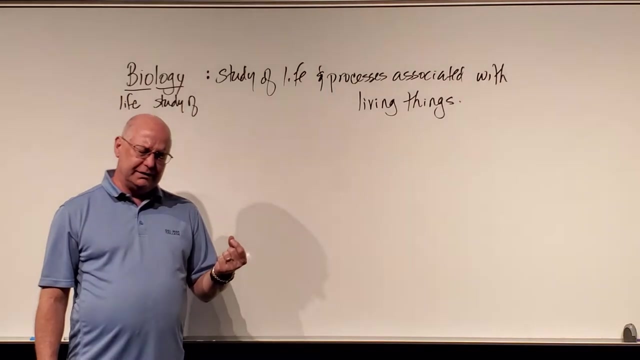 you a definition from a textbook of life. life, A living thing, is a physical entity that exhibits characteristics that distinguish it from non-living or dead things. Life is a physical, or living things are a physical entity that are comprised of characteristics that distinguish them from non-living things. What in the world? 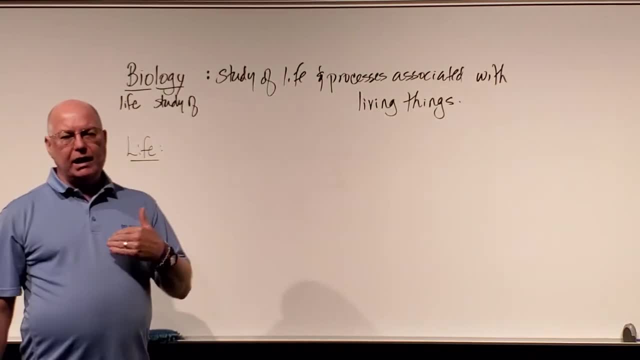 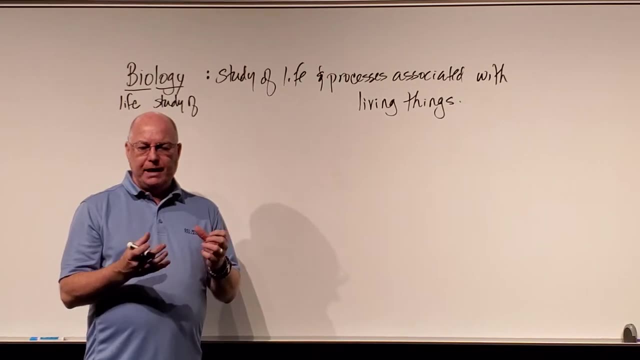 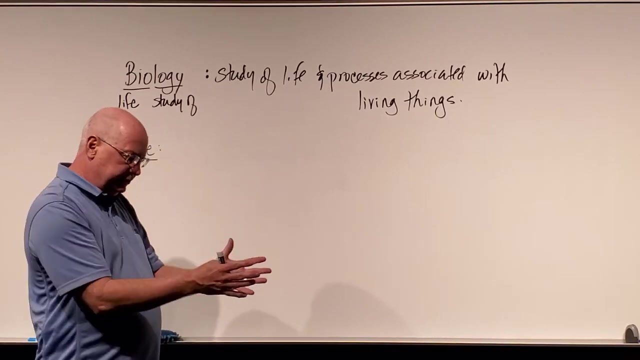 does that mean? So? one of the ways I like to think of defining life is: life is a collection of these characteristics or traits that allow us to determine whether something exhibits these characteristics and traits must be alive and something that is lacking one or more of these. 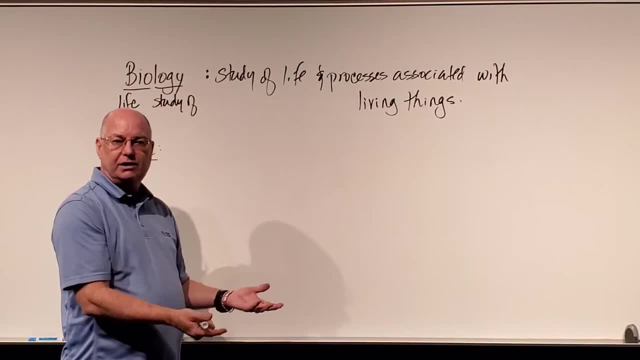 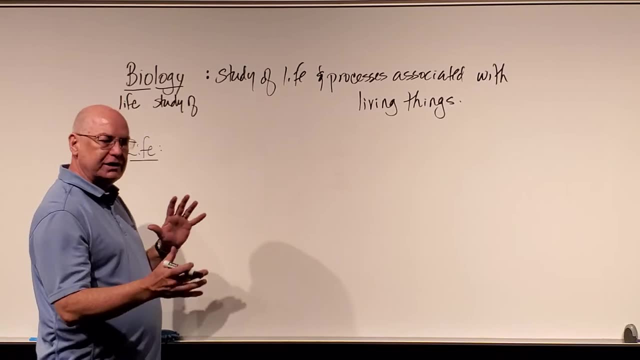 characteristics or traits cannot be defined as a living thing or as life. So I'm going to list those characteristics that you should understand. Now, different books have a different set and different number, but they all mostly cover the same ones. So if we're going 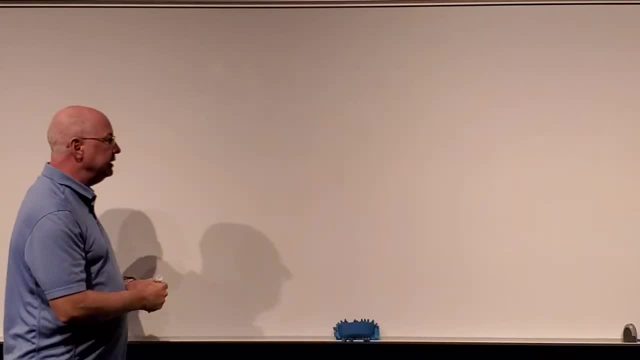 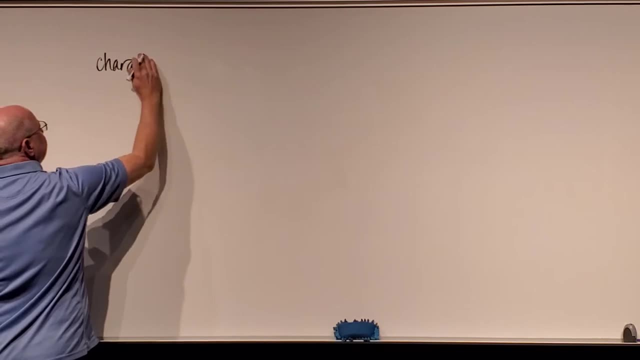 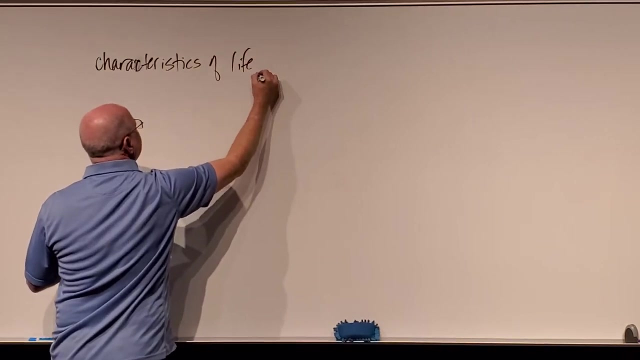 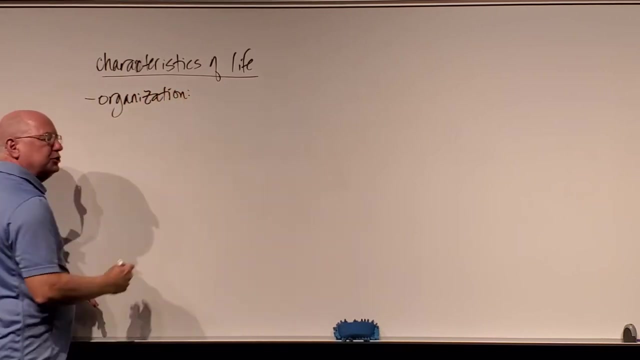 to just decide that something is alive or a living thing, it must exhibit these characteristics. Okay, so I'm going to just write this out as the characteristics of living things or of life. One of them is organization. It's not just random chaos like some parts of the universe, like if you looked inside the sun. 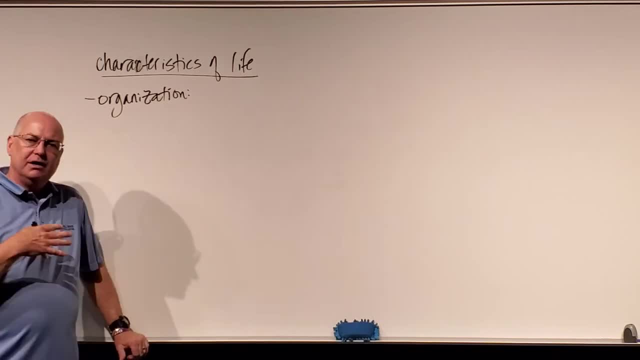 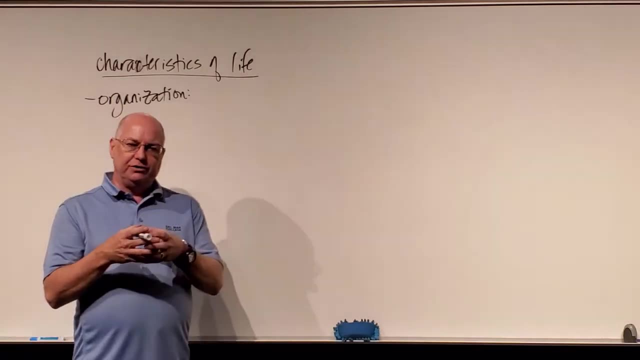 all the randomness of the universe. It's not just random chaos like some parts of the universe. It's not just random chemical reactions and nuclear reactions going on. It's not that. It's a very organized situation. So living things are comprised of cells and we know that all living 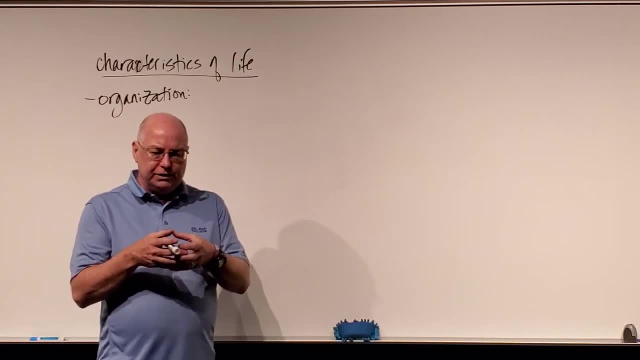 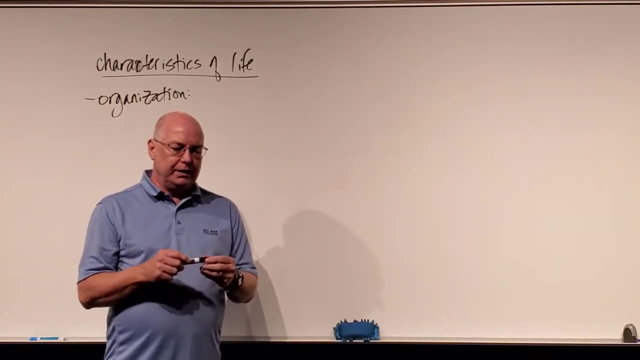 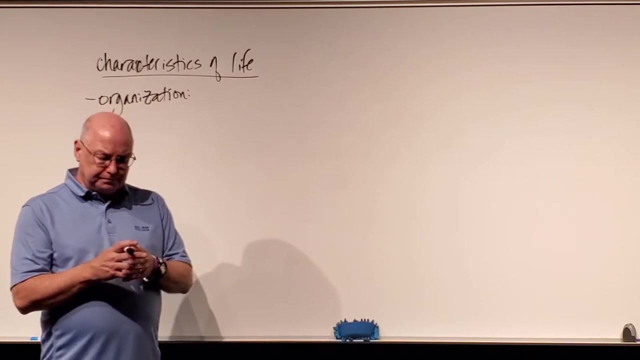 things are comprised of cells, and cells are the smallest living subunits of an organism, and some organisms are so simple that they're a single cell. Now, when we look at cells, cells are made up of smaller units, And some of those units are called atoms, and you study a lot of atoms in chemistry. 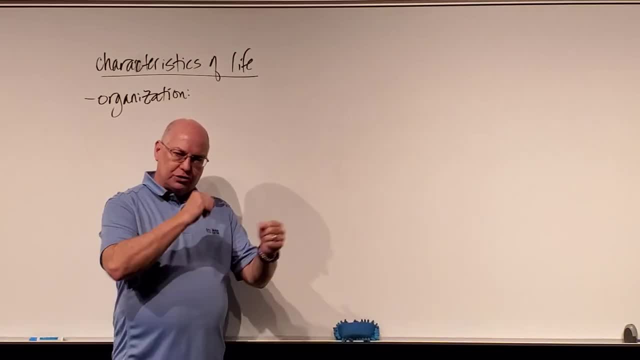 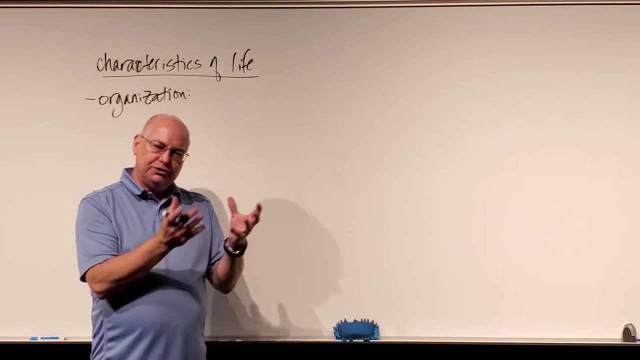 We're going to do a lot of chemistry in this class, And atoms are all behaving independently, but sometimes when a couple of atoms come together and interact, they form a molecule. So a molecule is just a collection of atoms that are exhibiting a unique and identifiable behavior. 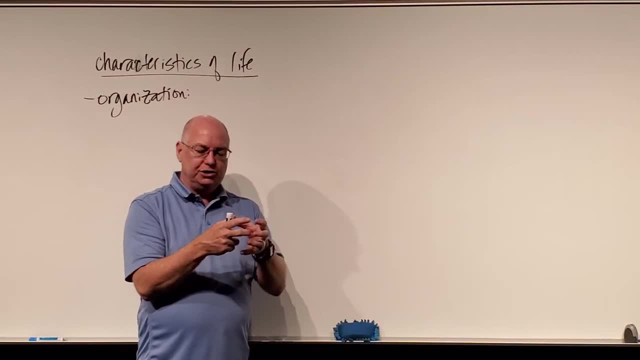 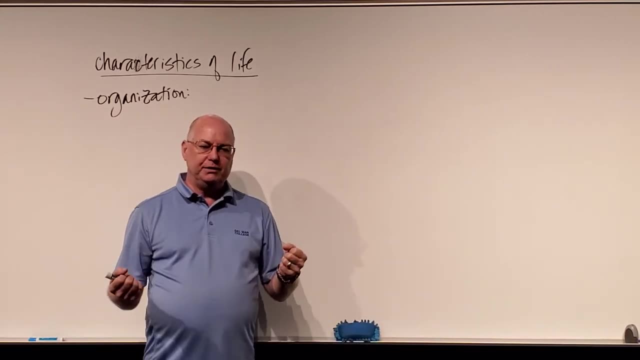 or performing what I- the way I define it is. they're performing a specific function. A bunch of different molecules behave differently, like water and methane gas and amino acid and lipid. But when we combine molecules together, sometimes they start working together to exhibit a definable or a defined behavior. 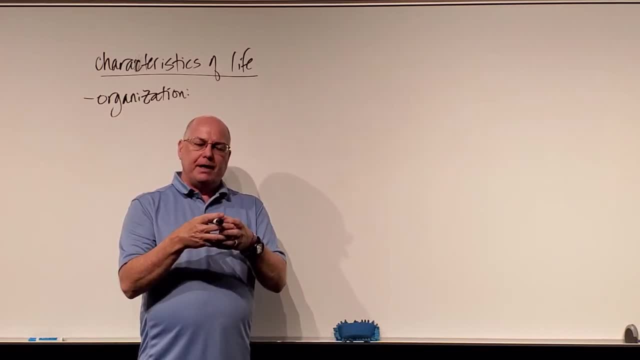 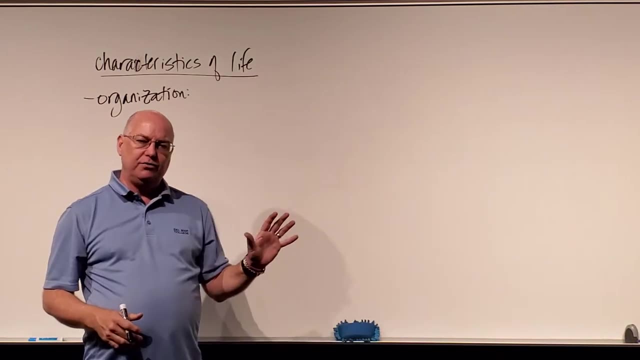 And we call those things organelles. And then organelles, each with their own behavior, can work together to form cells. Now, not all cells are made up of a lot of organelles, And we're going to learn that. 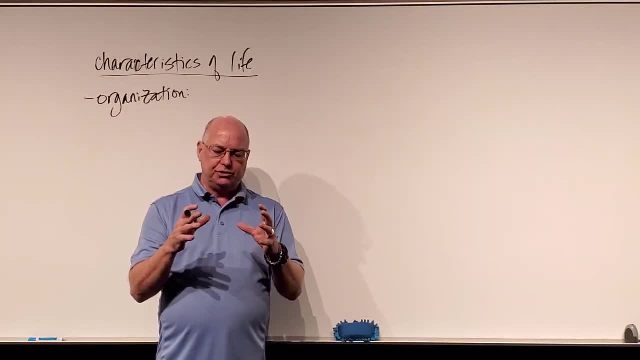 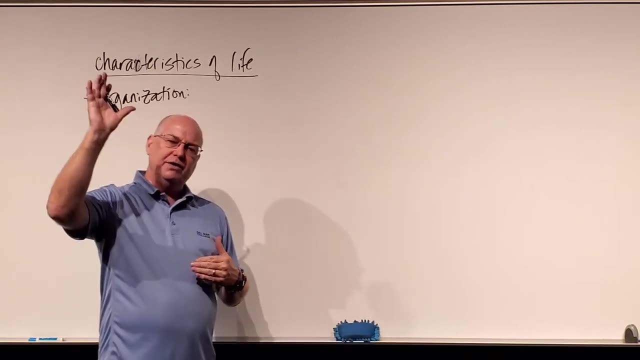 Especially in microbiology, And we're going to go over cell structure at some point. But then cells can come together to form tissues and then organs and organ systems and organisms And we go through all of that in anatomy and physiology and a lot of biology. 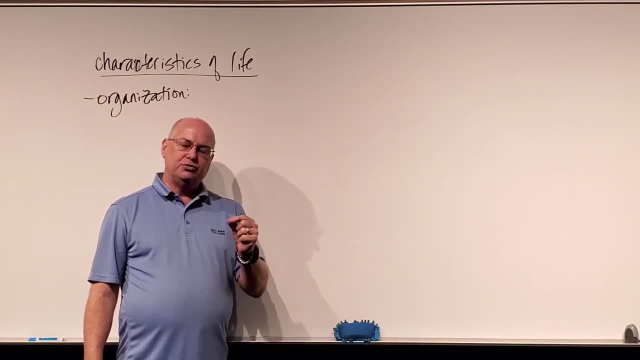 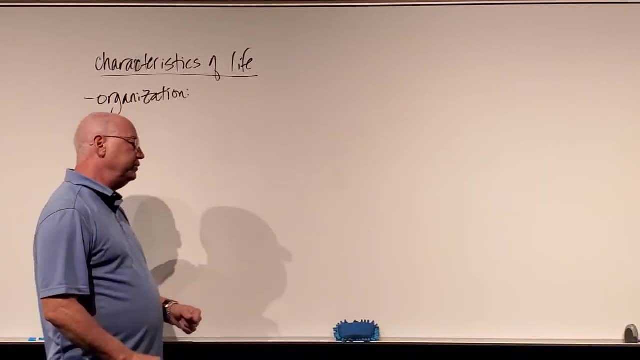 But when it comes to microbiology, sometimes the organisms we're looking at are a single tiny cell, Which helps us define what microbiology is, which we will do in just a moment. Another characteristic of life is that living things will exhibit what we call homeostasis. 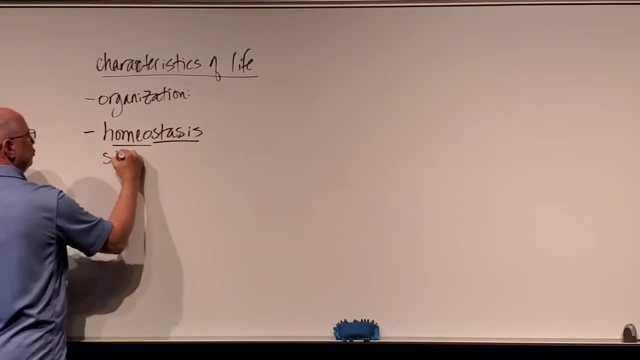 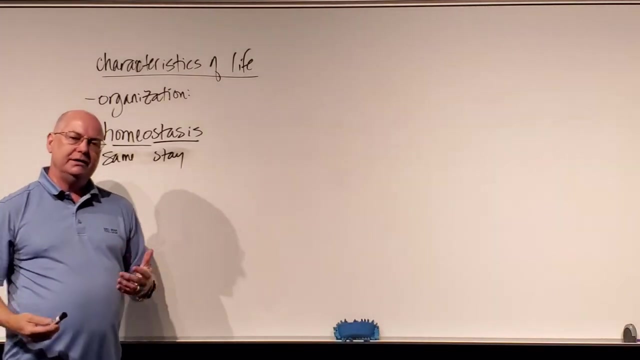 And if we look at homeostasis, it means to stay the same. Stasis means static or to stay, And homeo means same. I did that backwards, But this is same and this is to stay Okay. So the old idea is: if it ain't broke, don't fix it. 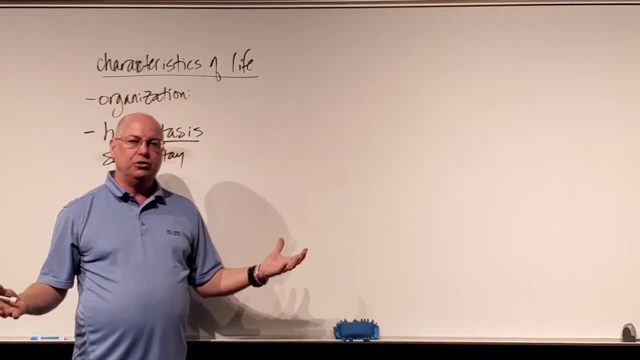 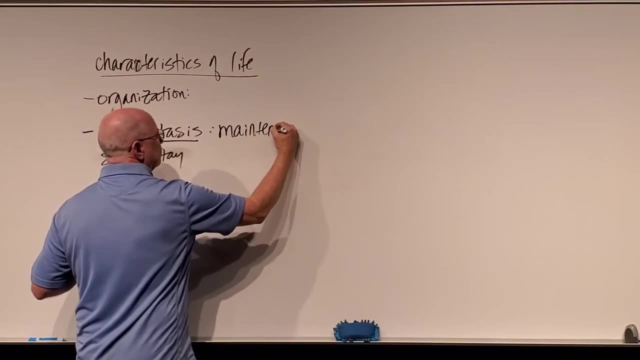 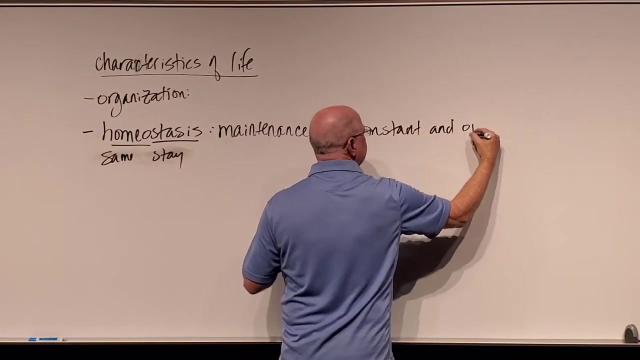 If your body is humming along, functioning perfectly, why would you alter what's working? So the technical definition of homeostasis is the maintenance. So the technical definition of homeostasis is the maintenance, The maintenance of a constant and optimal internal environment. 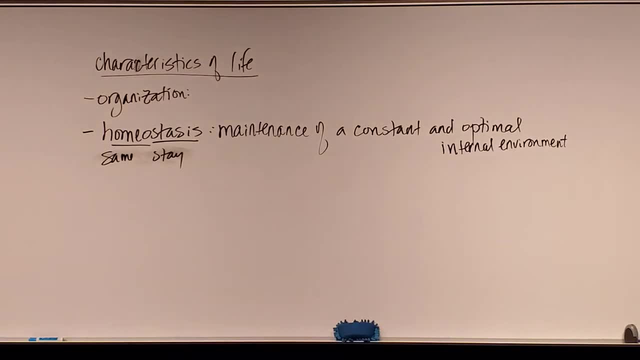 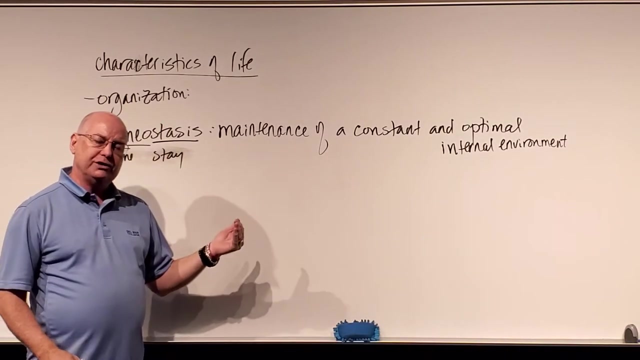 The maintenance of a constant and optimal internal environment. That's homeostasis. That's a definition that you should know, because it is the central foundation of all of healthcare. If our bodies are functioning perfectly, we need no intervention. If we're not in homeostasis, we're in what is called pathology. 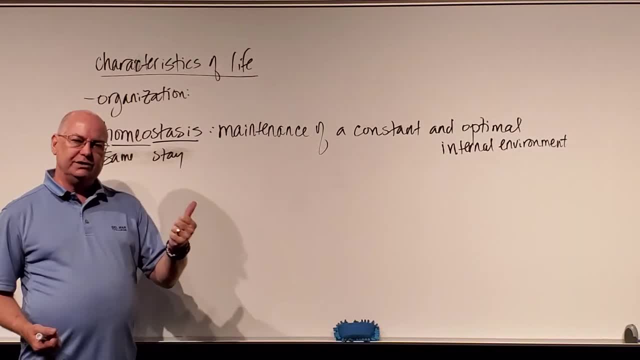 And in pathology, that is the study of disease or death and the processes that lead to that. As a matter of fact, we'll define pathology later on. But if your body is in homeostasis, you're not in pathology, and vice versa. 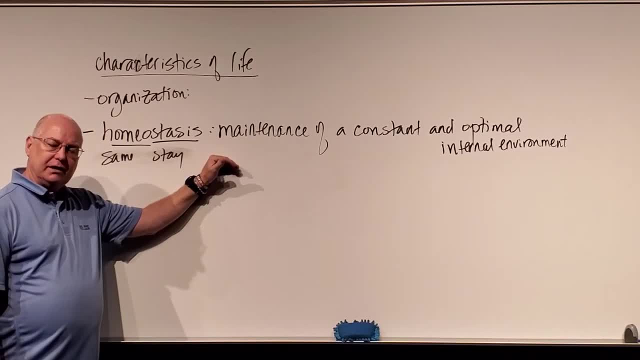 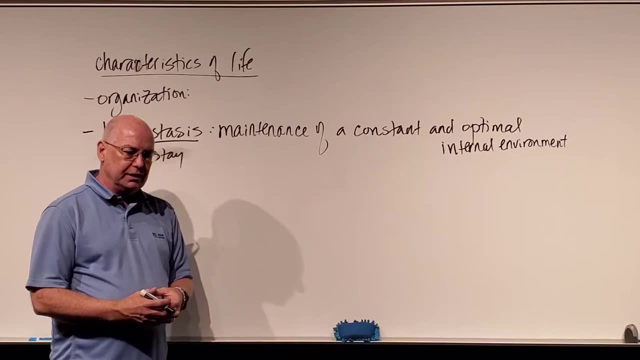 If you're in pathology, you're not maintaining that constant environment. Our body has feedback mechanisms. Our body has feedback mechanisms to control that, as do many of these microbiological organisms. But when that fails, sometimes we need to intervene with medicine. 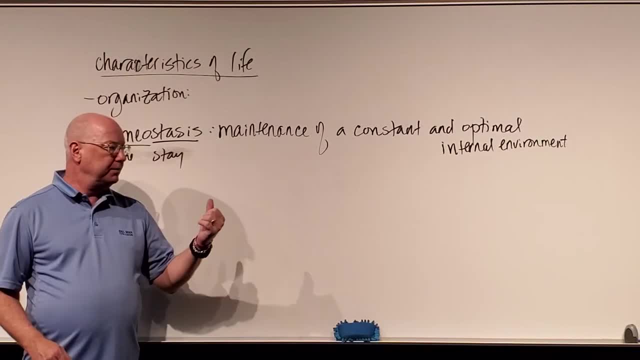 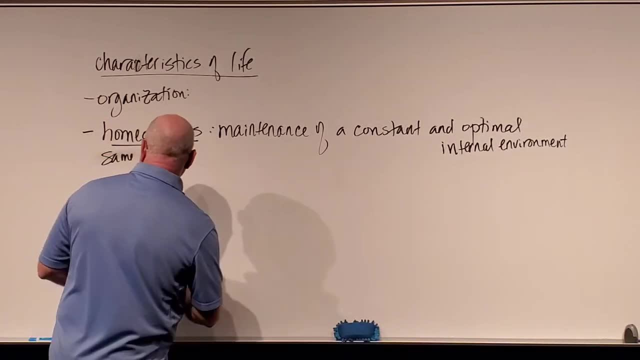 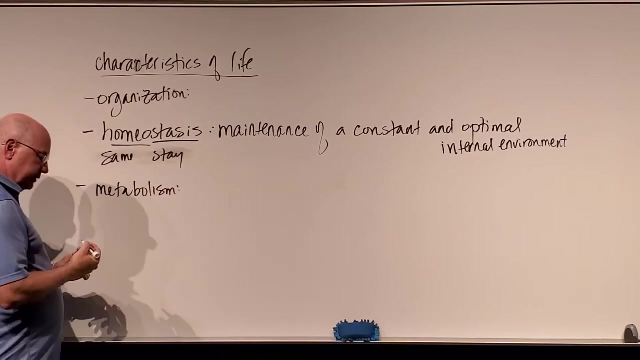 And a lot of the microbes we're going to be talking about result in pathology, And we'll see why and how when the time is appropriate. Now, another characteristic that all living beings exhibit is what we call metabolism. Now, technically, the definition of metabolism is the source of the body's energy. 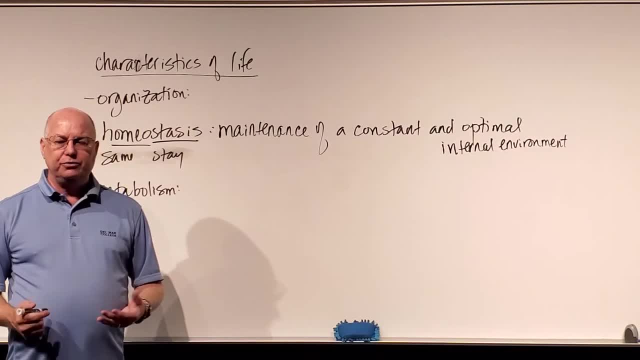 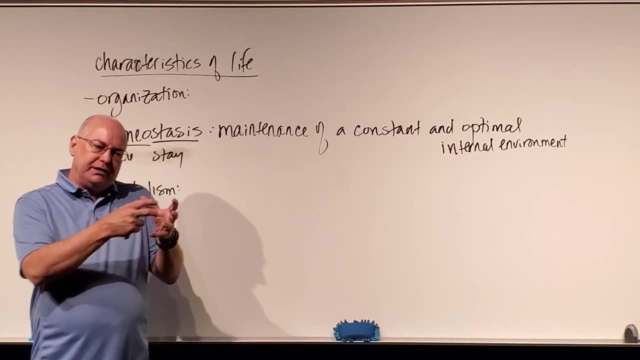 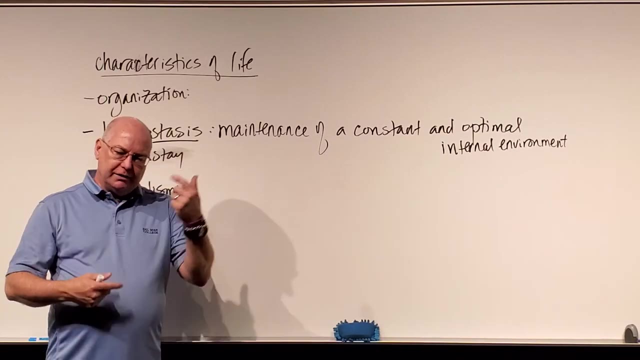 Metabolism is the sum total of all biochemical reactions in the human body, But in a general sense, metabolism is the ability to break down large molecules into smaller ones, or assemble small molecules into larger ones and convert some of those compounds into energy. 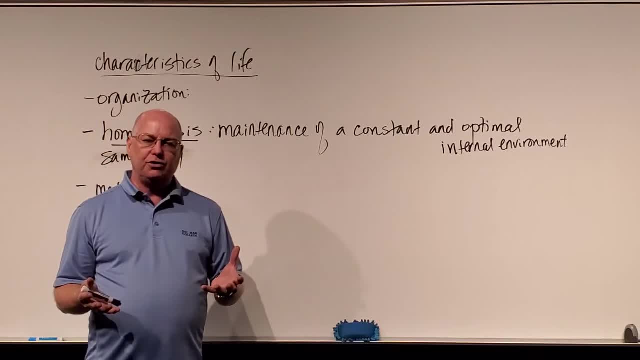 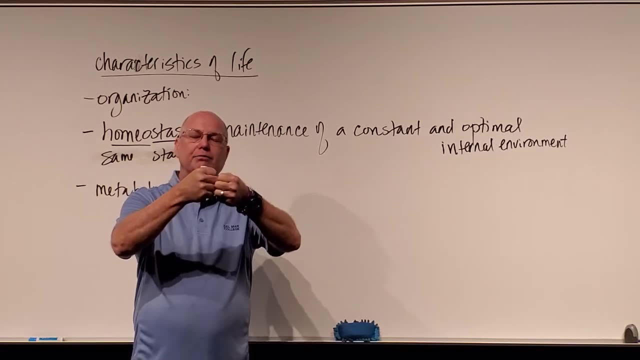 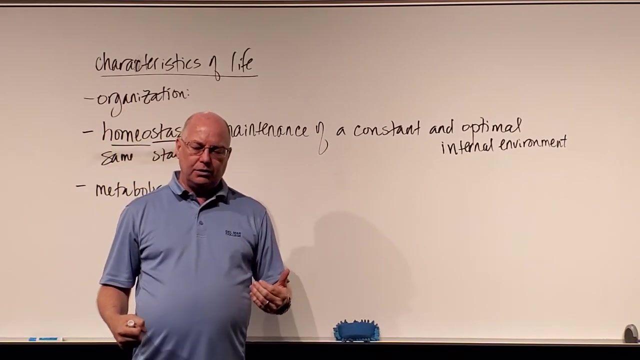 So metabolism is sort of all the chemical processes that are occurring in our body. If you eat a protein, your protein breaks down. Your body breaks that protein down into individual amino acids. So that would be catabolizing or breaking down a large molecule. 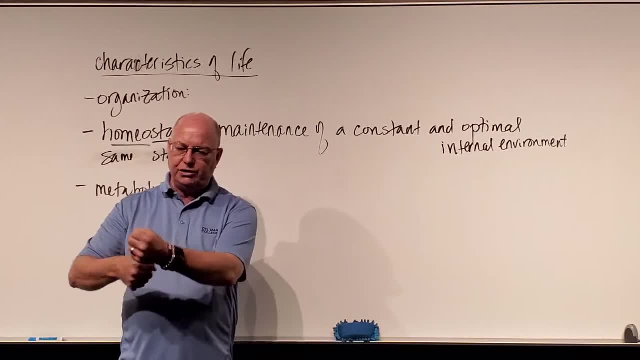 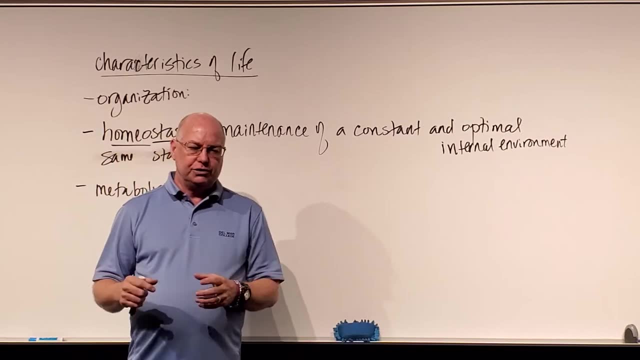 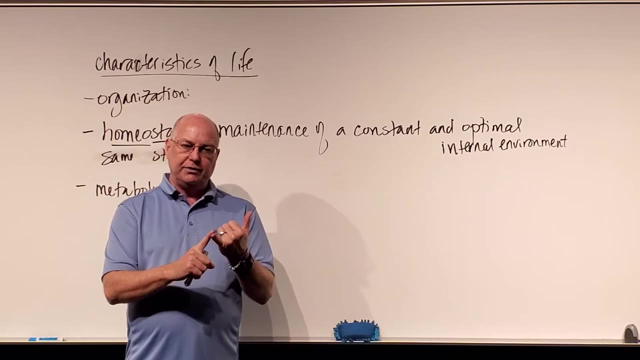 And then we take those amino acids, we send them to our cells and we reassemble them into human protein. So we would be taking small molecules and building them into larger molecules, assembling them together. We call those anabolic reactions. Now in the world of chemistry we also refer to what we call degradation or synthesis reactions. 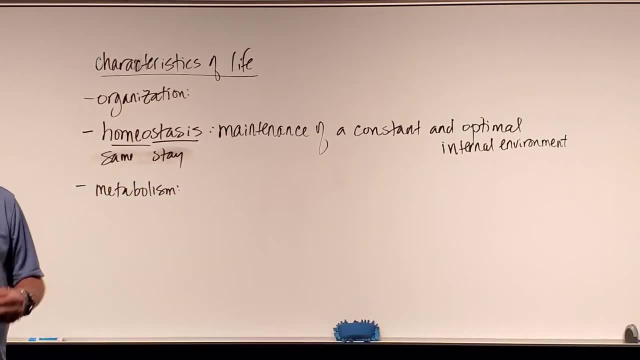 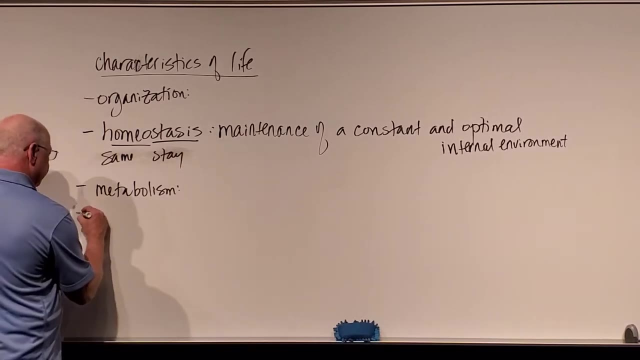 And we'll get into all that chemistry eventually. But metabolism, the ability to break things down and reassemble them and produce energy, is a really important part of, or one of the important characteristics of all living organisms. Now, another characteristic that is exhibited by living organisms is growth. 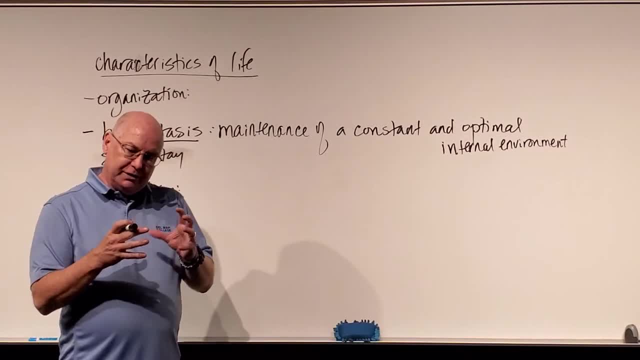 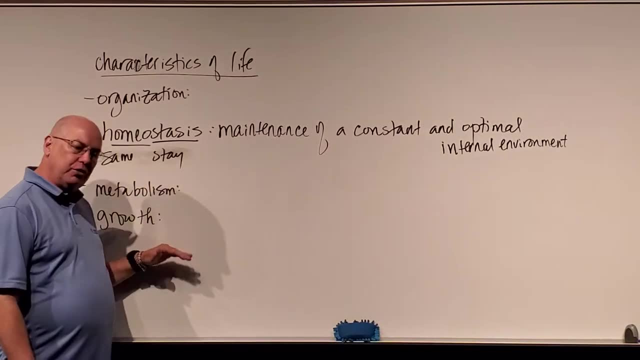 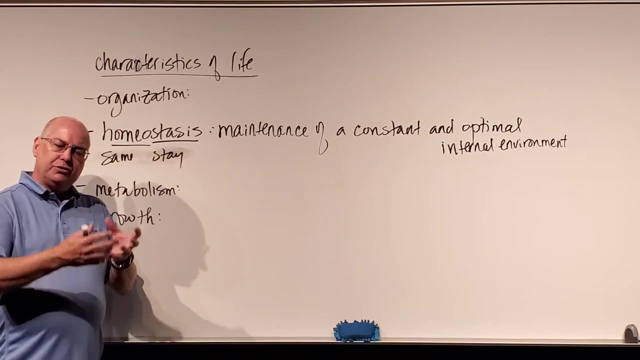 Growth, as an individual to become bigger in size, or sometimes as an organism, to increase the number of cells. And so we're going to look at microbial growth. We're going to look at how cells and some of these microbes will grow, how they can increase in size through their metabolism. 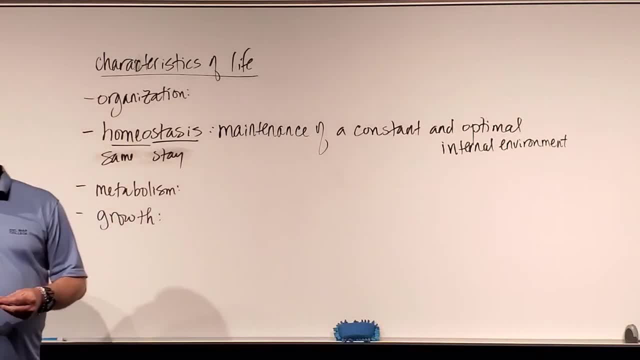 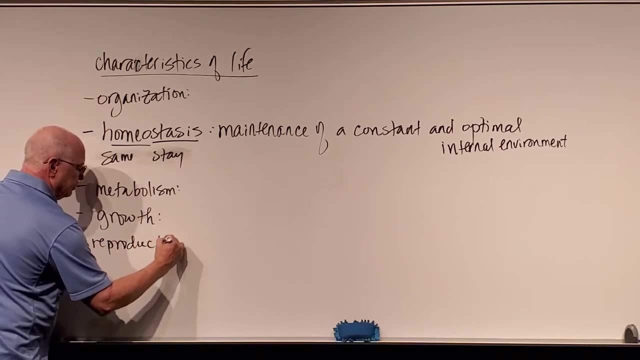 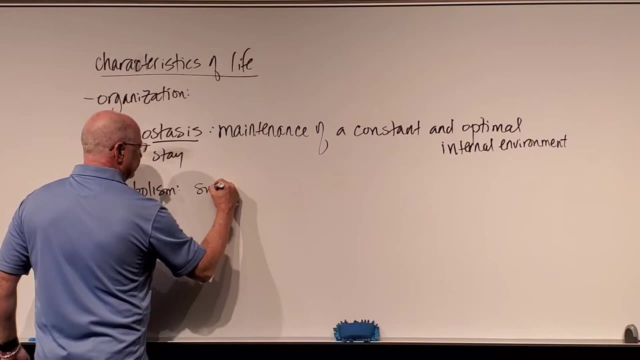 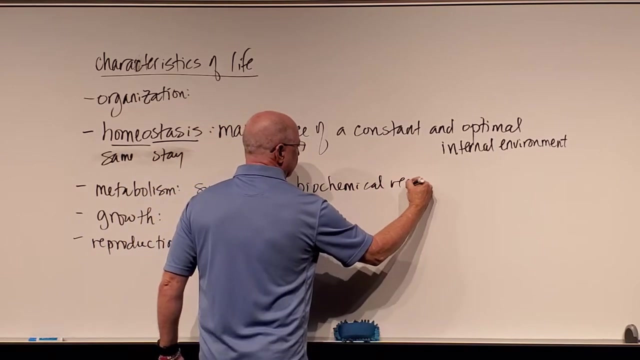 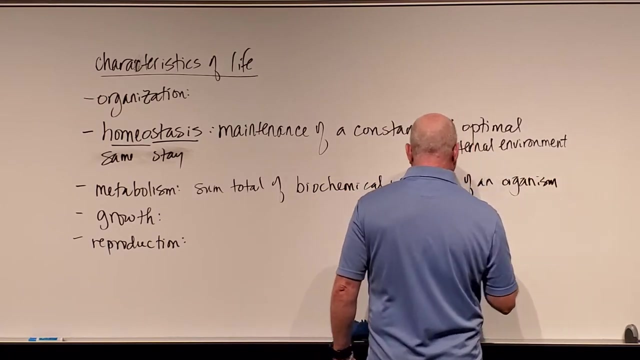 and how they can also grow in number of cells, And that's another one of the characteristics of a living organism is reproduction, The ability to reproduce or make more of yourself. Okay, So metabolism we'll define as the sum, total. Sum total of all biochemical reactions in the body or of an organism. 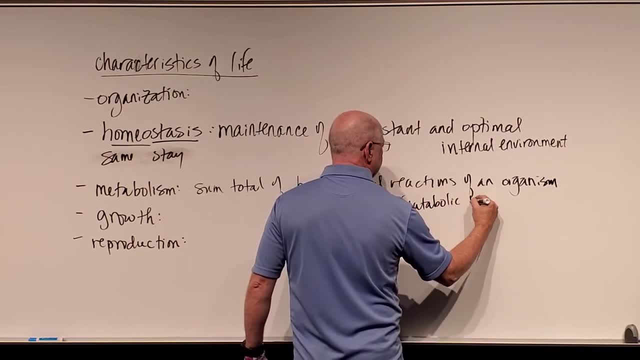 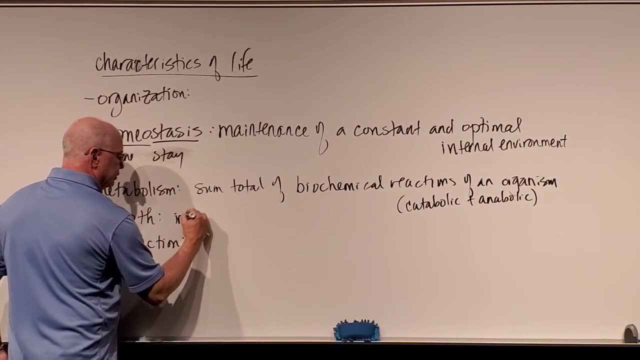 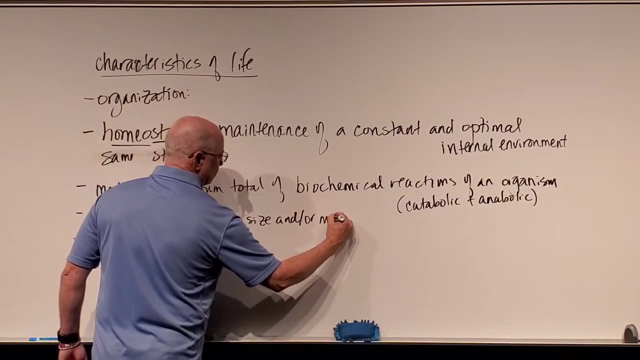 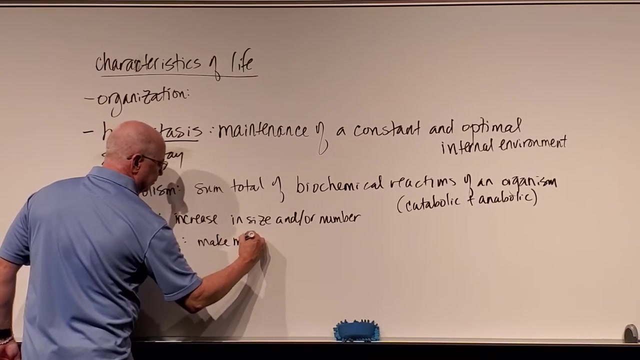 And that would be what we call catabolic plus anabolic reactions. We're going to define those one day. Growth is to increase in size and or number, And reproduction is to make more of yourself. Now, these are, Mr Long, general definitions, but they work. 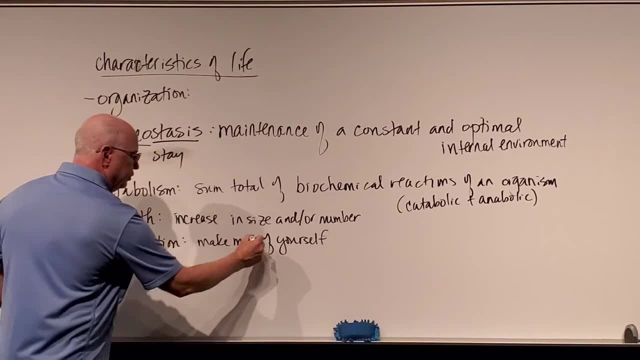 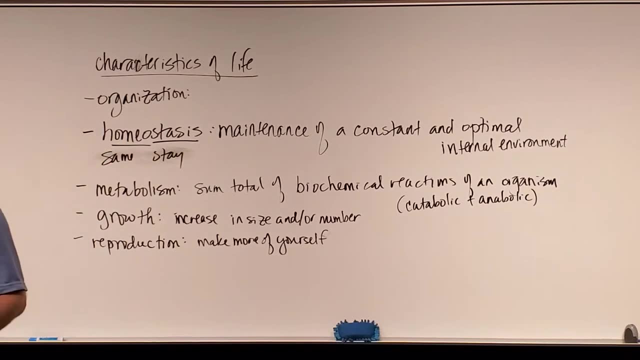 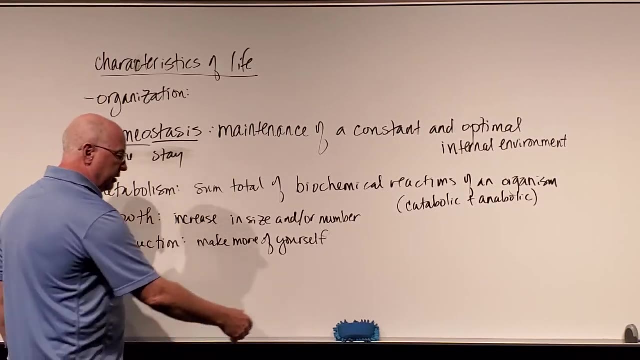 And so we're going to look at how organisms can sometimes reproduce and grow and metabolize and maintain their homeostasis. Now a couple of more of these characteristics. I'm running out of room at the bottom of the board, so I'm just going to go back up to the top. erase some of these. 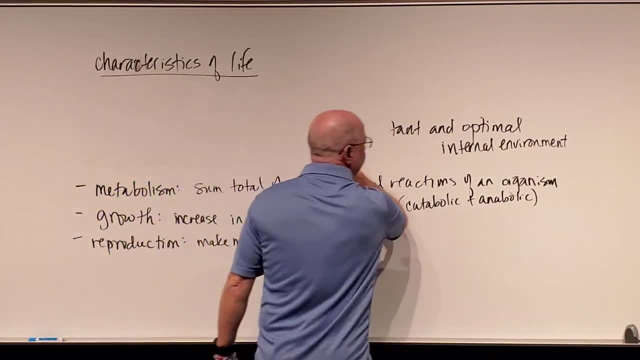 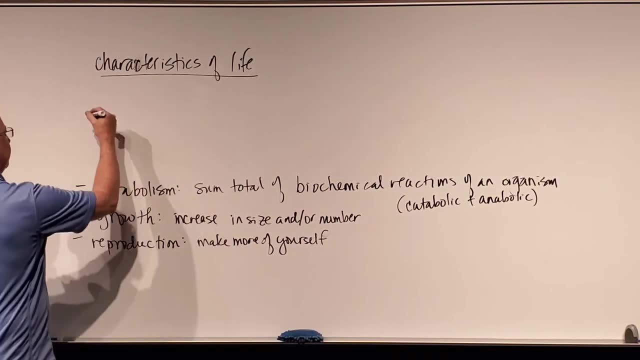 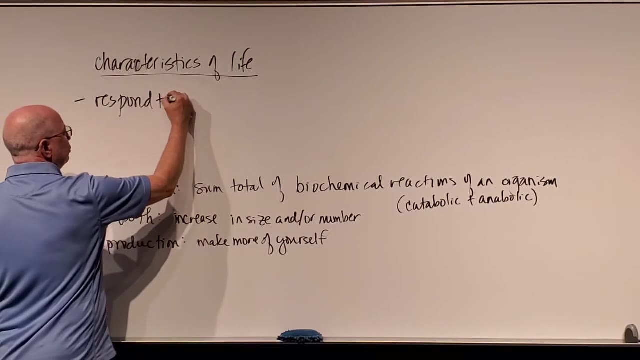 and add the last two that I want you to know. Now, some books have a few more than this. Break some of these out into other categories or combine some of these into a category, But nonetheless respond, And really we should say respond- to the environment. 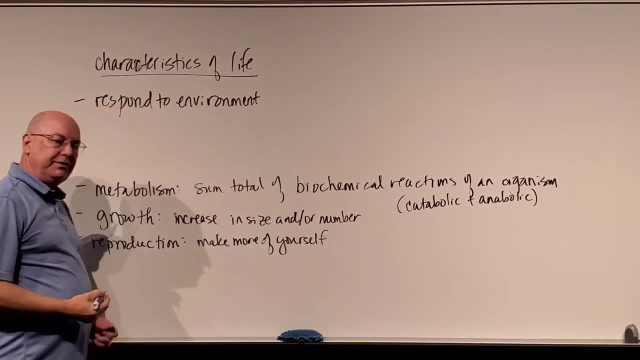 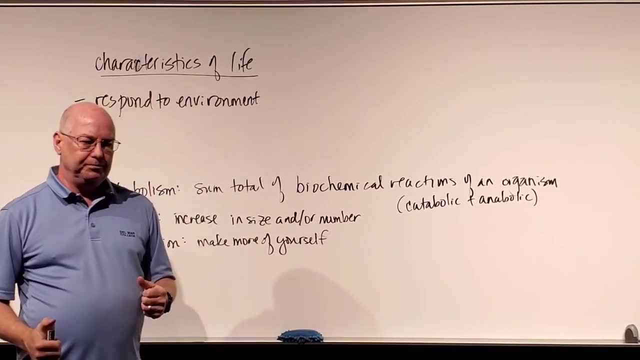 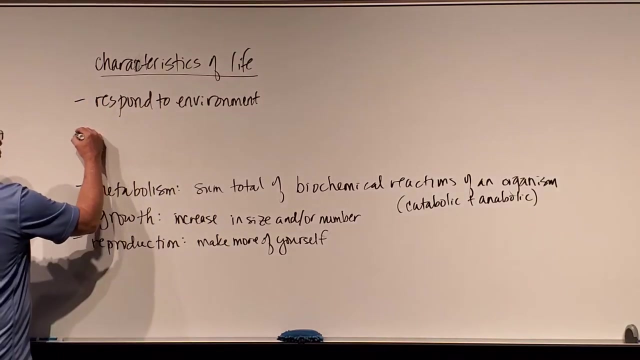 Okay. Living things can sense what's going on in the surrounding environment and then respond to those changes in the environment that allow them to continue to survive, And so that is one of the characteristics of all living things And similar to respond to the environment is to adapt. 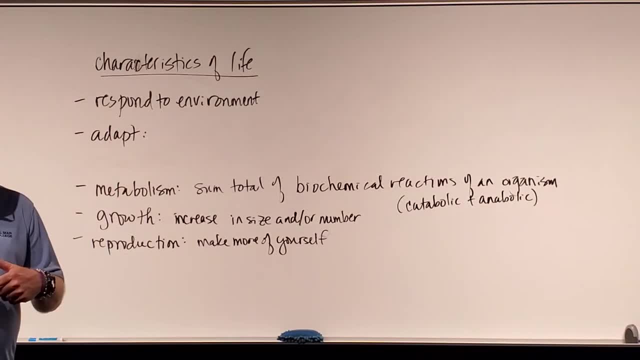 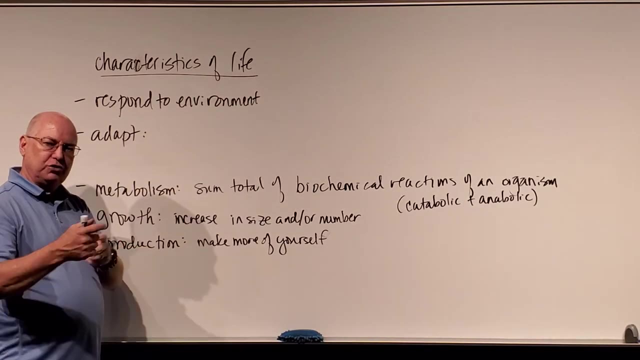 Now, to adapt means to change sort of in a long-term way over time to survive changes in your environment. So when we talk about respond to the environment or respond to changes in the environment, what we're talking about is sort of short-term things. 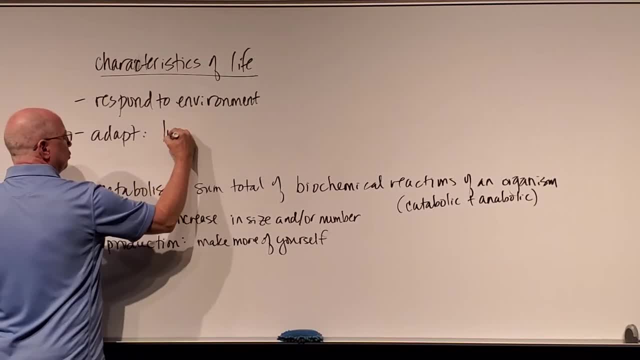 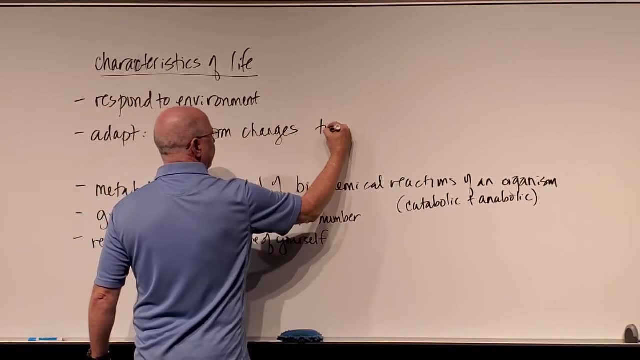 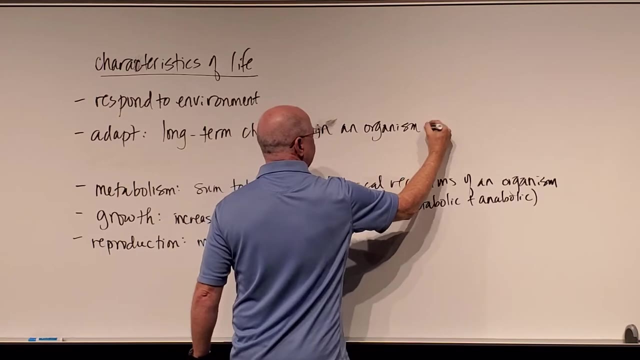 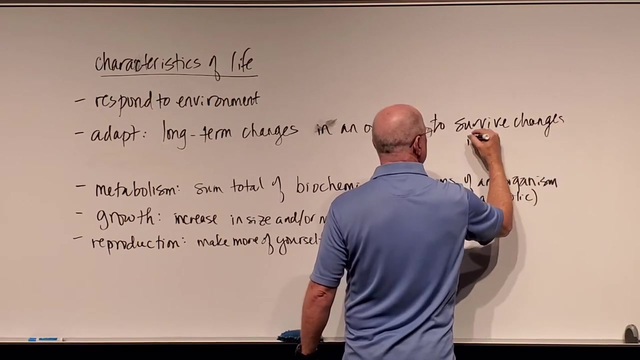 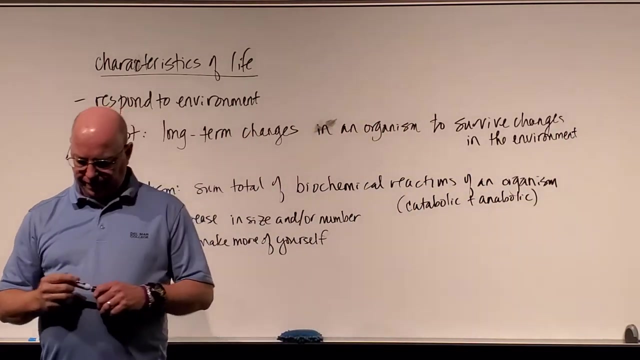 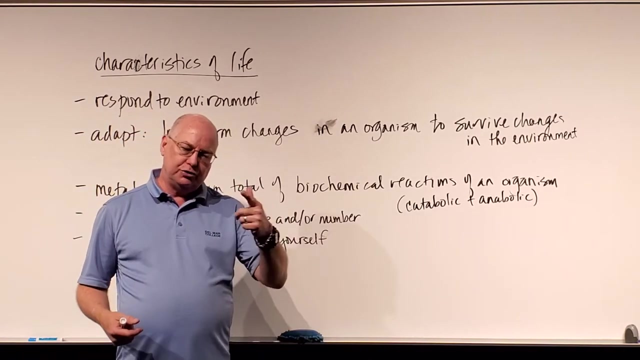 When I talk about adapt, we're talking about long-term changes in an organism to survive changes in the environment. So, for example, if there's a particular organism that has the ability for what we call motility, or to move, and it bumps into some predator, something that could kill it, 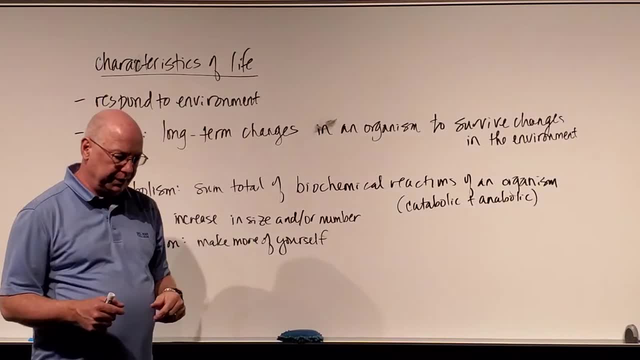 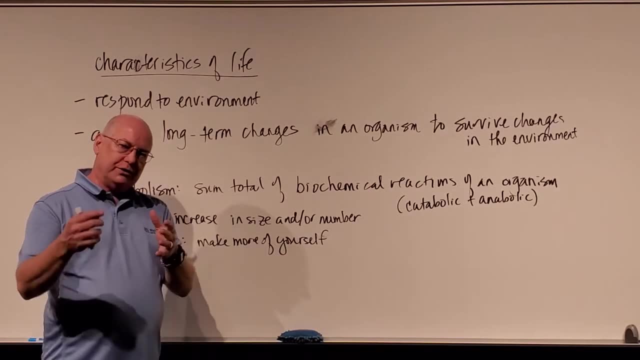 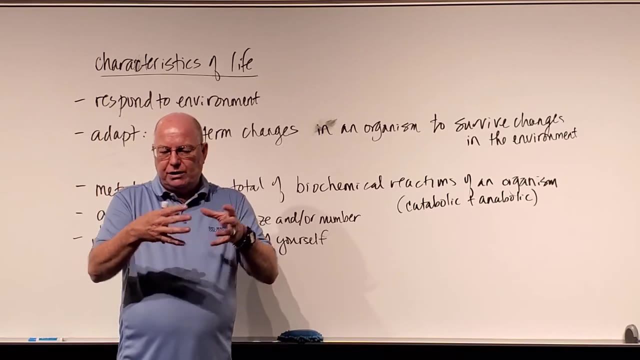 it can respond by swimming away or moving away from that organism. That's not adaptation, That's response to a change. Or if there's a different, if there's a chemical change in the environment, then maybe the organism will change its metabolism so that it can grow and develop. 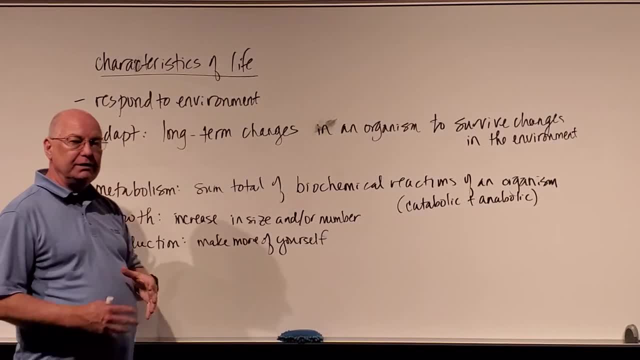 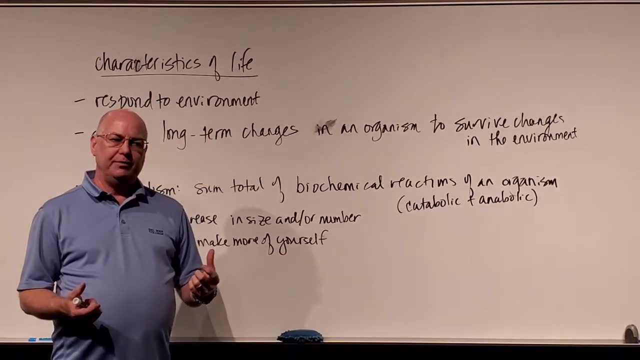 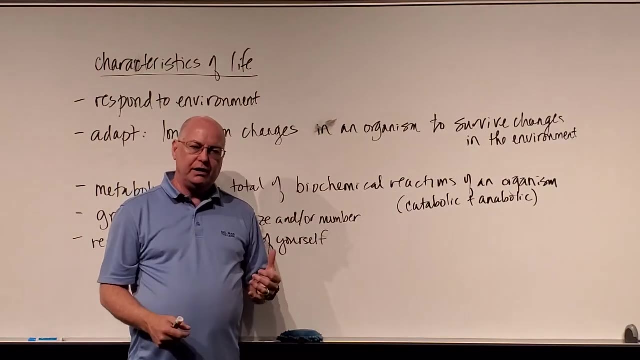 That's an immediate response. To adapt means to alter the organism's functions over the long-term to bigger changes in the environment. For example, if I were to take some bacterium that lacks a particular temperature and grows at a certain rate at a specific temperature. and over time the temperatures in that region start changing. maybe some of those bacteria will develop a new metabolic pathway to deal with the changes, the slowing of metabolism, as the area may cool so that they can survive, where many other organisms might be killed off by that change. 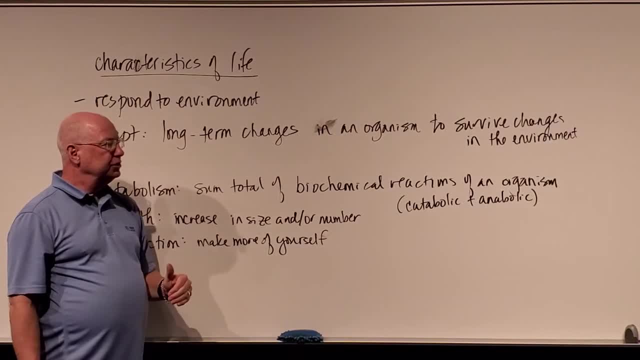 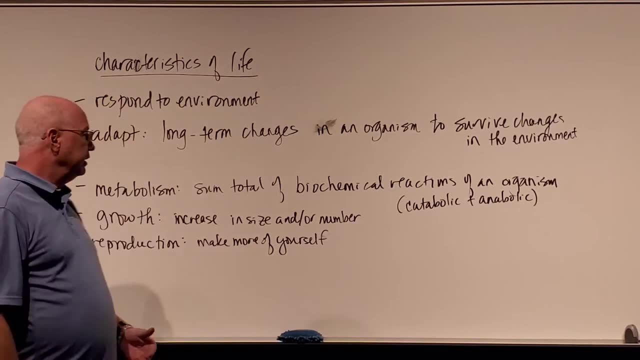 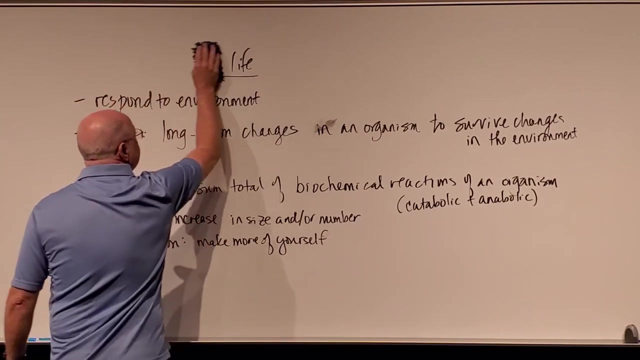 That's adaptation, Long-term changes in an organism that allow them to survive changes in the environment. So these are some of the major characteristics of a living organism and you should be able to list them and know them. Now this leads us to some other things. 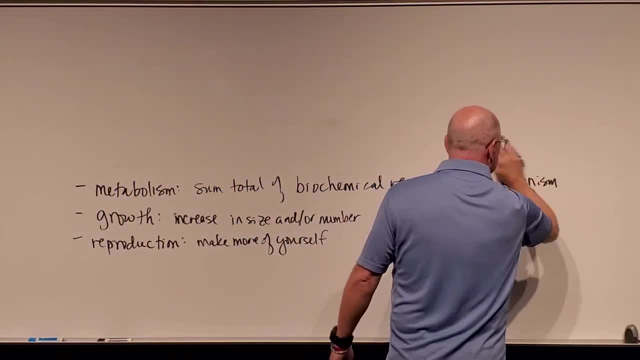 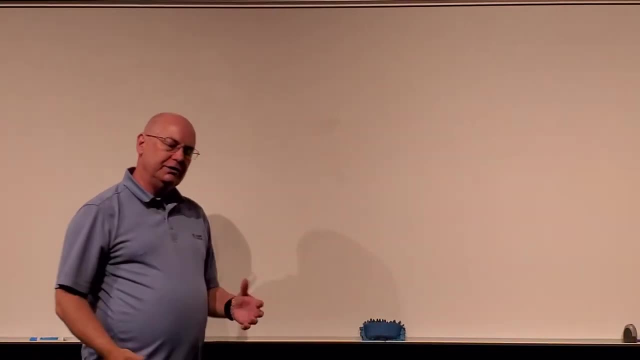 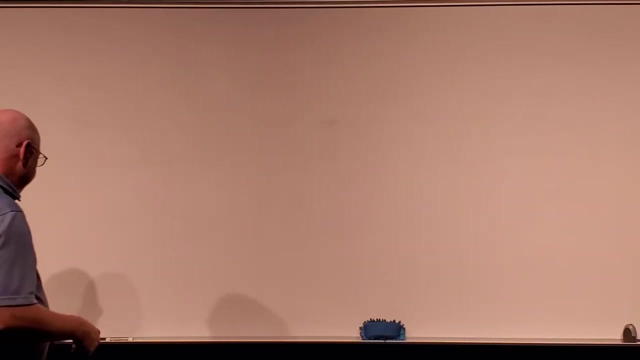 We're talking about biology, the study of life and living organisms. We were able to define some of the characteristics that determine if something's alive and all living organisms exhibit some of these characteristics or some combination of them. But a few of the other terms that we need to discuss. 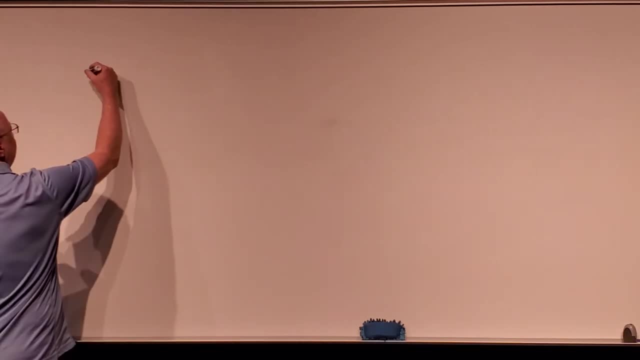 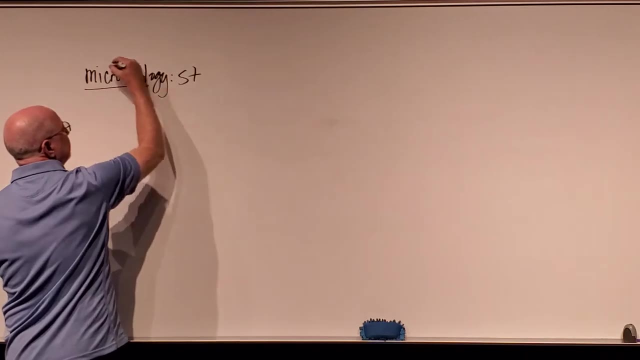 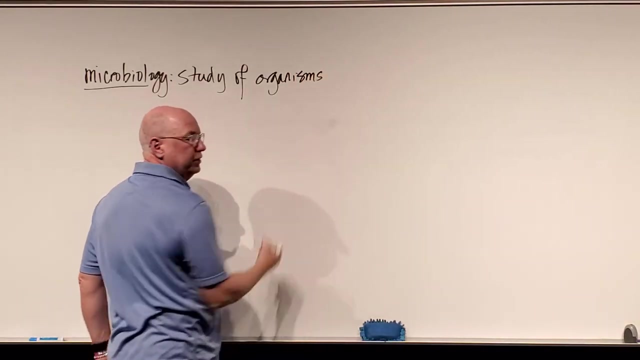 Now that we understand what life is and that we're studying life, what is microbiology? Well, microbiology is the study of organisms and, again, none of these definitions are perfect for every situation, because some of the stuff we're going to look at are not considered living organisms. 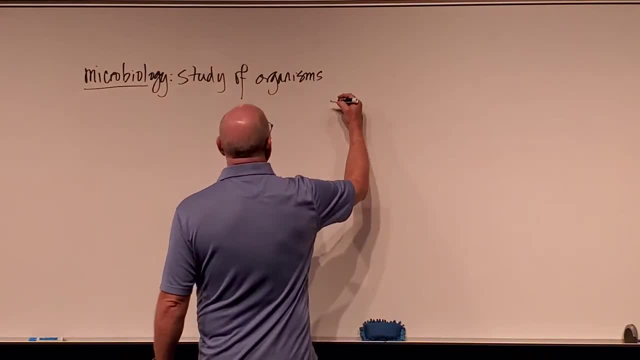 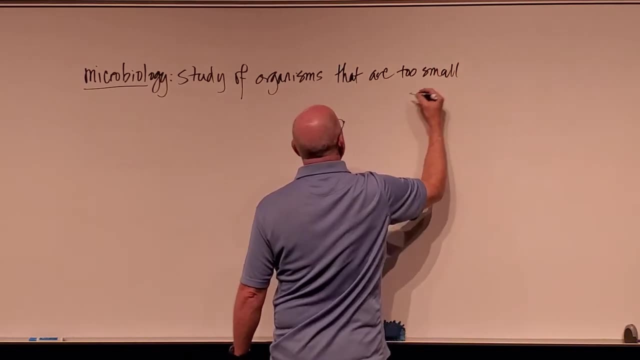 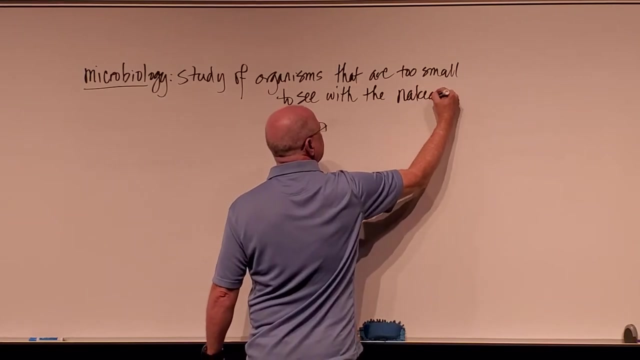 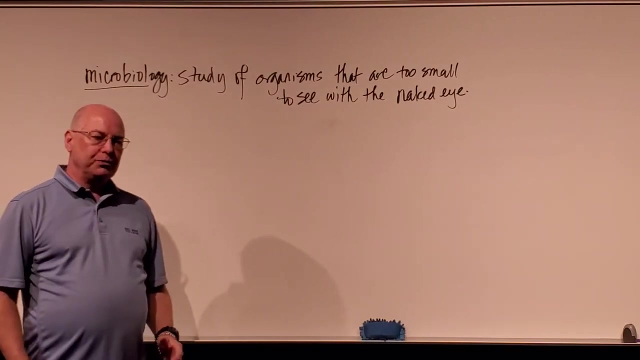 like viruses and primates, But nonetheless it's the study of organisms that are too small to see with the naked eye. These are tiny little creatures that we cannot see with just plain old vision. We have to use a specialized instrument called a microscope in order to see them. 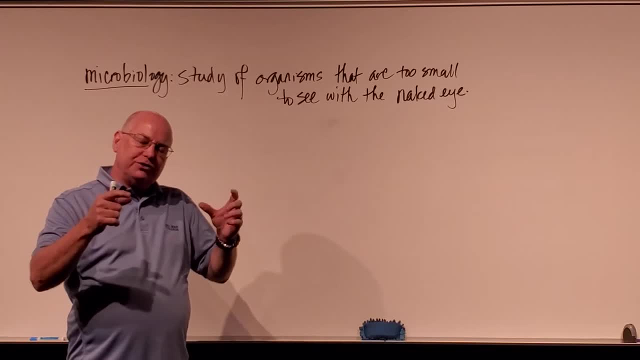 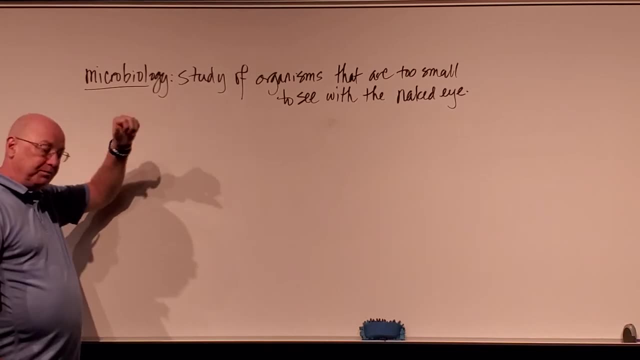 And the microscope is simply going to magnify something and resolve something so well that we can see it with our eyes, but we need a machine or a tool in order to see these organisms. Now, technically, that's not 100% accurate. 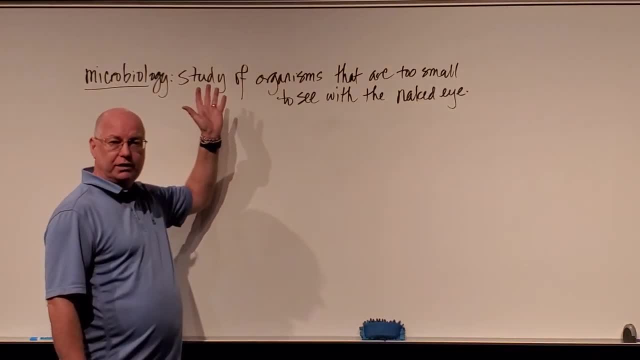 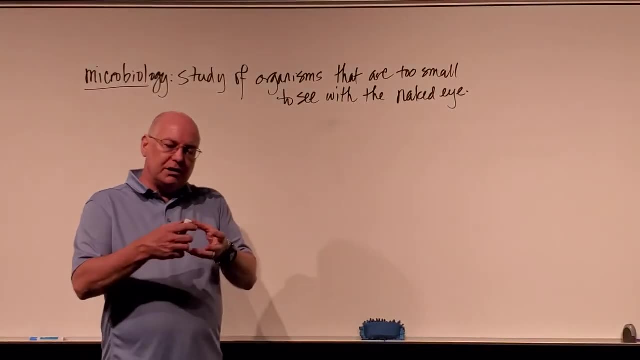 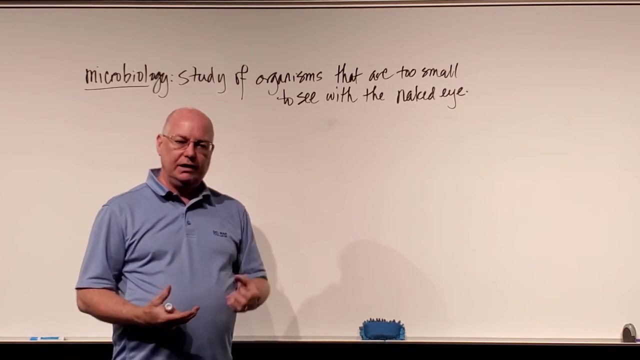 For number one, not everything I said a minute ago. not everything is a living organism, like viruses, And we're going to study them And also some of the things we can see with the naked eye, because sometimes these microbial organisms will grow in a manner and in number that they become visible to the naked eye. 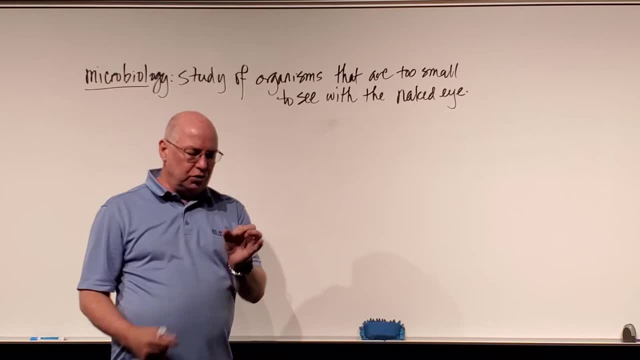 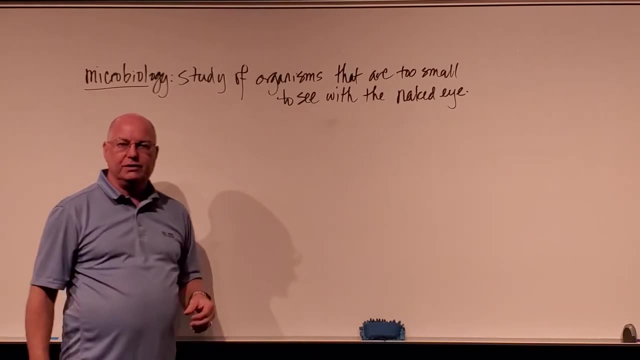 Like one bacterium that you may not see, but as it divides and grows and grows and grows. it'll show up as a little colony or a plaque on a petri dish and some of them grow and turn into fuzz, like the microbes that result in mold growing on your cheese at home. 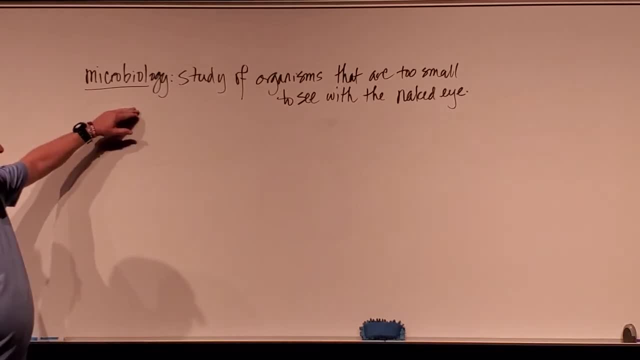 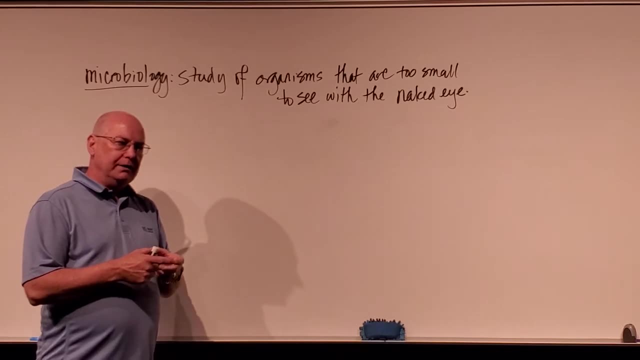 if it's been sitting in the fridge too long. So some of the organisms eventually we could see with the naked eye, And actually there's a few organisms that we can see with the naked eye, but we study them using other techniques in microbiology. 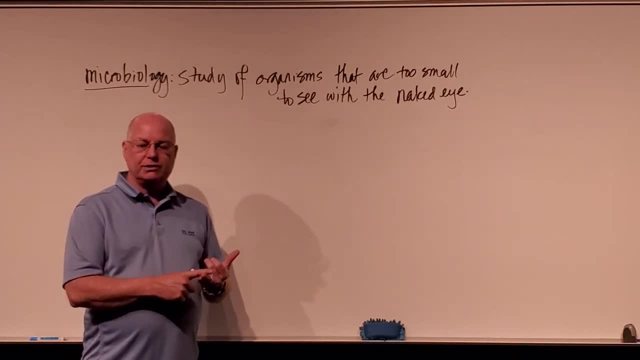 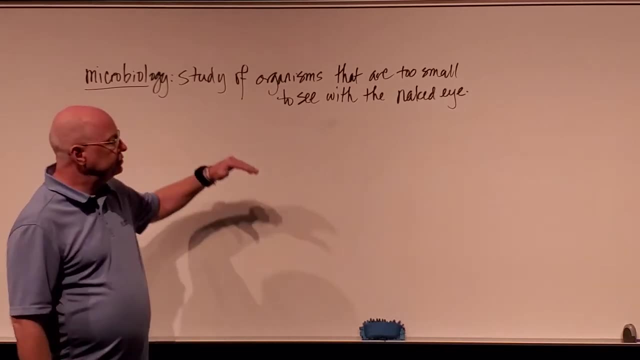 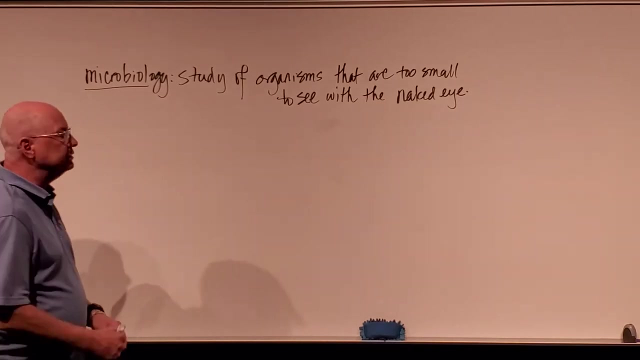 like staining and other types of microscopy or other biochemical techniques in order to see them and understand them. So, again, this is an imperfect definition, but ultimately, that's what microbiology is. It's the study of microbes, which are things that are too small to see with the naked eye. 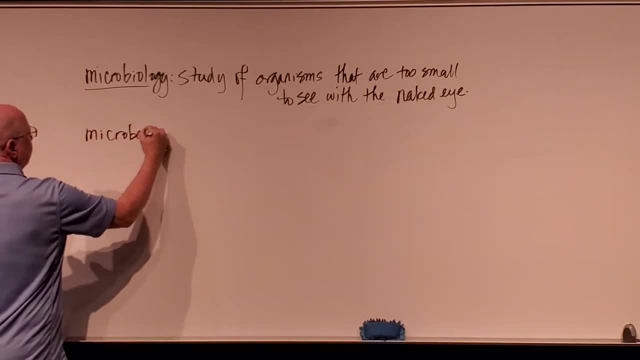 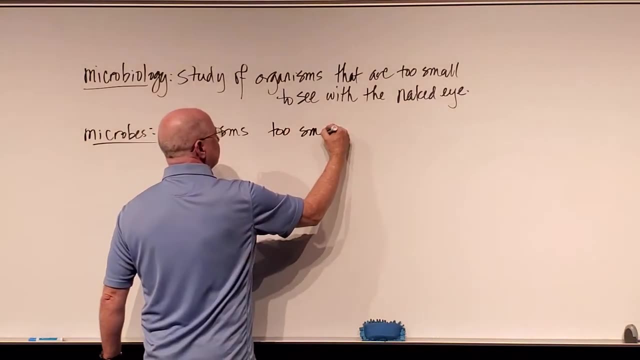 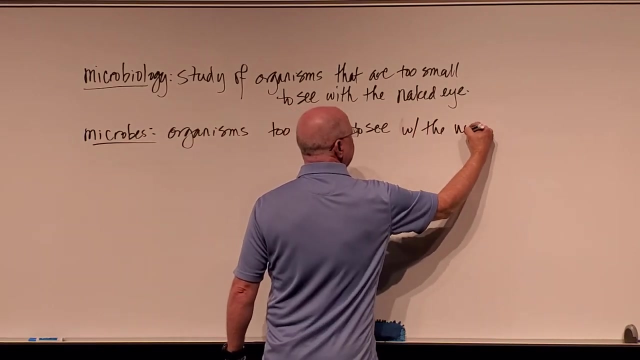 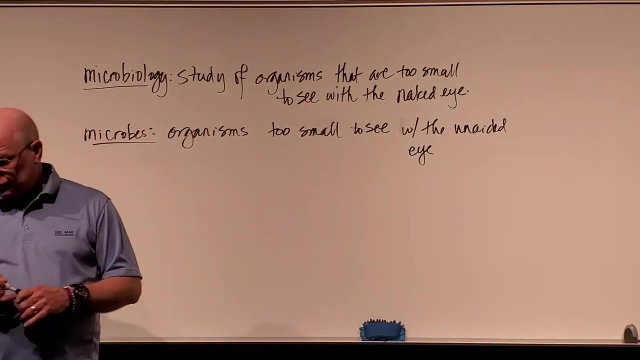 And that's another definition. you should know What is a microbe. Microbes are organisms too small to see with the unaided eye, And when I say naked eye we can say also unaided eye. It doesn't have the aid of a visual scope. 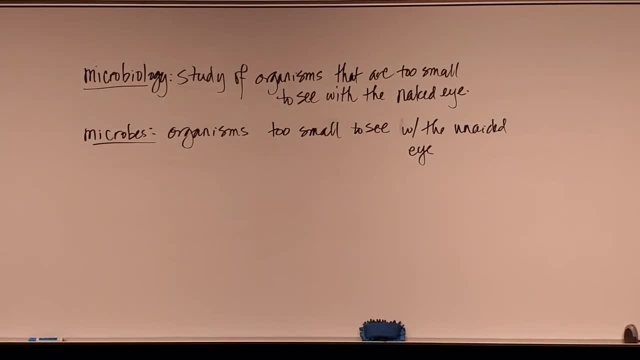 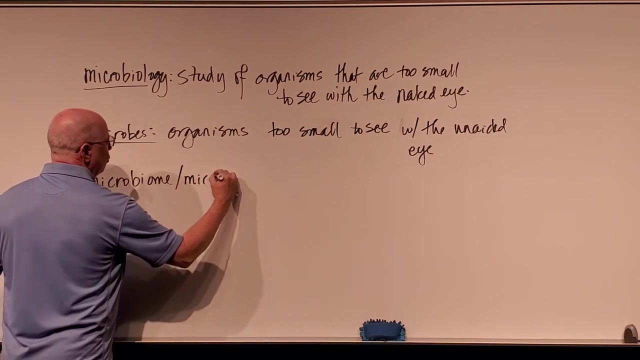 or a tool that allows us to see it. So it's a group of organisms that are too small to see with the naked eye, And one other term I need you to know is what we call the microbiome, also called the microbiota. 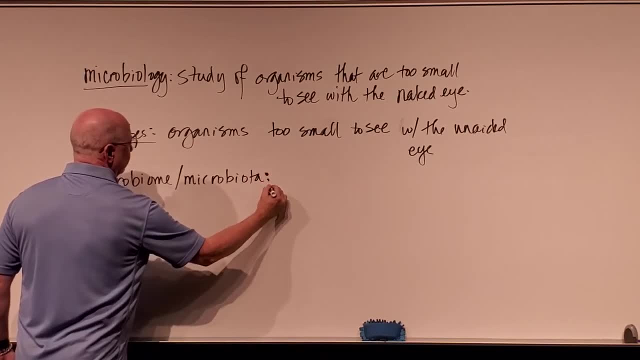 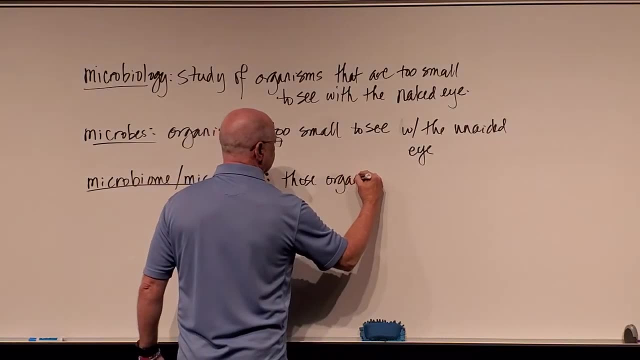 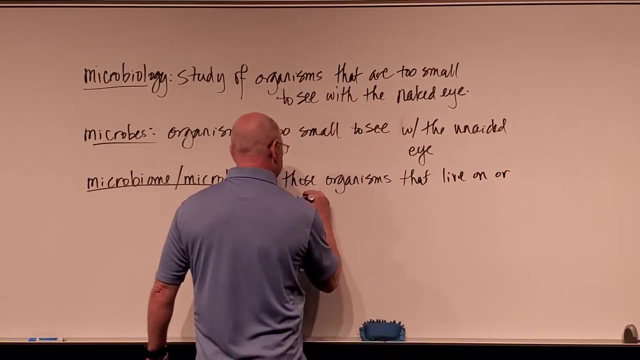 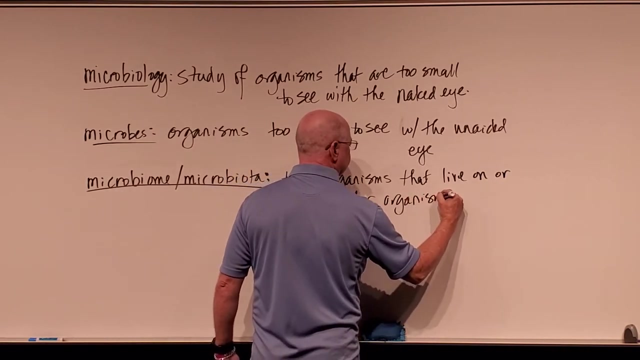 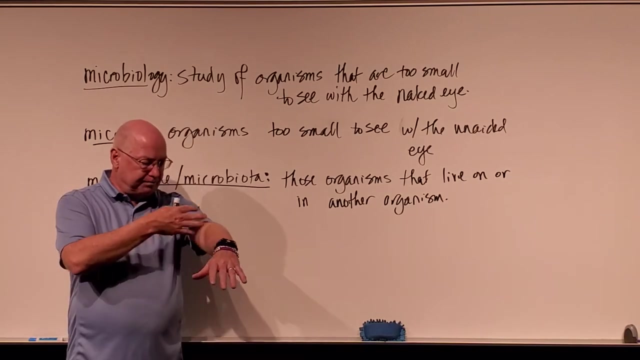 The microbiome or the microbiota are those organisms that live on or in another organism, Usually an animal, but not always. Sometimes in plants as well. So, for example, human beings have a microbiome, We have bacteria and things that grow on our skin. 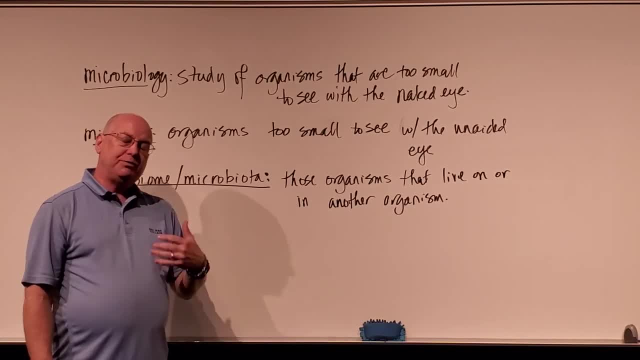 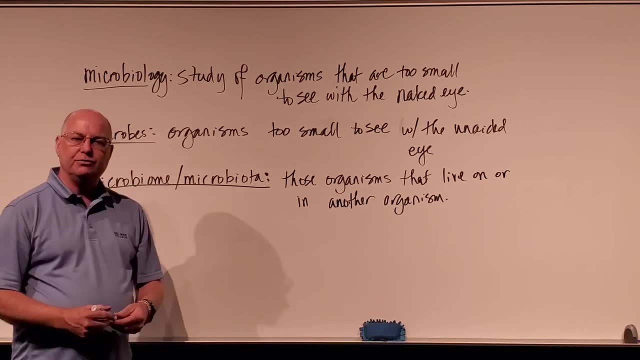 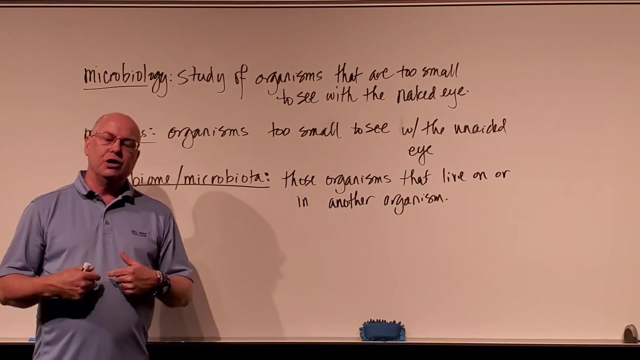 and in our gut. that actually provides a lot of benefit for us. They can prevent parasites and fungi and other things from growing on us, And some of the bacteria and the normal gut flora or the microbiome helps us break down some of the materials that we eat. 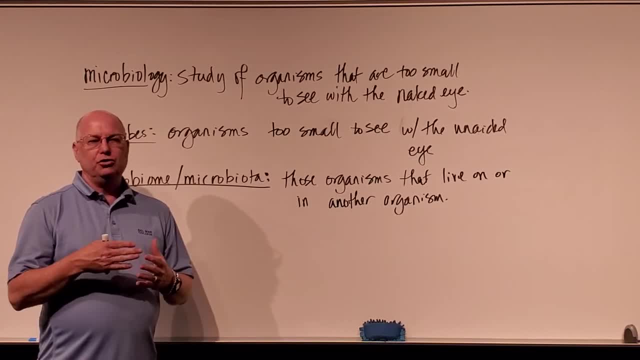 They produce vitamins that we absorb, And so same thing with cows. Some of them are what we call ruminants: Certain organisms have bacteria that live in their gut that allow them to break down things like grasses and other types of plants. 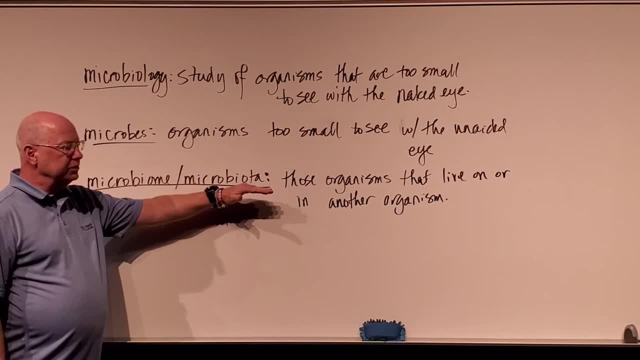 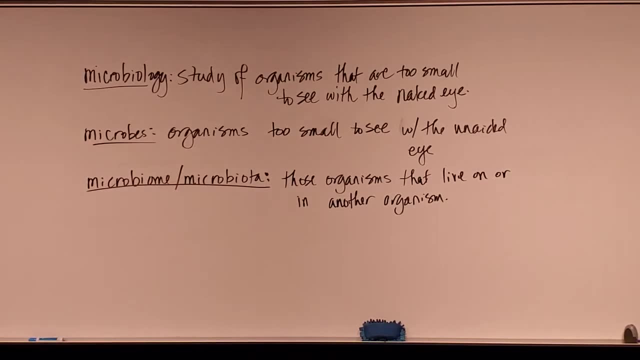 And so we would call that the microbiome, That group of organisms that live in another animal or organism that usually benefit it. They provide a beneficial, Well, they provide benefit for that organism. One of the things that we do know is that microbes can be very beneficial. 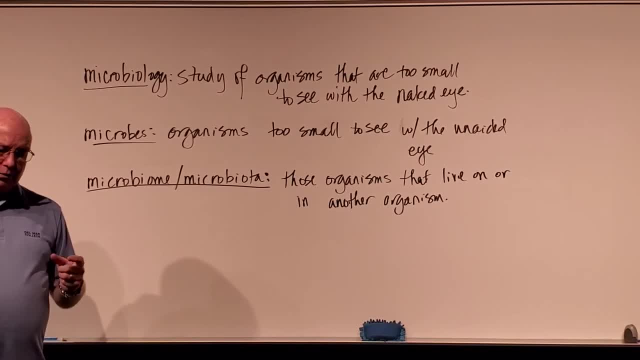 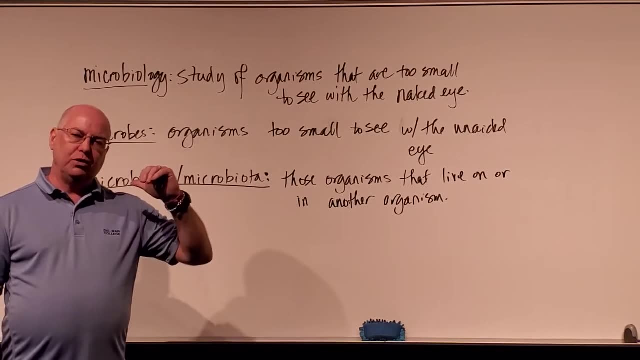 but many of them can also be very harmful. But one thing we know about all of them is that they are ubiquitous. They are everywhere on Earth that we go, Even at places where it was previously thought that no life could exist. here we are finding living organisms. 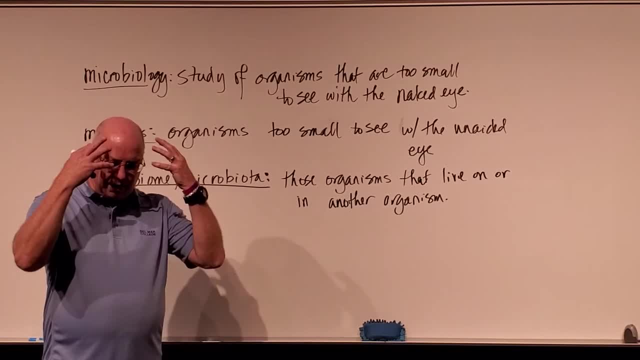 And we're going to talk about some of those in a minute. But they're on our skin, They're in our hair, They're inside our mouth, They're in our gut, They're in the urinary tract, They're in the vagina. 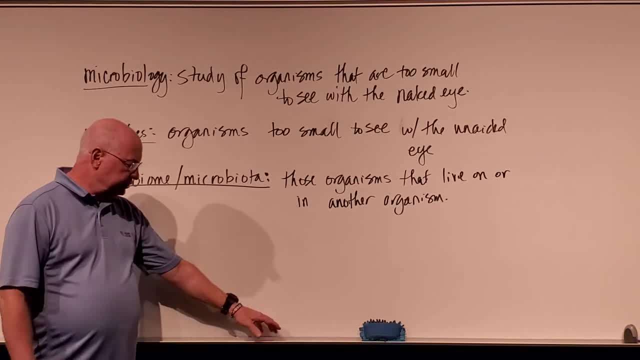 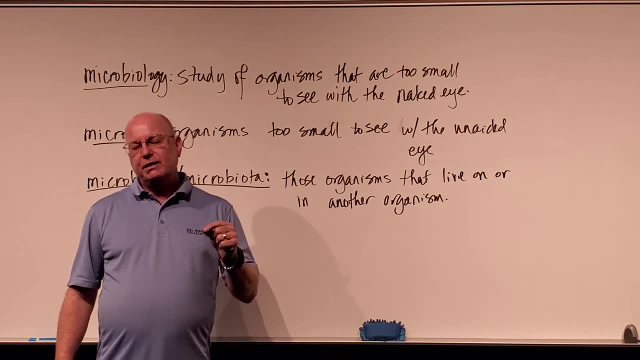 They're in the reproductive tract, They're on tables, Everything that you touch. everywhere you go, there are microbes growing everywhere. As a matter of fact, it's estimated in some instances that there are more microbes growing on your skin than there are cells in the human body. 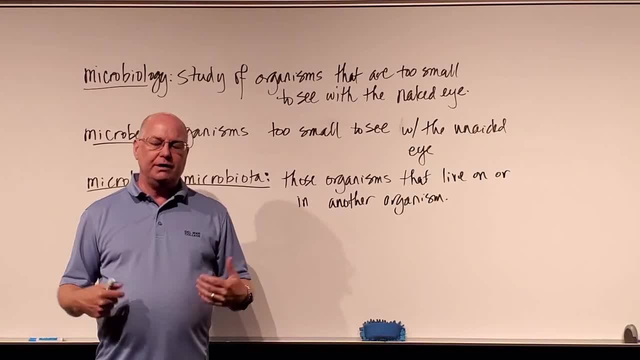 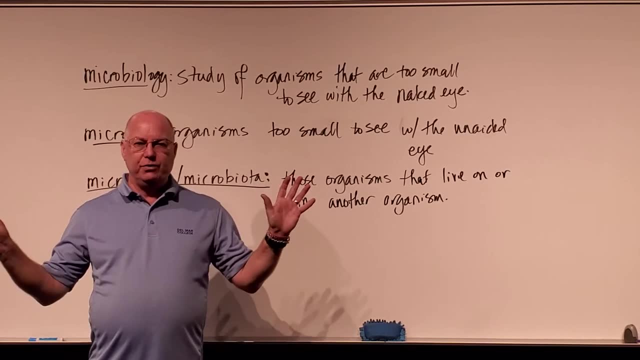 Pretty hard to fathom, but in our skin and in our body there's more microbes than the total number of cells in the human body. That's crazy, but it's true. They're everywhere. So if you think you're going to get a problem, 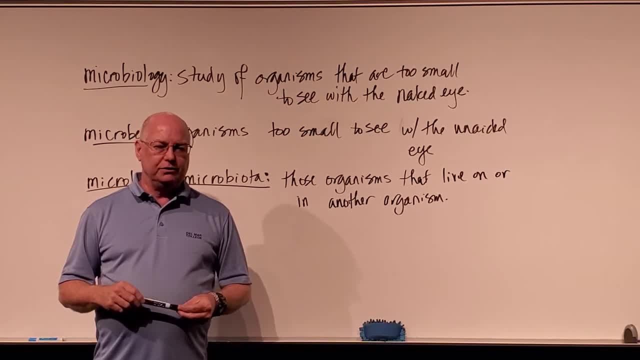 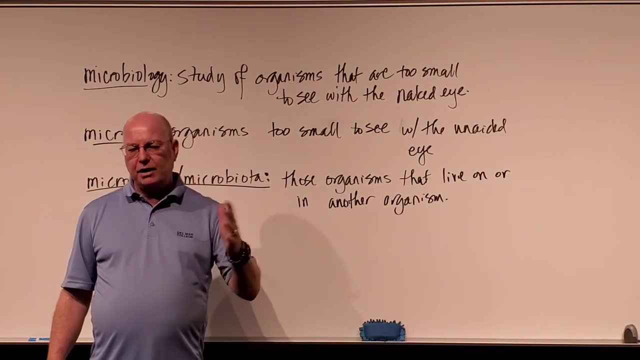 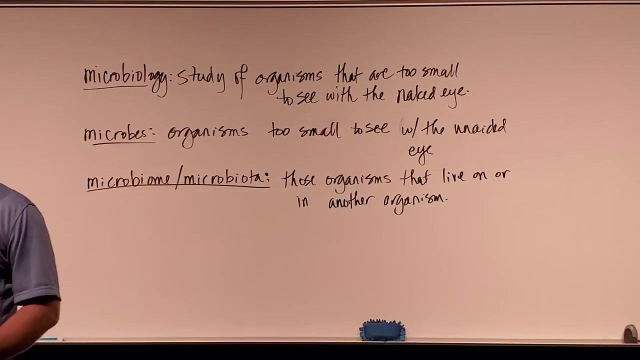 in a perfectly sterile environment anywhere. it's extremely difficult And it requires a lot of effort and energy to keep microbes out of an area, For example, like a surgical suite, or out of the room with a patient. We'll talk about all that as time goes on. 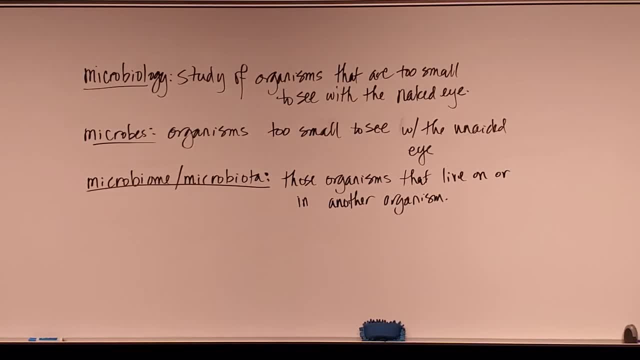 Now. so we know what life is, or some characteristics of life, We know the definitions of biology, microbiology, the microbiome. One of the things we need to look at is like, what roles do microbes play in our life? And sometimes, if I step off camera, 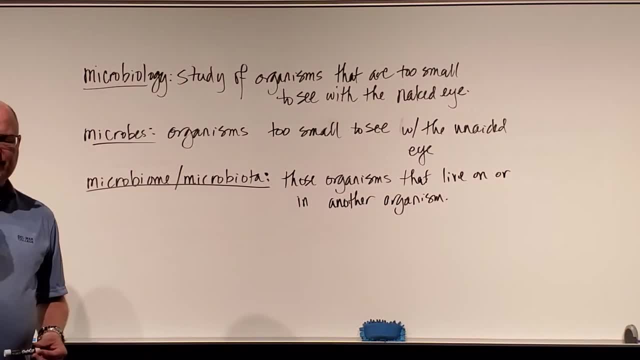 it's because I need to grab a drink, So please bear with me. After lecturing a whole lot, your throat gets a little raw, So if I take a pause and I'm off camera, forgive me, All right. So what roles can microbes play in our lives? 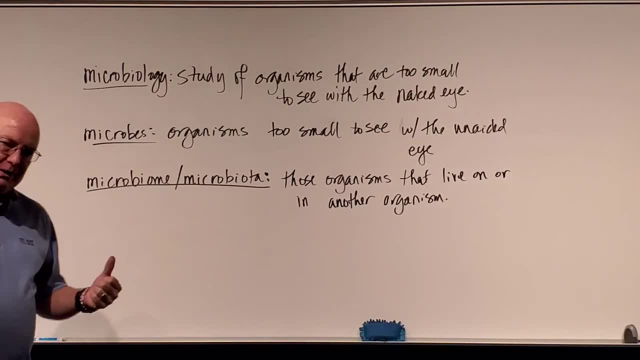 Well, one of the things we know is they impact human health both in a beneficial way but also in a detrimental way, And that's many microbes cause the pathology or the diseases that we experience. They can aid in the natural balance in nature. 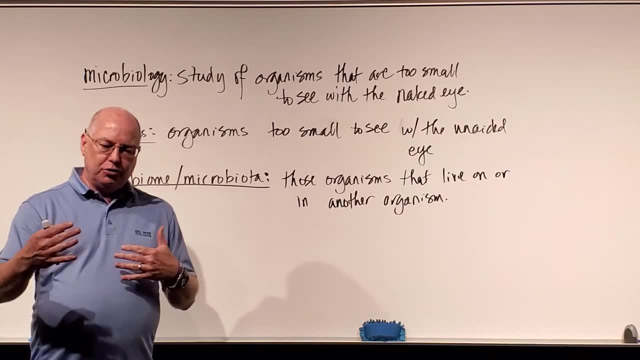 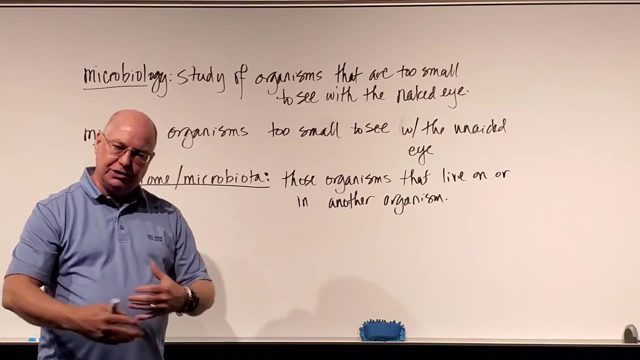 So a lot of times microbes are breaking down a lot of the stuff, like the leaves and things that fall on the jungle floor and other plants and animals. as they die They get digested and broken down, or even things in the ocean are broken down. 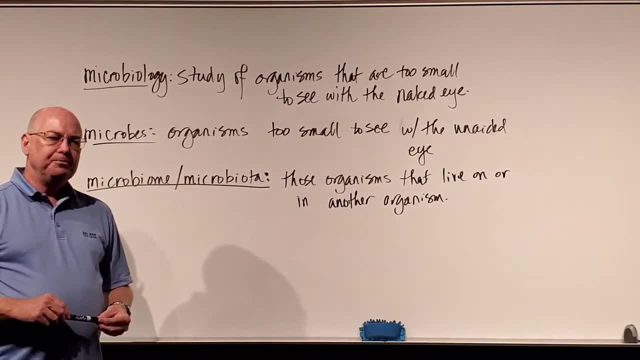 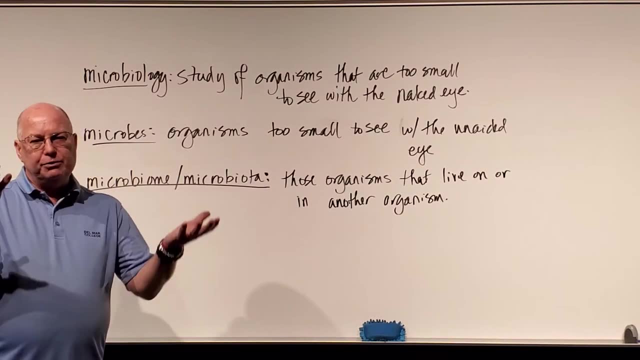 by some of the microbes there, And some of the waste products and the microbes themselves are consumed by other things. Others are consumed by other organisms, And so they can help us balance out things in nature. There is a bunch of environmental uses. 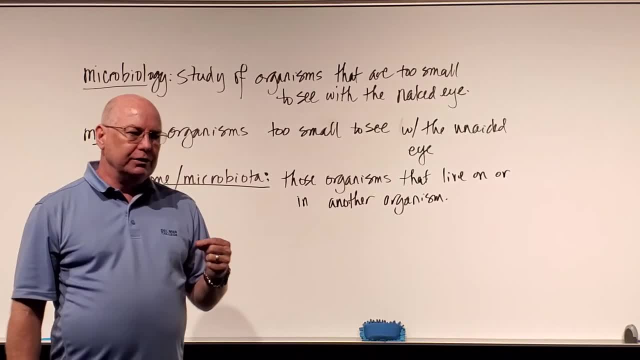 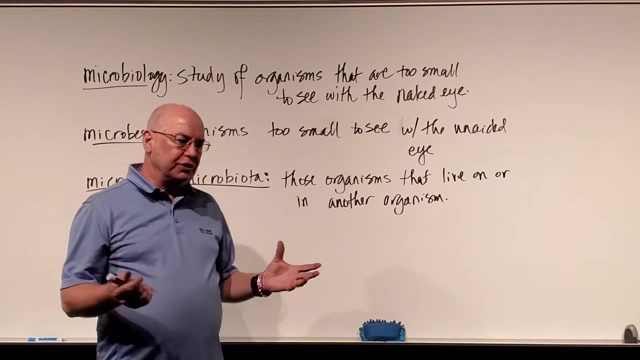 One of the things that we call is bioremediation. This is where we use microbes to break down things. There are certain microbes that are being studied that break down plastics, so that if we threw a whole bunch of plastic waste in a particular landfill, 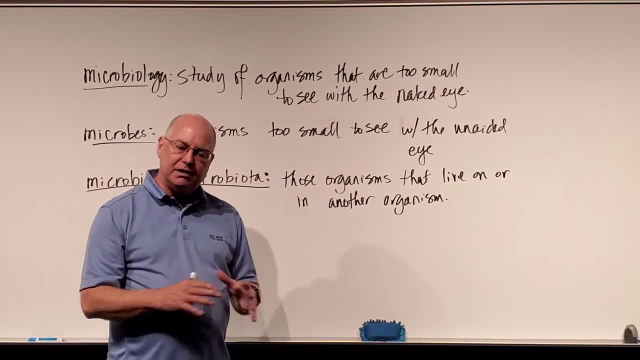 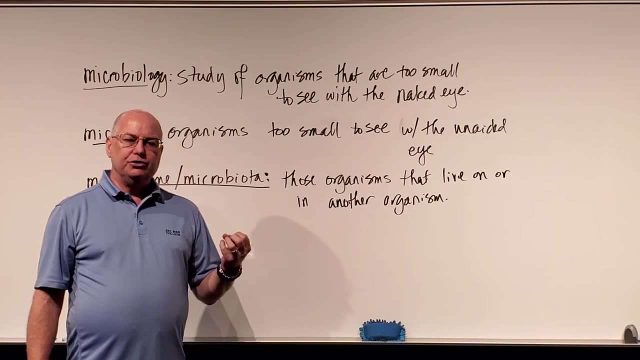 maybe if we introduce these microbes, they'll break down the plastics much faster than they would over time over centuries, Paper and other products. we can use microbes to break down a number of things, So they play a role in the natural balance of things. 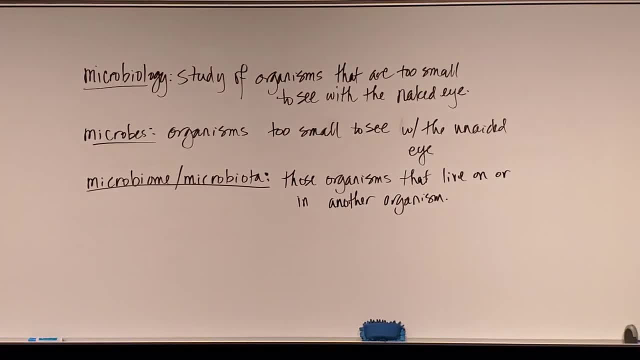 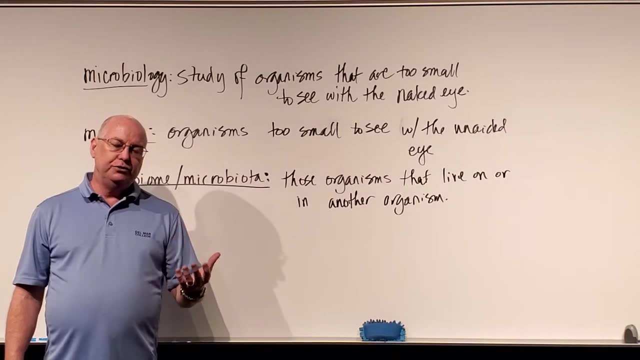 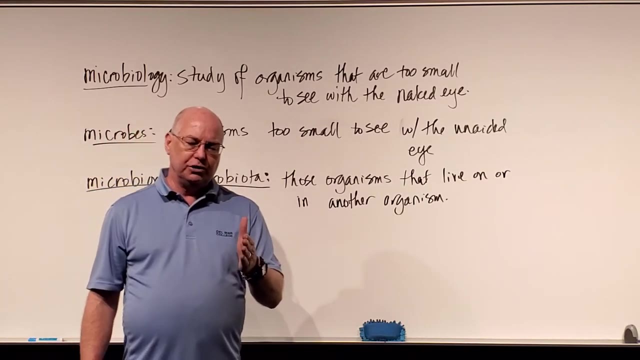 and in helping balance out the environment. Another way that microbes play an important role in our life is through what we call fermentation or in food production, And one of the ways that they do so in food production is through fermentation. Now our cells convert oxygen and glucose into energy. 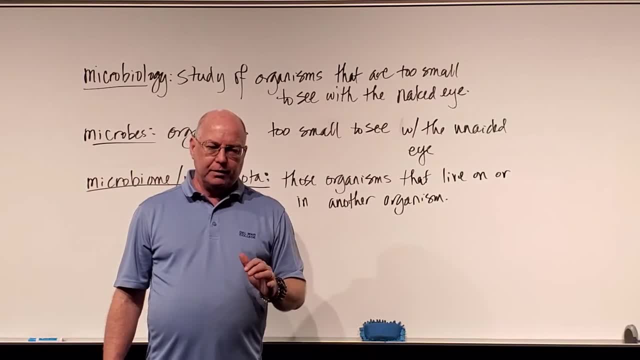 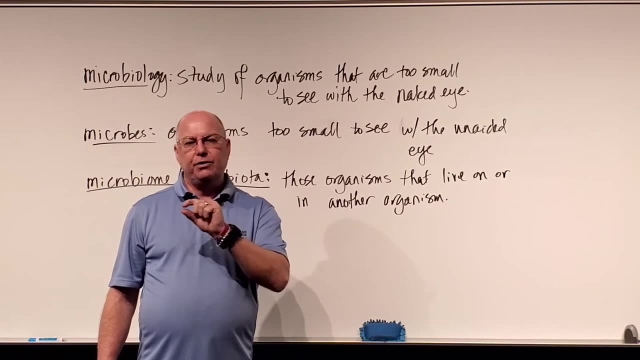 And there's a complex biochemical pathway. But because many of the microbes like bacteria are so simple, bacteria and yeast and other things can convert some of the sugar into other products like alcohol or vinegar, And that results in the production of some of our alcoholic beverages. 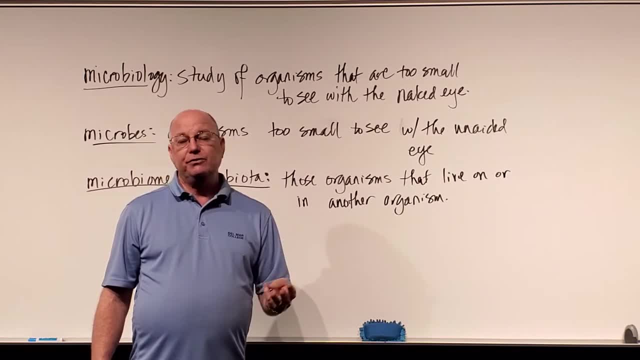 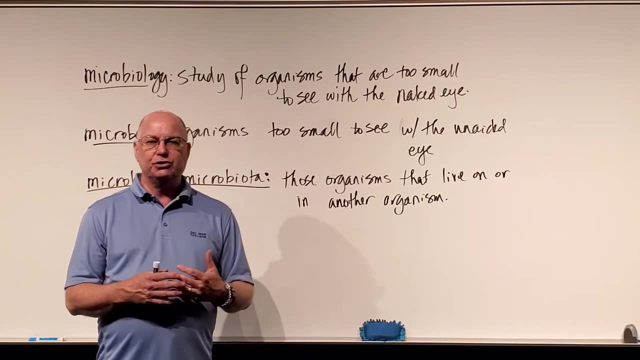 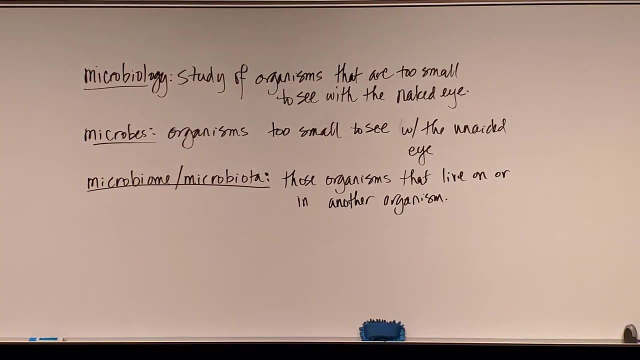 and the vinegars and things that we use for cooking into some of the foods, like molds are used for certain cheeses and yeast can help us produce some of the gases in bread that make bread nice and tasty and fluffy and soft, So they're used a lot in food production. 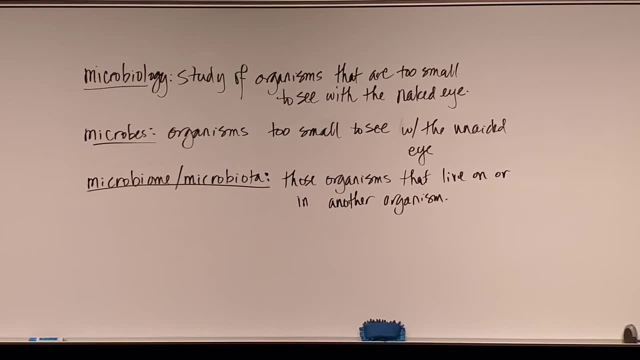 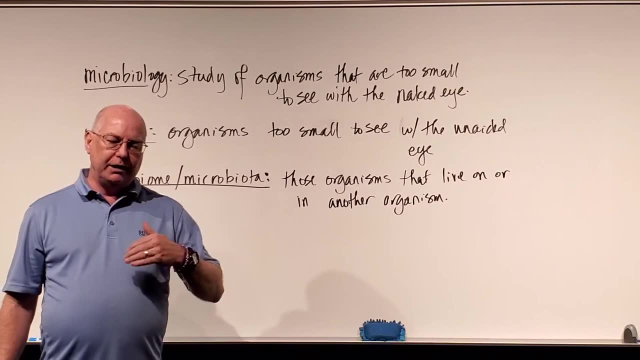 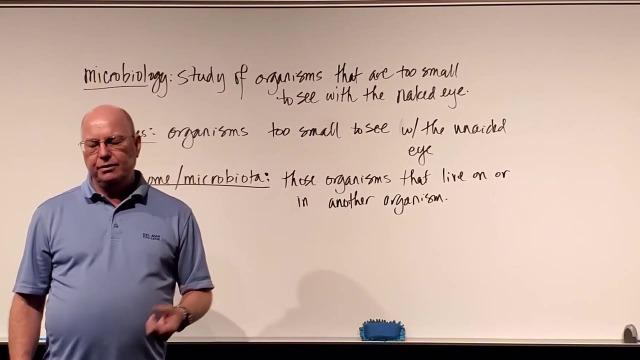 Another way that we use microbes or how they impact our life is that there's industrial uses. For example, there's a compound that's produced called cellulose. that microbes can help produce and also can help digest, by the way, other microbes, But cellulose is used in a number of 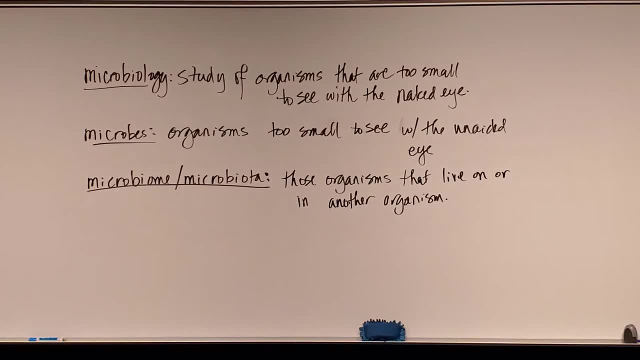 biological and environmental processes and in industrial use. They can generate a whole lot of chemicals that are used in industrial engineering, and so they play a huge role in industrial production. Also, some microbes can result in compounds that we use for pharmaceuticals, So they can be used for the production. 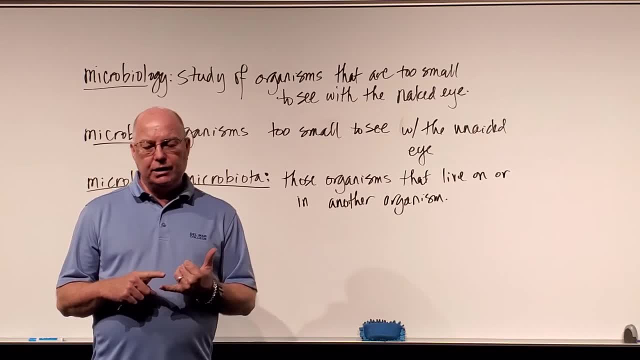 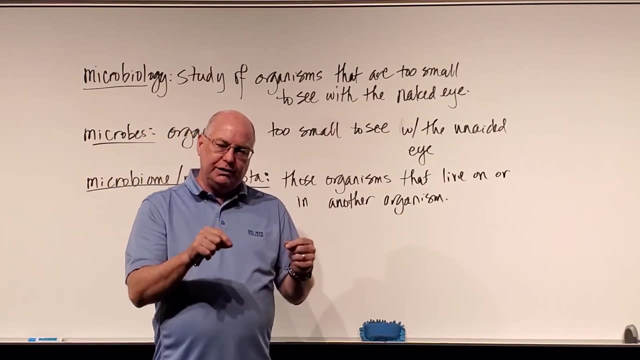 of medicines We can even. one of the roles they play is in what we call genetic engineering, where we can play with the DNA of a microbe and also alter its DNA and make it produce something, And one way we do that is in pharmaceutical production. 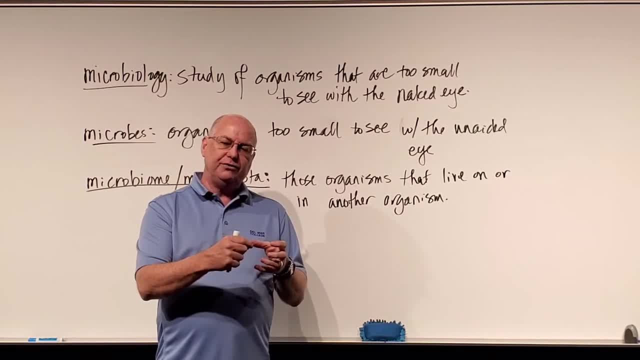 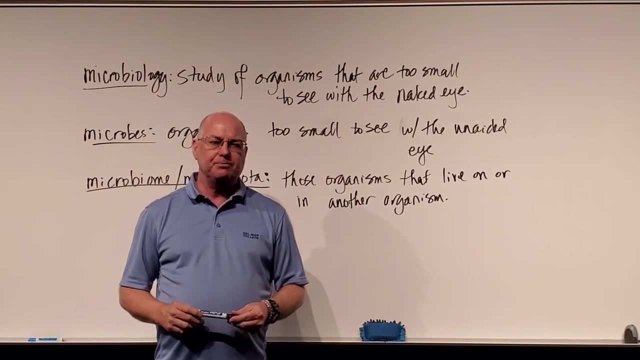 We can produce insulin now by using bacteria, by splicing a gene for insulin into them, growing them in a giant vat, filtering off all the insulin, putting it in a syringe for diabetics Where many, many years ago we just ground up the pancreas of a pig. 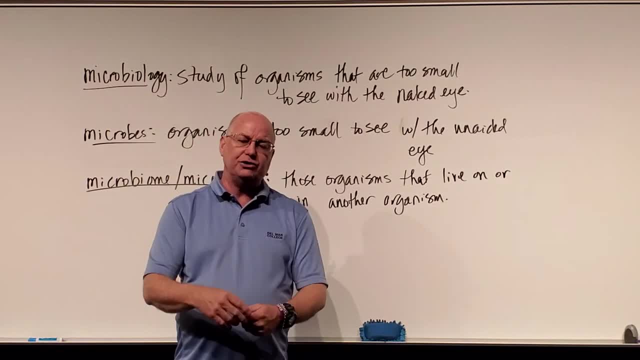 and tried to isolate it and roughly 20% or more of the patients might have a reaction to the foreign type of insulin. We can eliminate that by producing human insulin from a human gene put into a bacterium and they grow like crazy and produce tons of insulin. 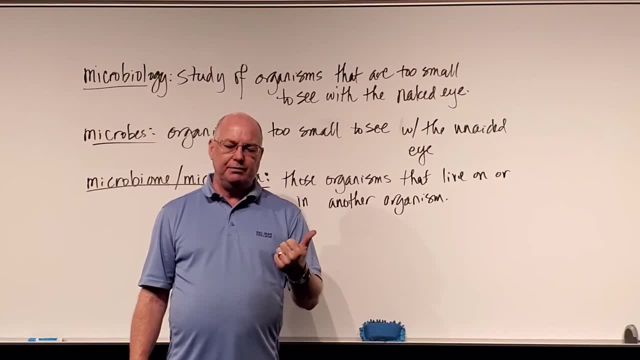 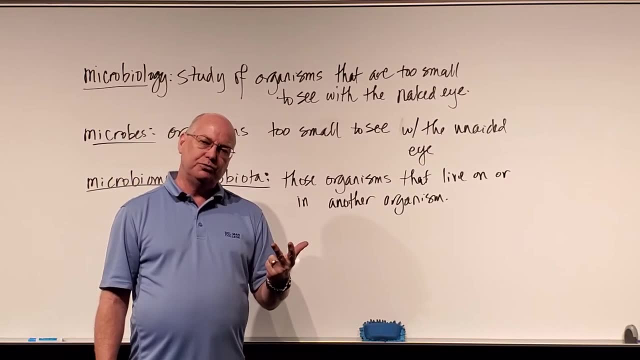 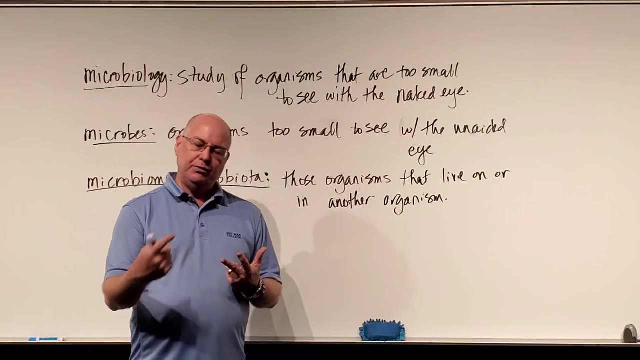 So we use microbes in genetic engineering and biomedical engineering, recombinant DNA technology. We are using microbes for pharmaceutical production In other ways. some of the bacteria, like penicillium, produces penicillin and they were discovered to produce the first antibiotics. 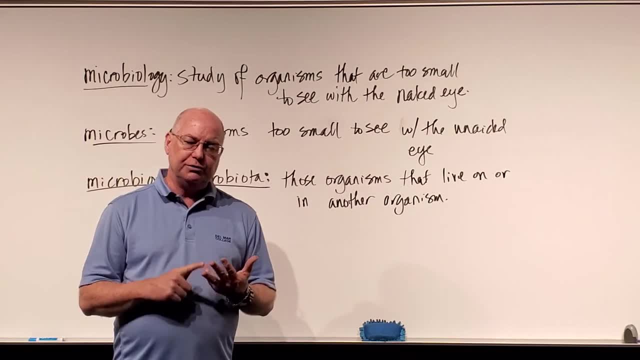 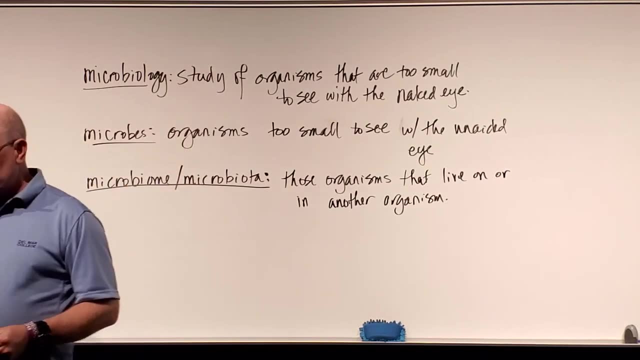 we use them in industrial uses and bioremediation and the natural balance of nature. so all of these myriad of ways we can use microbes and a lot of these notes, by the way, if you are in my class, will be posted online. they are also in the first chapter of your textbook. 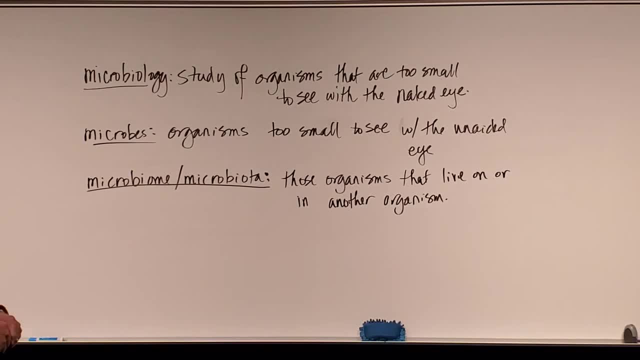 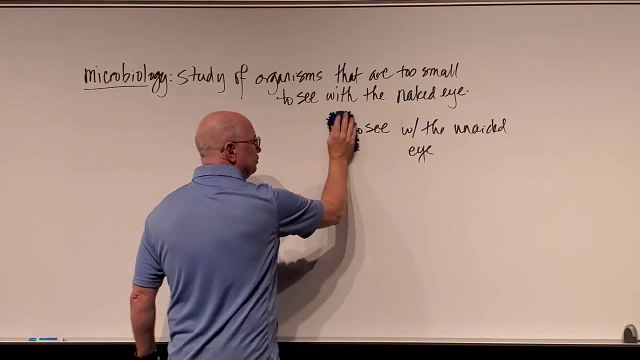 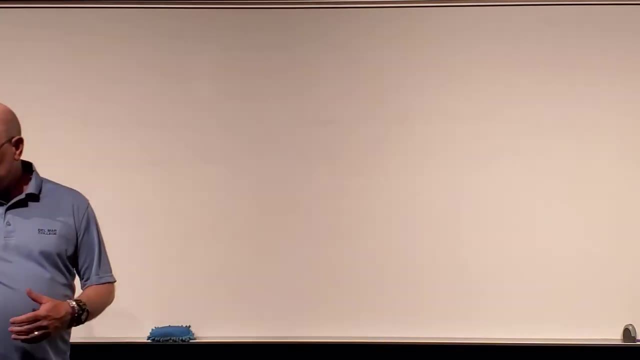 So now, why do we study microbiology? Well, if we understand how microbes work and what they are capable of, then we can use them for all these purposes. There are several ways for pharmaceutical production and genetic engineering and industrial uses. So we study microbiology. to help prevent, cure and treat diseases, to understand the underlying causes of diseases. we use them for production of food, also to prevent food spoilage. if I understand that certain bacteria or certain microbes can cause food to rot and break down, how do I counteract that? 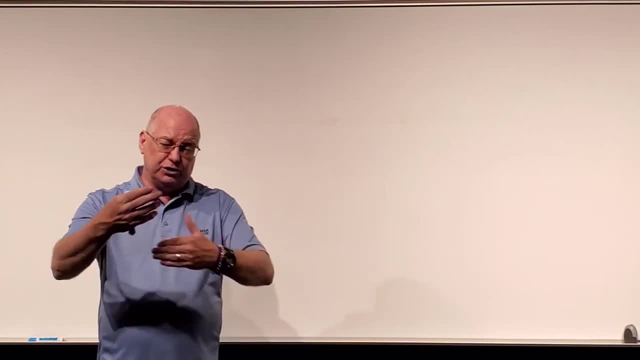 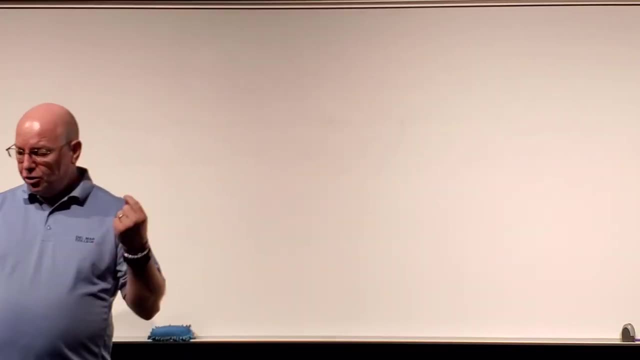 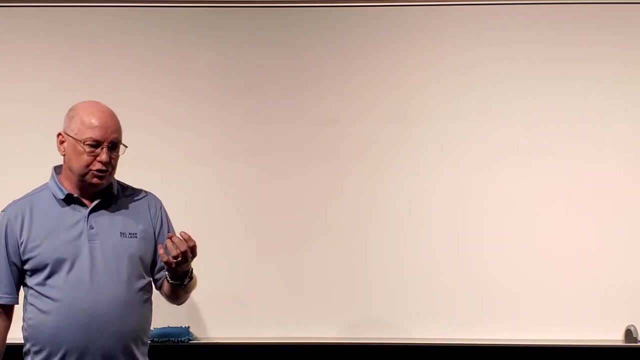 I can treat it with chemicals or I can put it in a refrigerator which slows the biochemical processes of that breakdown so that food lasts longer. so we can prevent food spoilage, we can increase food production. we can use it in industrial uses we can have, while some people are opposed to it. 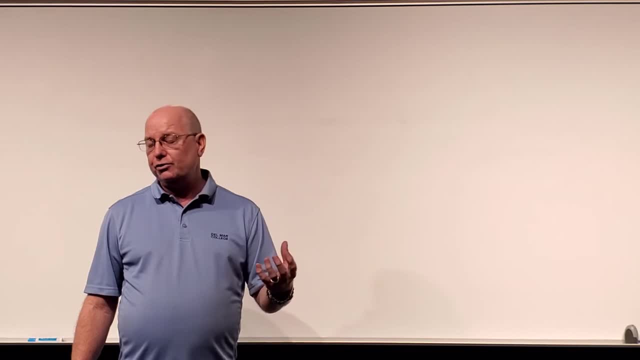 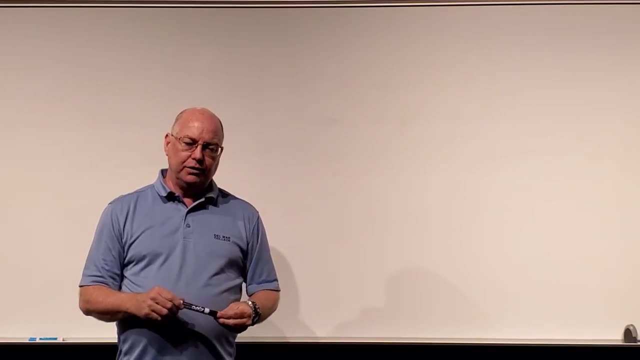 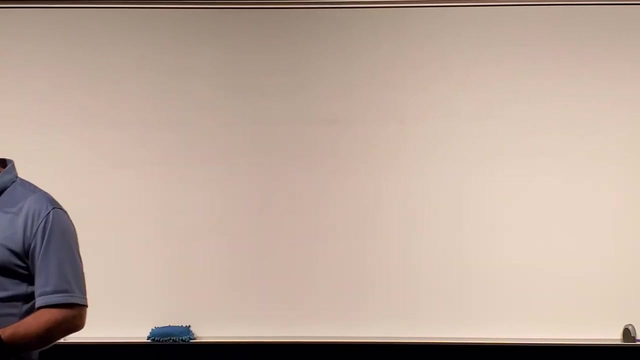 we can have genetically modified organisms, like tomatoes or other crops, where we can modify them so that they are not easily attacked by other organisms that would eat the food, or bacteria and other things that would cause the food to rot or break down, so we can use, we study microbiology for all these reasons. to prevent and cure diseases and treat illnesses, to understand the underlying causes of illnesses and diseases, to prevent food spoilage and also to develop new technologies with recombinant DNA technology. and all of this Now, a lot of important terms and definitions are needed for us to understand. 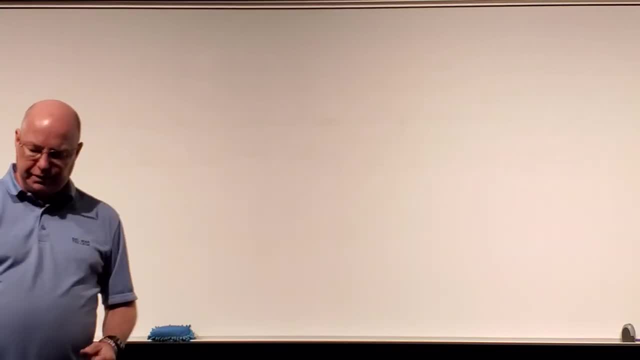 and for us to do well in microbiology to understand everything we are going to be talking about this semester. I am going to provide some terminology now, and I am going to provide some as time goes on, so bear with me. these are some of the ones you need to know for now. 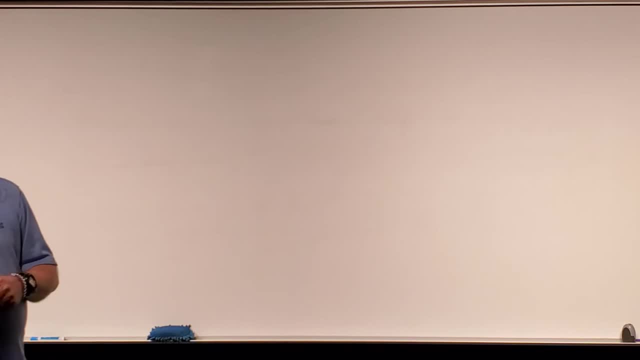 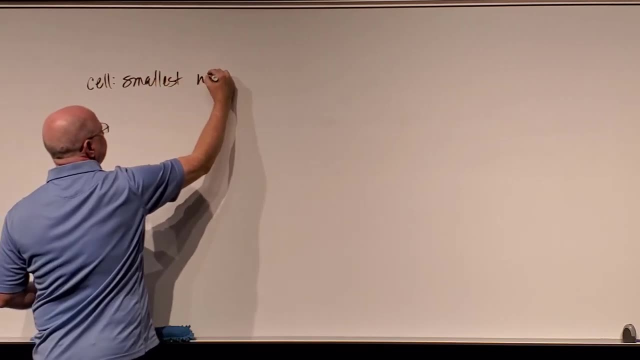 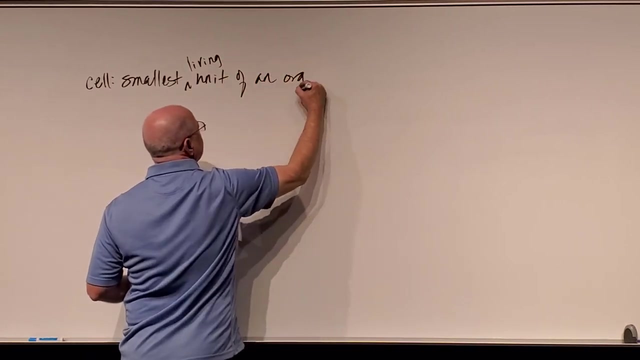 so when we talk about cell, one of the things we need to know is that a cell is the smallest unit, or we should say the smallest living unit, of an organism and, while it might require a lot of difficult technique, we can isolate some cells from an organism. 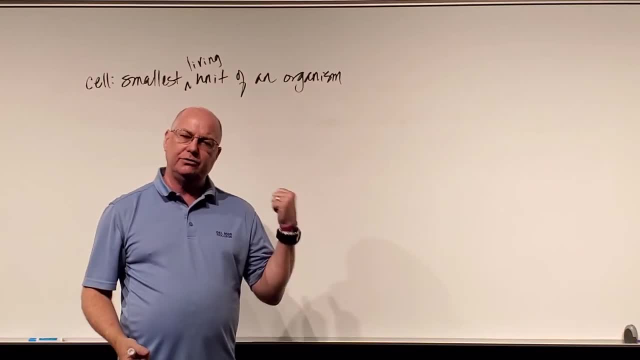 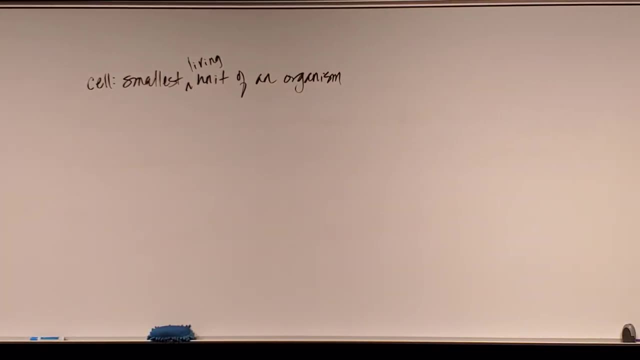 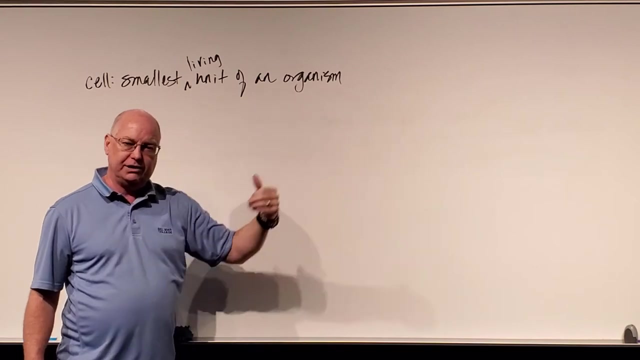 put it in a dish and they will exhibit all the characteristics, or many of the characteristics that we listed earlier, of a living organism. another way to say this is: this is the smallest living unit of an organism that can perform all of the life processes and exhibits the characteristics of life. 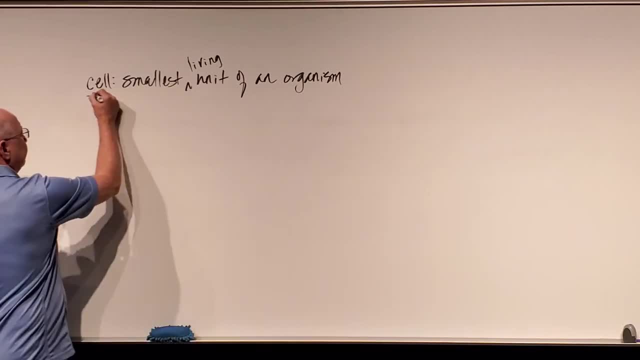 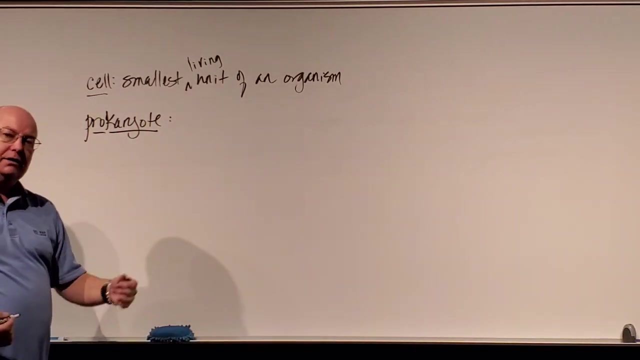 now, when it comes to cells, there are different types of cells. so when I talk about what is called a prokaryote- p-r-o-k-a-r-y-o-t-e prokaryote, or if I say the term prokaryotic, it is referring to a prokaryote. 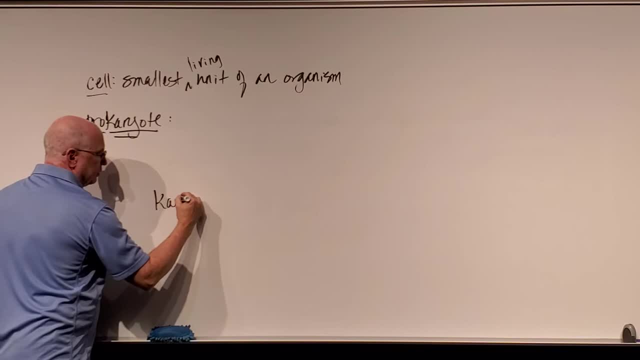 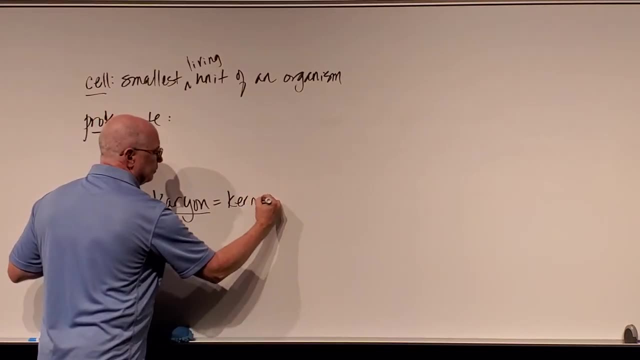 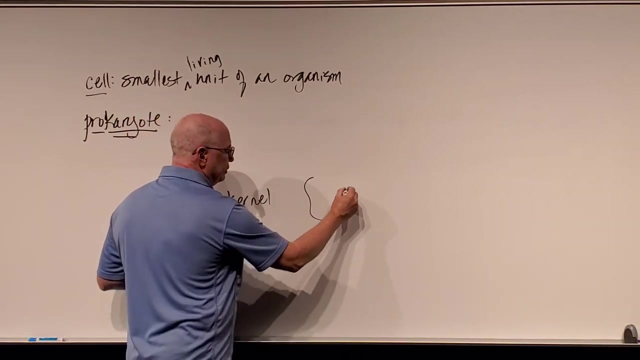 now the karyo comes from this word. karyon is apparently a latin or greek word. I think it is latin. that means kernel. now, when scientists first started studying cells under a microscope, they noticed that no matter what the shape of the cell, they always had this little dark spot. 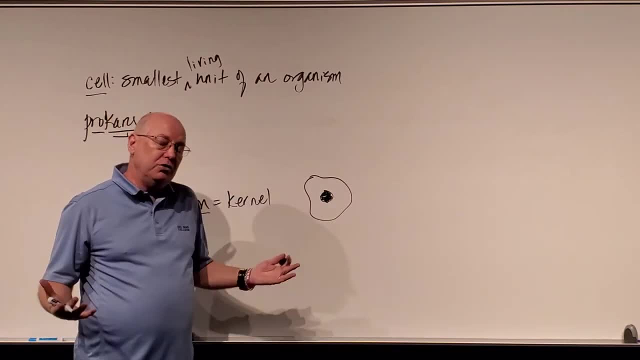 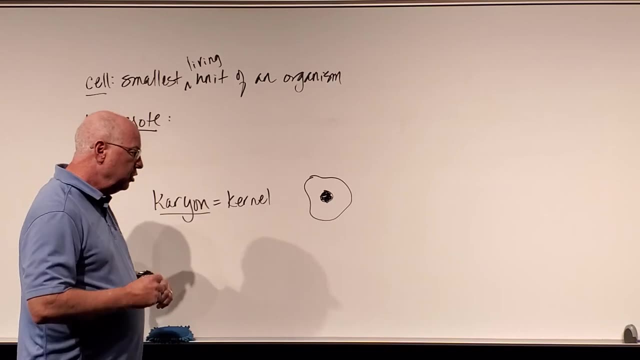 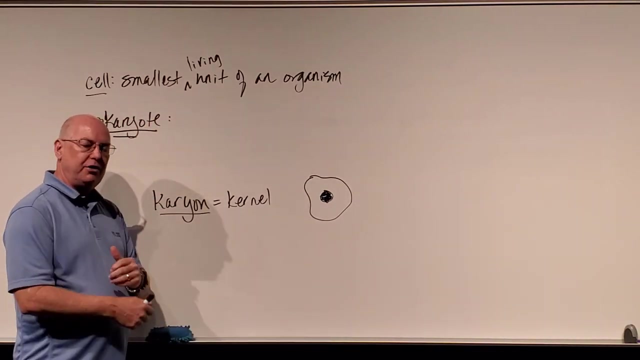 if we stained them properly in the middle. they didn't know it was a nucleus. they didn't know what it was, so they called it the karyon or the kernel, that little seed looking thing in the middle. we now know that is a nucleus, and a nucleus will define what the organelles are. and how they function a little bit later, if you haven't done that already. karyon means kernel or nucleus, then prokaryon means before a nucleus. so these are what are considered to be some of the older cells in life and some of the first cells. 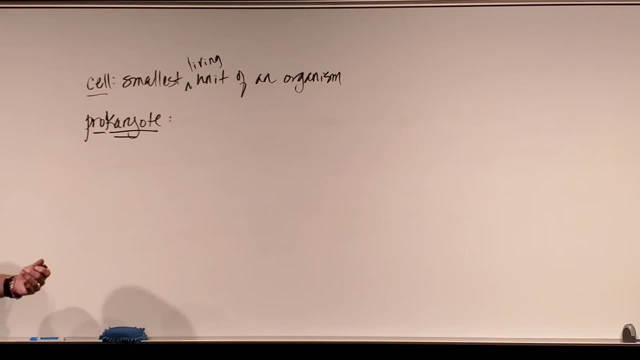 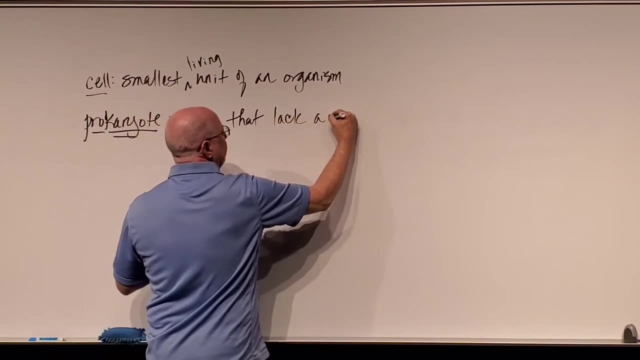 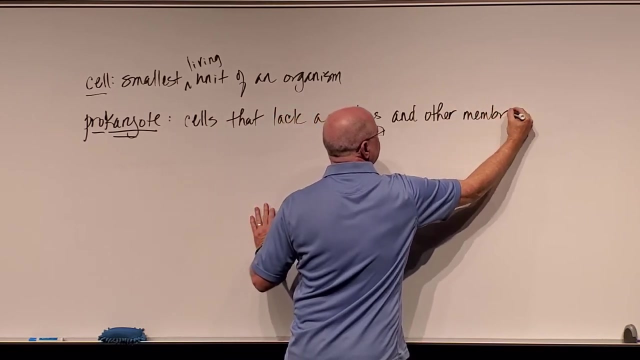 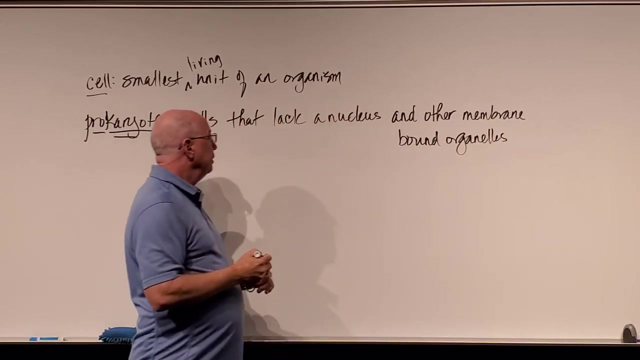 to evolve were called prokaryotes. now, one way that we define prokaryotes is we define them as cells that lack a nucleus and other membrane bound organelles. ok, you have to pardon my back, but as I teach this stuff, I realize. when I was a student. 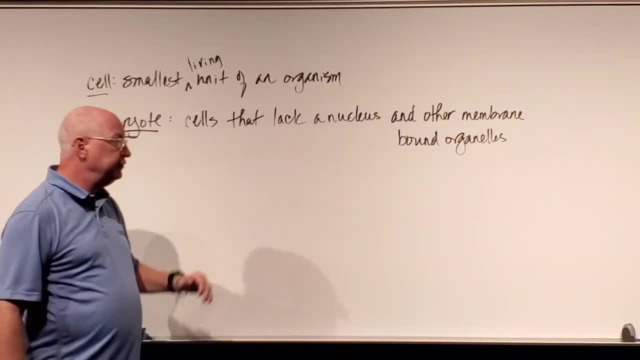 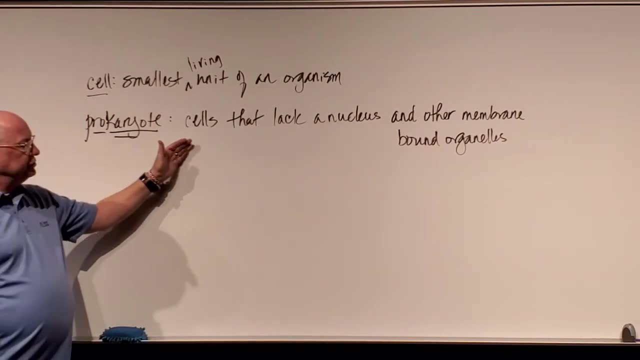 I couldn't keep up with as fast as the instructor was going through powerpoint. so the things that are important for you to know, I'm going to write out on the board so that you also have time to write them. so a prokaryote or prokaryotic cells. 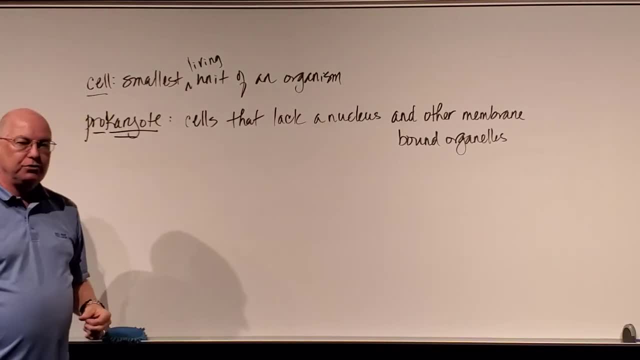 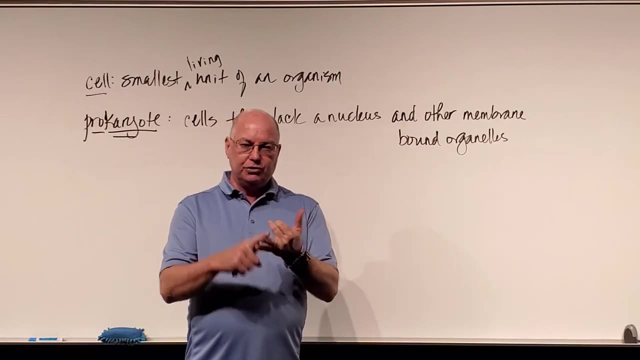 are cells that lack a nucleus and other membrane bound organelles. when we study cells in biology, you learn about the endoplasmic reticulum, which has a membrane. you learn about the nucleus, which has a nuclear envelope or a membrane, the golgi apparatus, which has a membrane. and other types of membrane bound organelles. prokaryotes don't have a nucleus. they don't have a wall around their DNA to protect it. they usually have a single chromosome with no nucleus. they have a few ribosomes and a lot of cytoplasm. 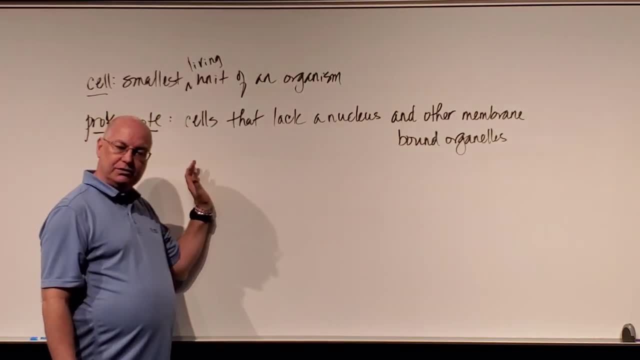 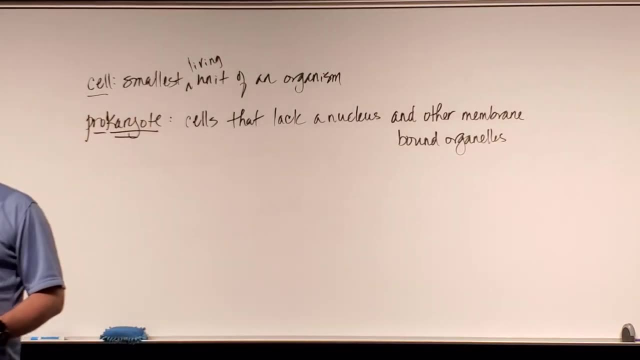 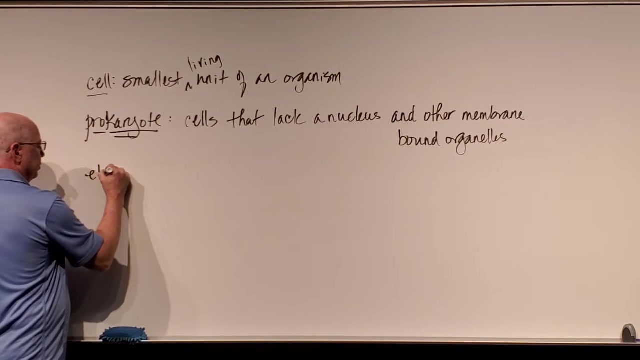 and that's about it. they're essentially a cell membrane with a cell wall, very often some DNA, usually a single circular chromosome and some ribosomes and some cytosol, and that's it now. the opposite of a prokaryote is what we call a. 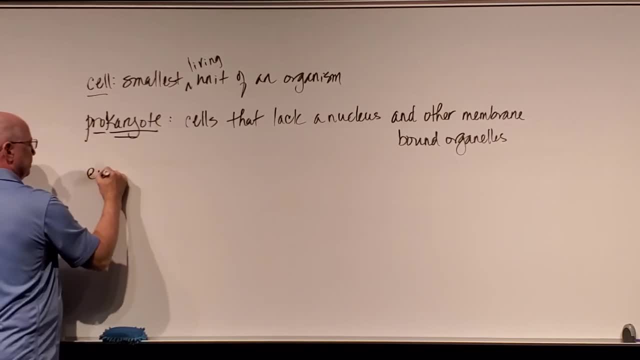 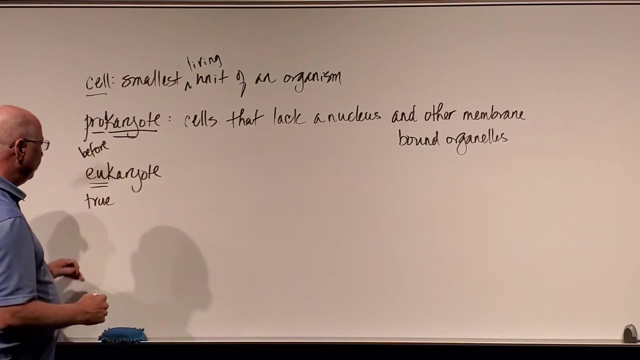 a eukaryote. let me erase that. eukaryote comes from the word true. pro means before, so before it had a nucleus. the ancient cells didn't have a nucleus, no membrane bound organelles. eukaryote means a true nucleus. these are cells. 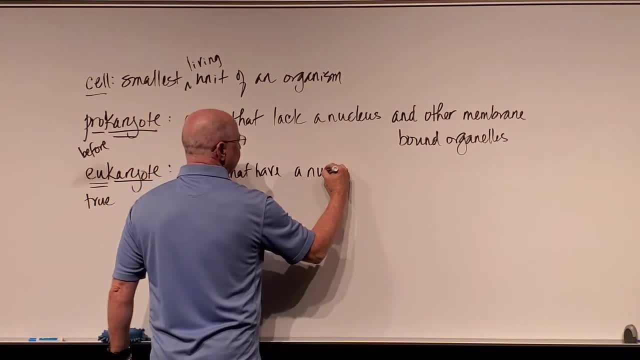 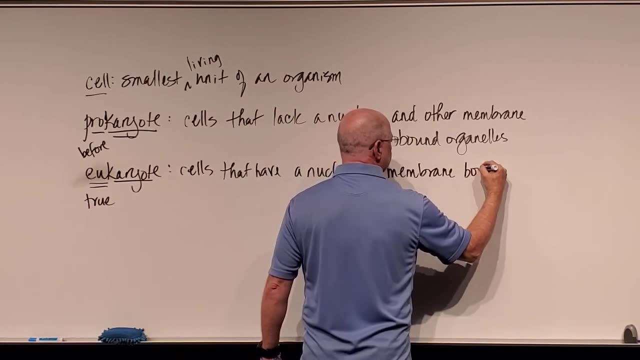 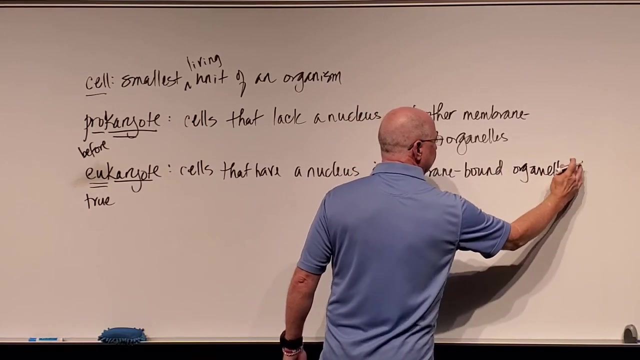 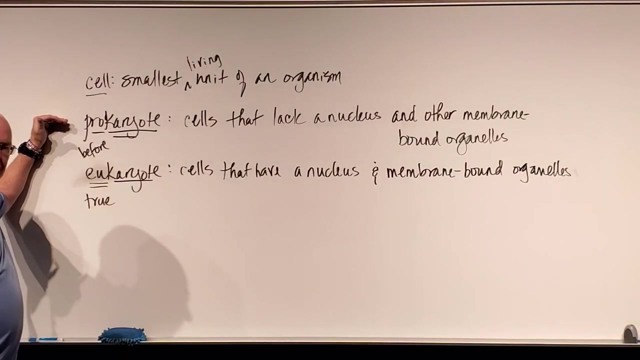 that have a nucleus and other membrane bound organelles. all the cells we're gonna talk about when we talk about living cells fall under one of these two categories: they're either prokaryotic cells, or they are eukaryotic cells, or sometimes we say they're prokaryote. 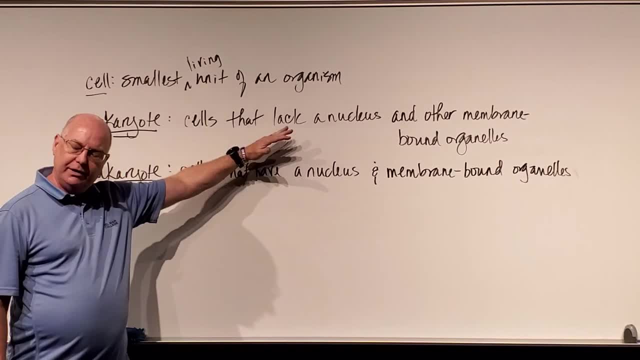 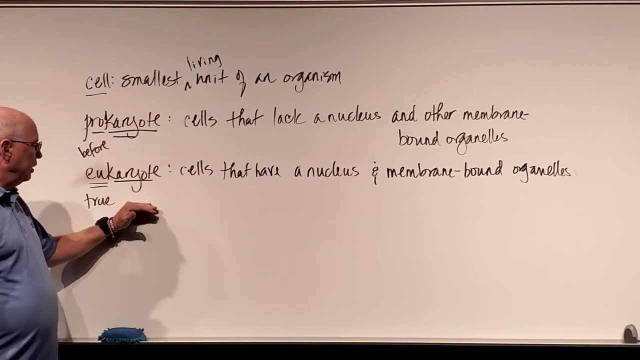 or eukaryote. prokaryotes don't have any organelles. they have a single chromosome with no nucleus around it and some ribosomes and some cytoplasm, where eukaryotes have Golgi apparatus and endoplasmic reticulum. and other types of ribosomes and a nucleus and mitochondria and all these other membrane bound organelles. now that's really, really huge. now two other definitions that we can talk about. sometimes we're gonna talk about unicellular prokaryotes or unicellular eukaryotes. 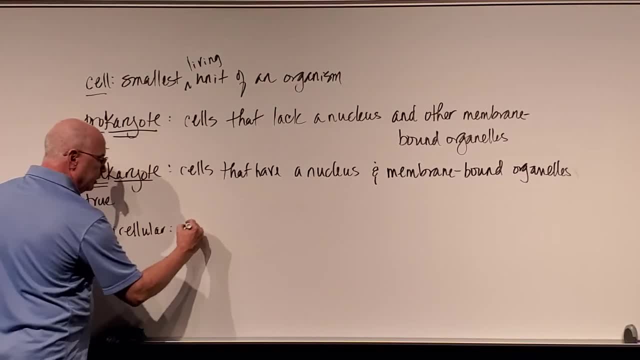 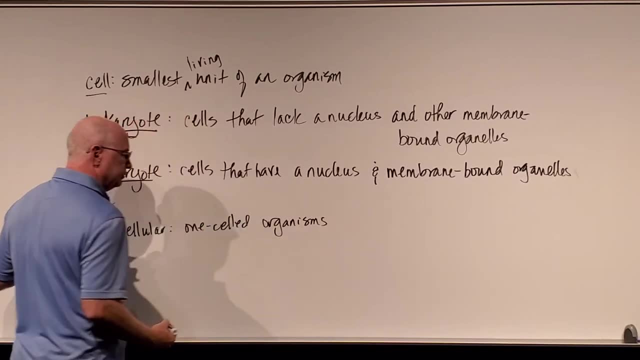 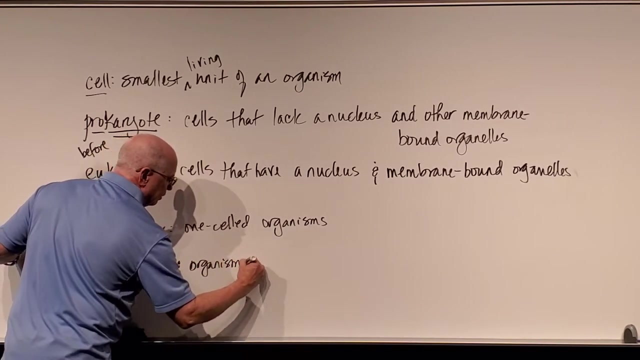 uni comes from the same word as uno, which means one, so these are one celled organisms. the entire organism is made up of a single cell. the opposite of that would be multicellular organisms. when we talk about multicellular organisms, these are organisms that are made of or comprised of. 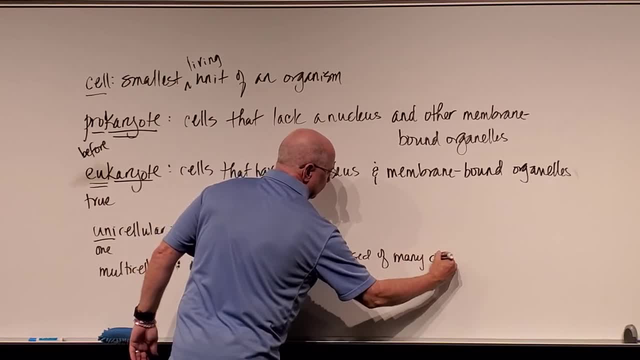 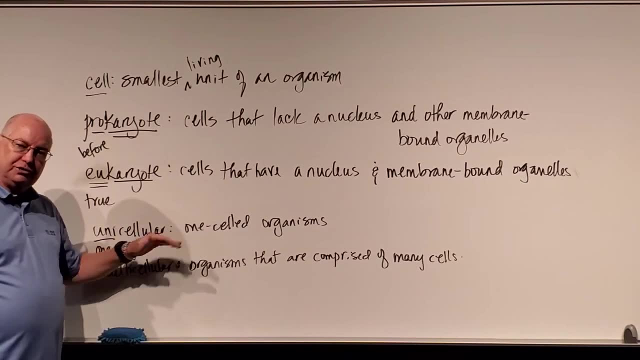 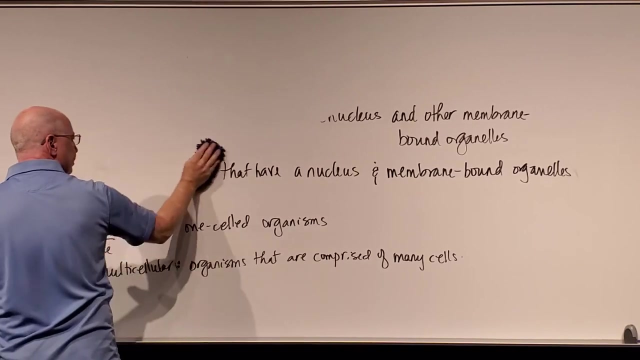 many cells, like humans, are multicellular. most bacteria are single celled organisms. now some additional definitions that we're gonna talk about. we're gonna do a lot of definitions in the beginning and I'm gonna finish up with these definitions in a moment, and then we'll do another video. 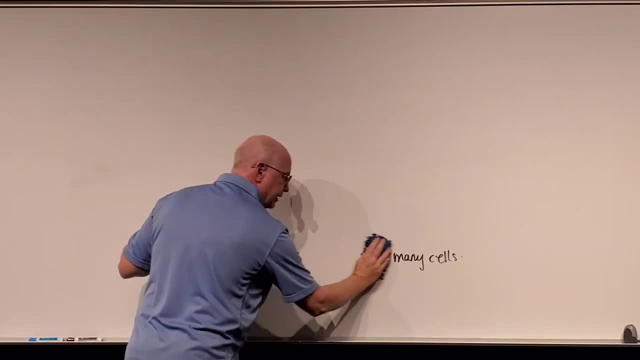 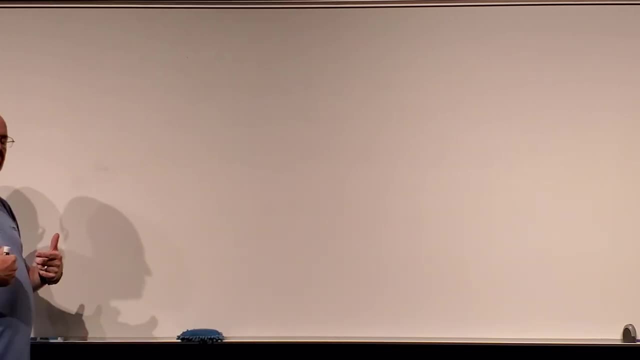 on the history of microbiology and all this intro level stuff. so when we talk about unicellular and multicellular organisms and prokaryotes and eukaryotes, one of the things we talk about is their mode of reproduction, and there's two ways that organisms can reproduce. 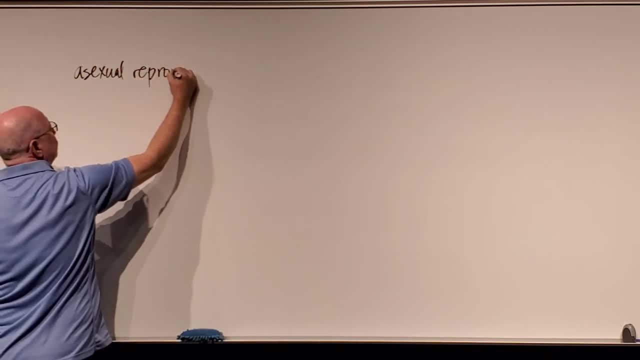 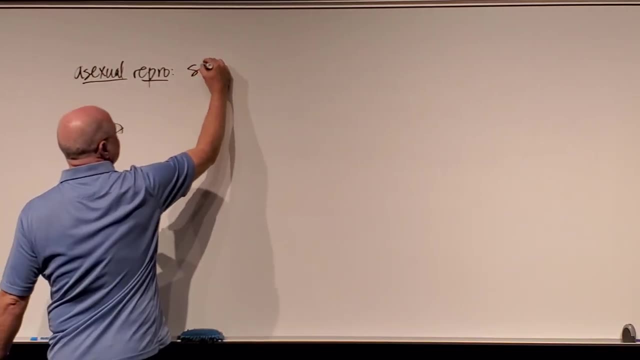 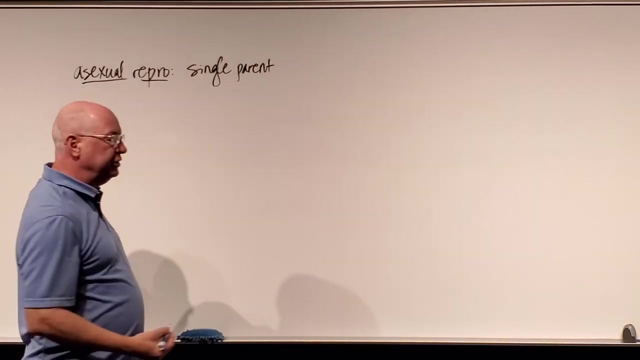 there's what we call asexual reproduction, and I'm not gonna write out the word reproduction, I'm just gonna put repro on the board. but asexual reproduction is when you have a single parent. you only need one. you don't need the other, the opposite gender or sex. 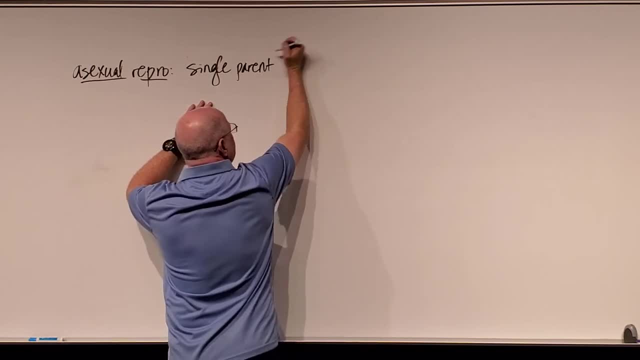 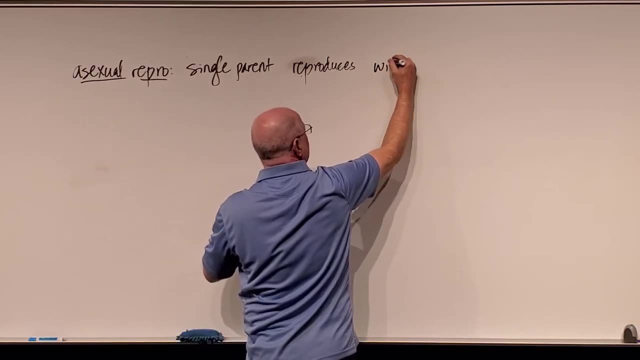 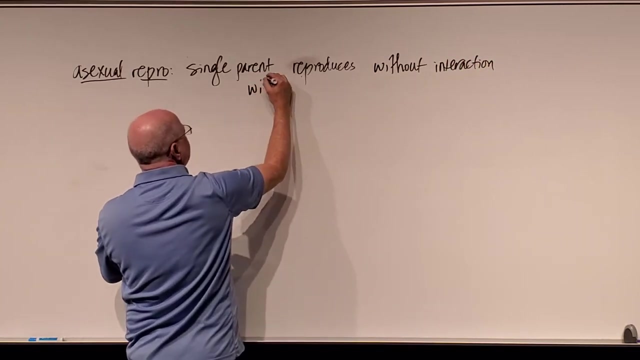 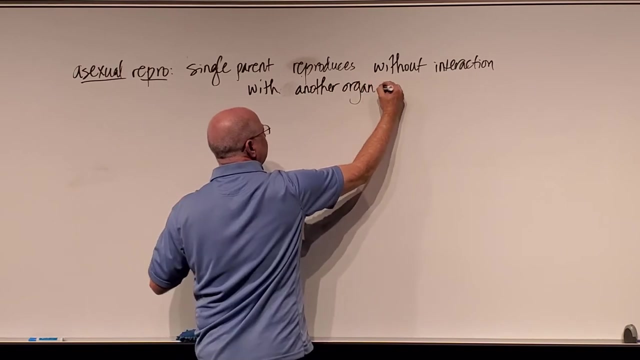 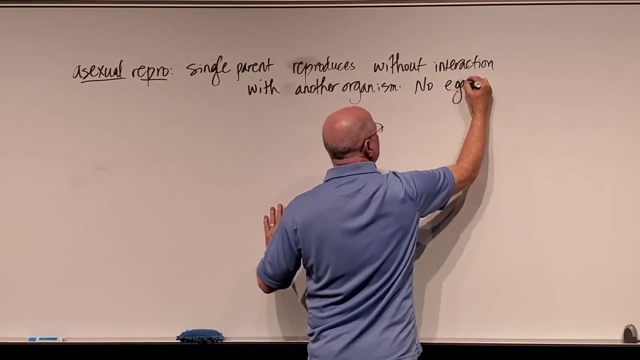 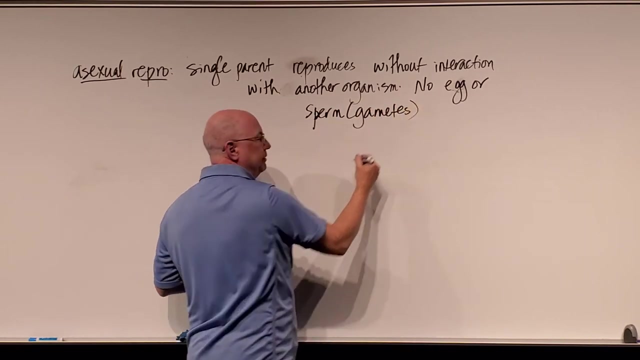 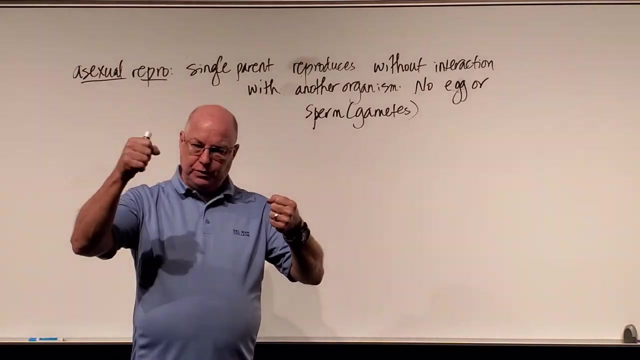 or another partner. but when a single parent reproduces without interaction with another organism, there is no egg or sperm, which we often refer to as egg, as gametes. they don't require any gametes, no egg or sperm to reproduce. so in sexual reproduction we need a sperm and an egg. 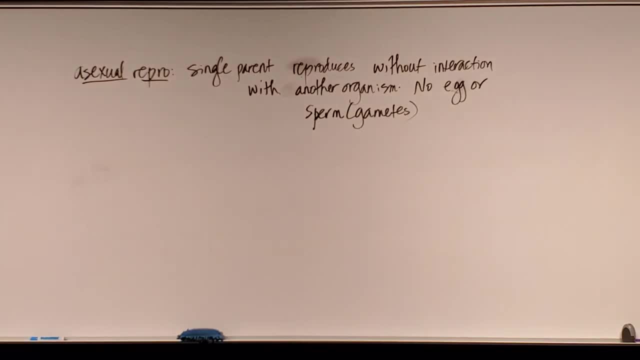 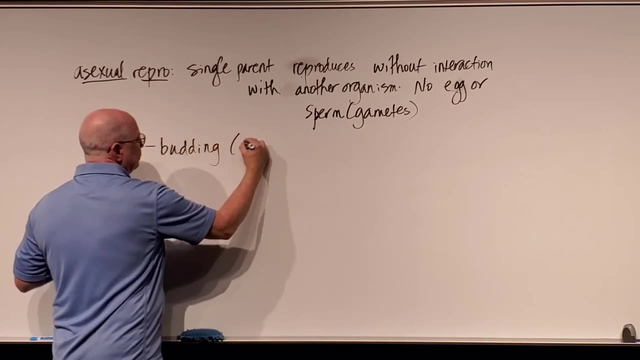 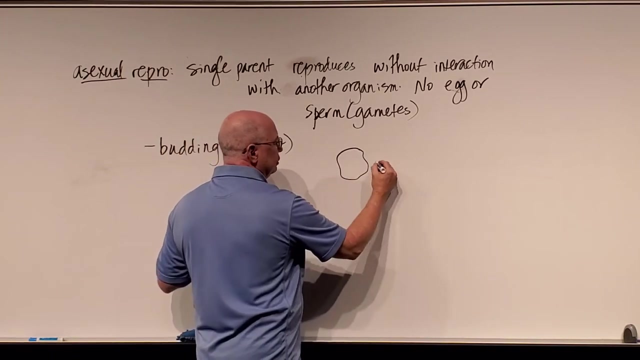 or the gametes to fuse together the male and the female gametes, and a couple of ways that this happens is by what we call budding, for example in yeast. some yeasts have the ability to bud, which means if I have a little yeast cell here over time. 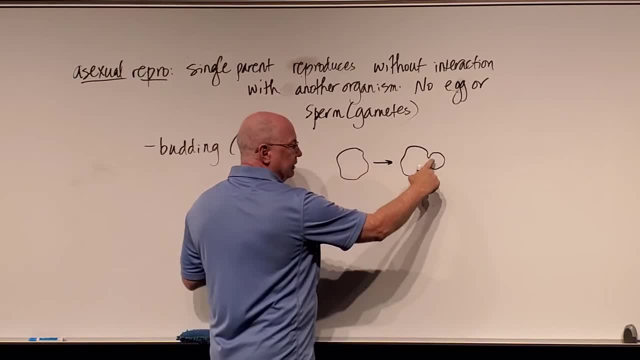 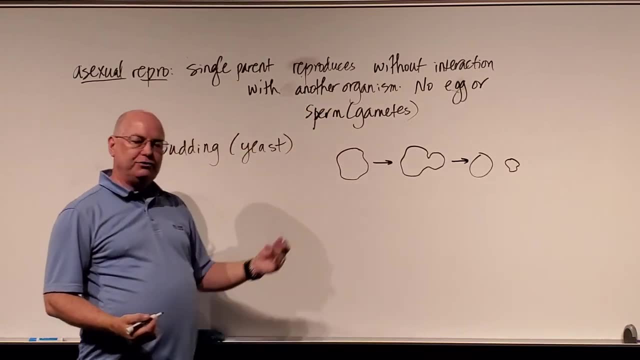 can start to package a whole bunch of its own stuff in this little bud, like its DNA and its organelles, and then over time it will pinch that little ball off, and now I have two yeast cells. so we call that budding another way that some organisms 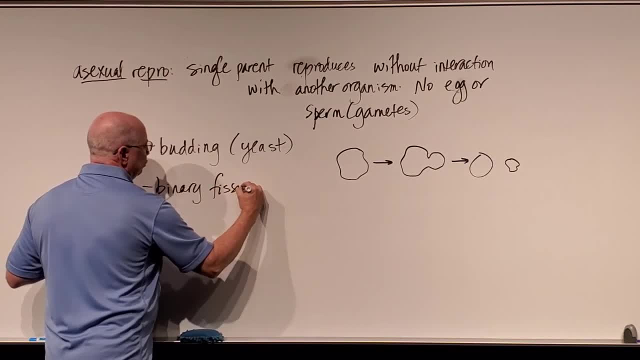 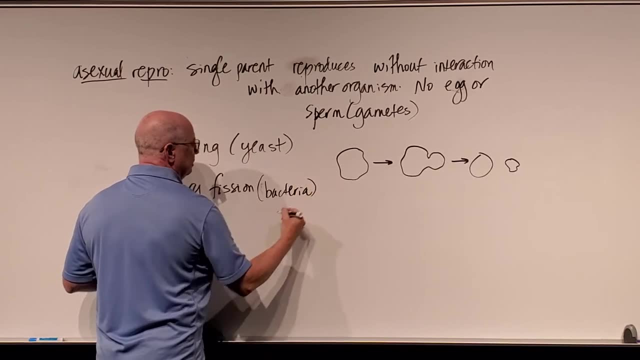 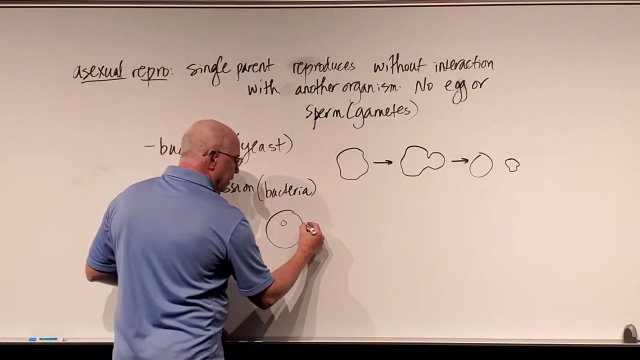 can divide is by what we call binary fission and, in this situation, an example of an organism that can do binary fission, by the way, is some bacteria. if you have a bacteria with its single chromosome, no nucleus, just a single circular chromosome, what will happen is it will reproduce that. 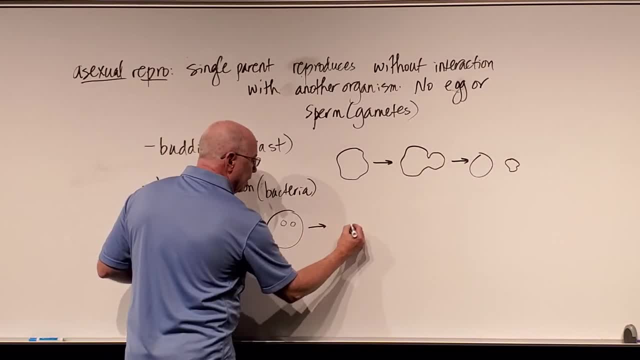 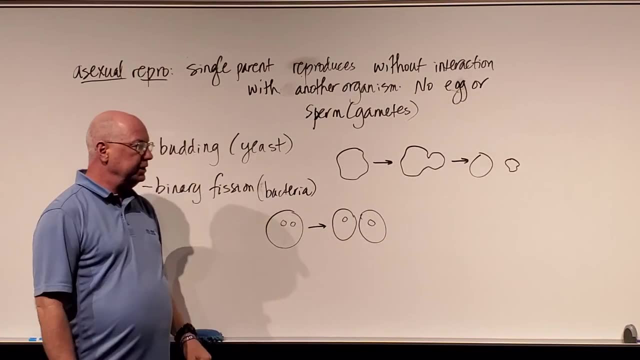 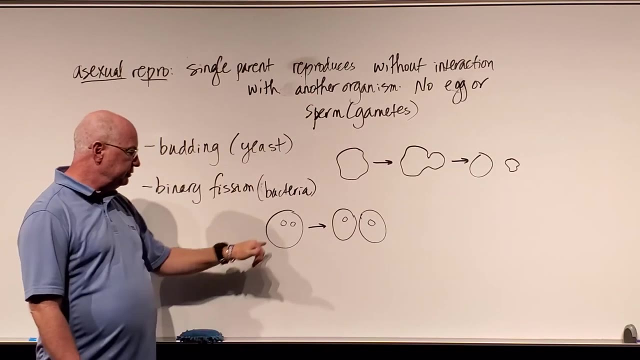 single circular chromosome through DNA replication and then it will split in two. it literally divides in two and I have two identical clones, each with the same genetic information. so some organisms can bud, split off a little piece of themselves. it's going to grow into a whole new organism. 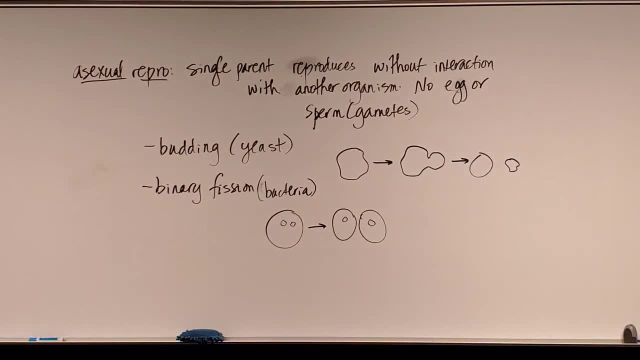 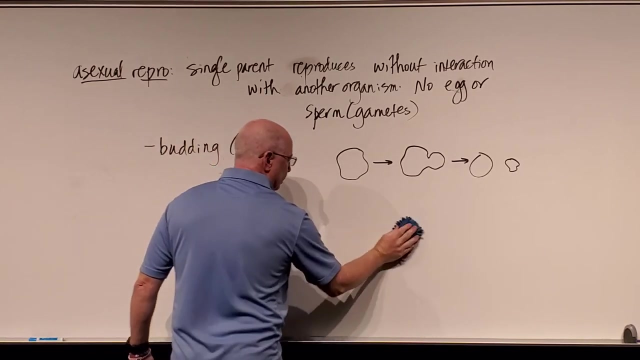 and some organisms have the possibility of undergoing binary fission. okay, the opposite of asexual reproduction is going to be sexual reproduction. so I'm going to erase a bunch of this and we're going to talk about sexual reproduction a little bit, not in great detail. we do that in human anatomy and physiology. 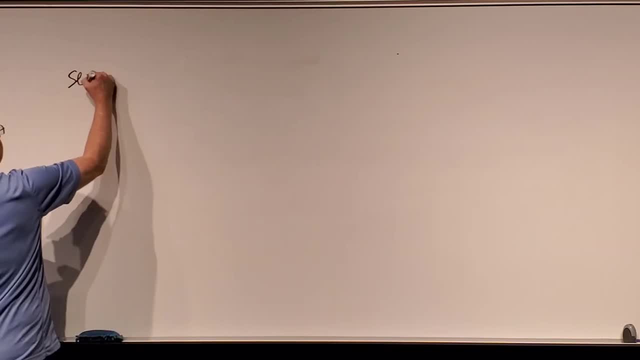 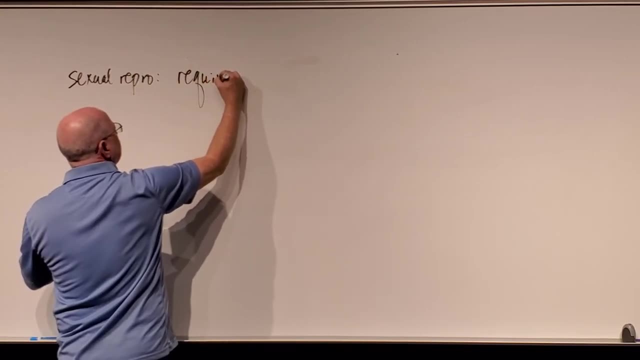 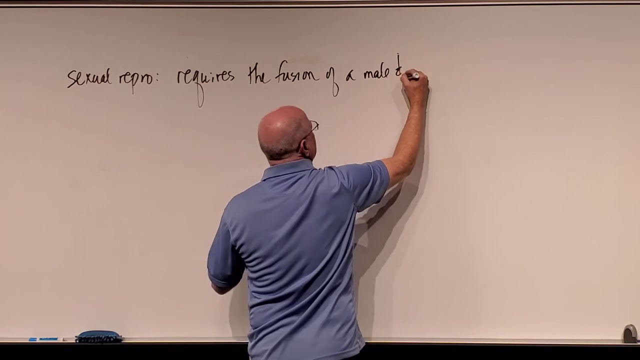 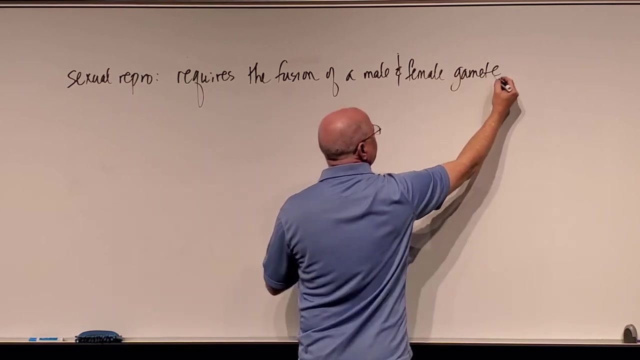 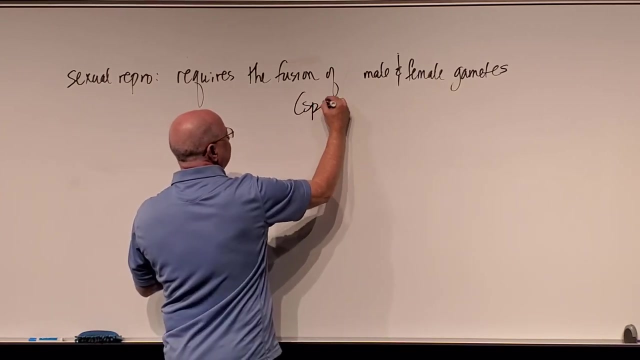 but the basics are in sexual reproduction. it requires the fusion of a male and female gamete, or the male and female gametes- we'll take the word of male and female gametes- that would be, the sperm from the male and the egg from the female must fuse together. 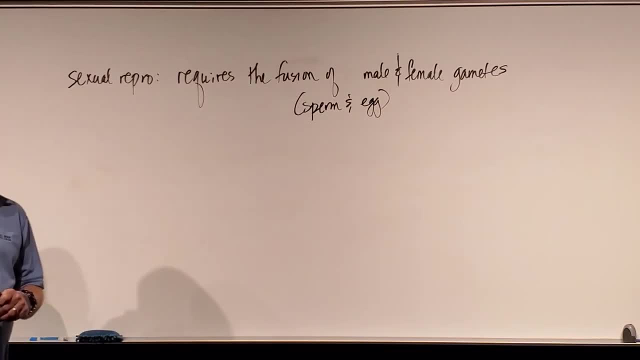 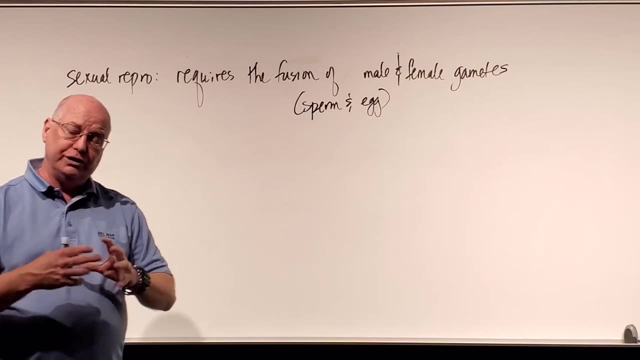 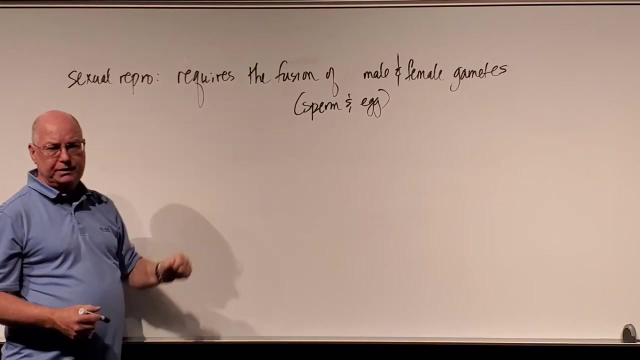 to form a complete organism and you get some of the DNA from the male and female gametes from the male parent and some of the DNA from the female parent, and this results in a lot of genetic variation. so it requires the interaction of two organisms to share the sperm and the egg. 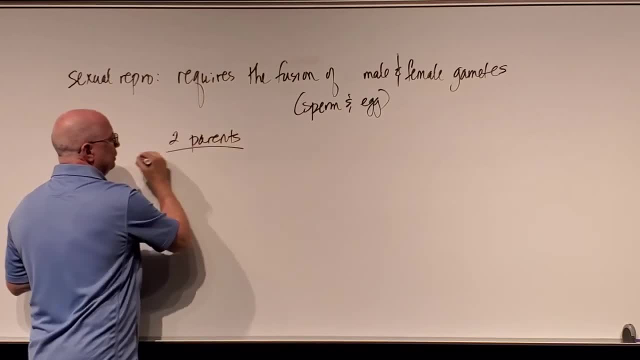 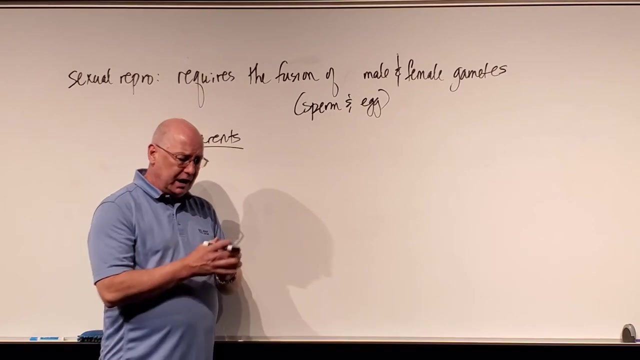 there are two parents involved in this process usually, although there's occasionally where a plant or two can mate with itself, but we're not going to worry about that. so the advantage of asexual reproduction is it's very simple and these organisms can multiply rapidly under the appropriate conditions. and increase in number from one to billions overnight, like some bacteria. the advantage, the disadvantage of asexual reproduction is that they are all genetic clones and if they're all in a tight little community and I have some chemical that can kill one, that chemical can wipe them all out. 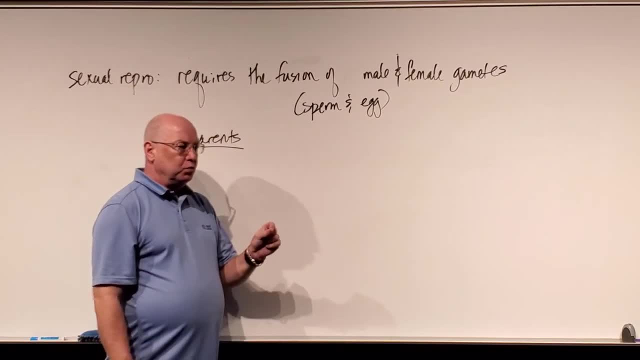 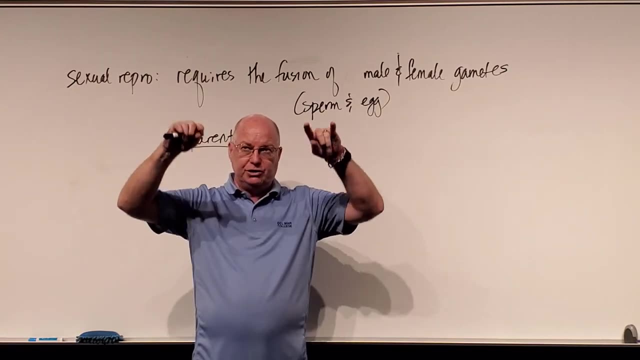 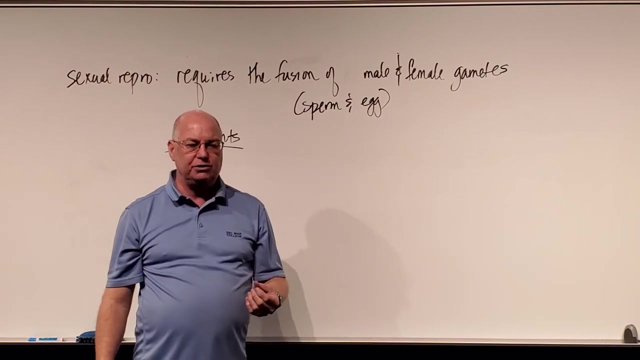 and kill an entire colony of bacteria and kill them all. where in sexual reproduction? because we are mixing the DNA of two organisms, which is a combination of the DNA from the previous generations. we get these very complex changing mixtures of DNA, of genetic material that may allow that if some disease 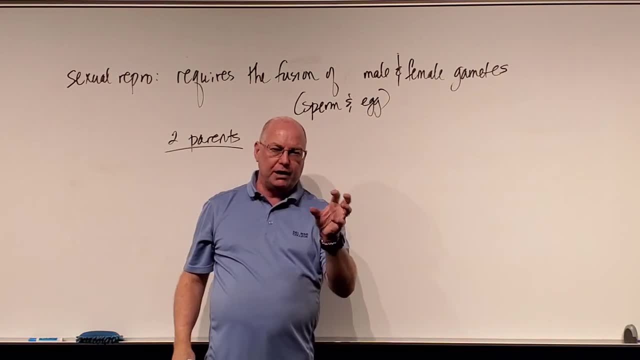 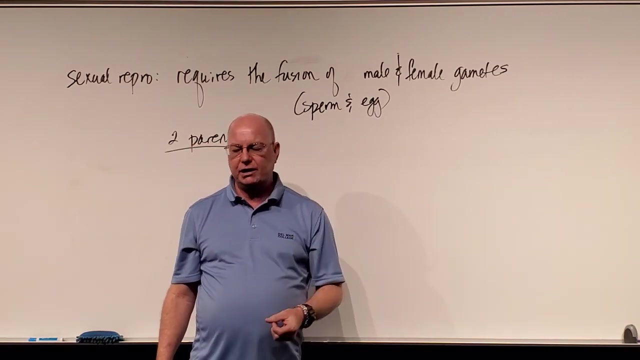 or chemical comes in and wipes out a whole segment of the population. you might have one that has a unique set of genes and gene products and proteins that allow it to survive- to survive a toxin or survive an illness. some people have a natural immunity to certain illnesses. because of their genetic makeup and that results from sexual reproduction. so again, the advantage of asexual reproduction is rapid reproduction, to increase in number rapidly. the disadvantage is they're genetic clones, so if one of them is susceptible to some other chemical or product in the universe, they are all susceptible to it. 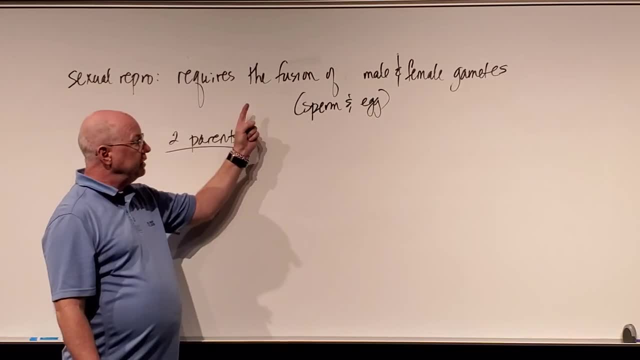 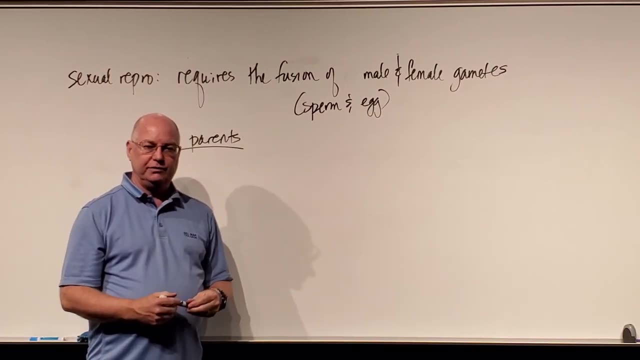 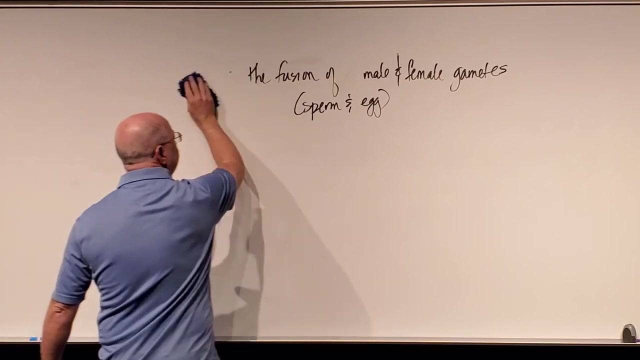 asexual reproduction. the advantage is it's slow. you have to have the right partners. the advantage is it provides a lot of genetic variation to increase chances of survival under changing conditions. now, when we talk about two organisms or when we talk about the offspring of two organisms, 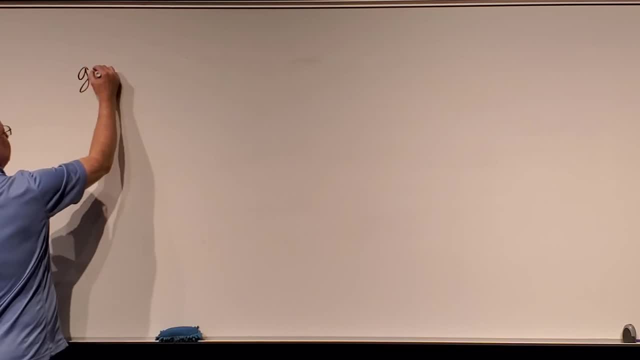 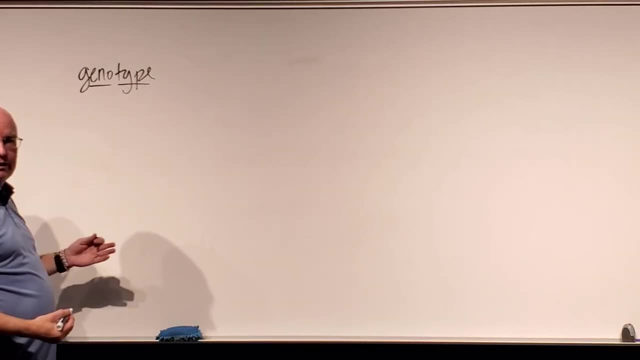 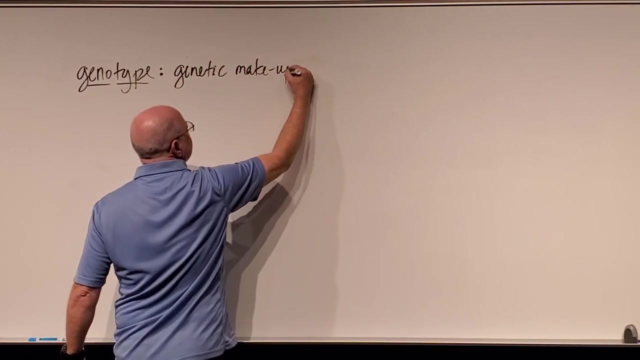 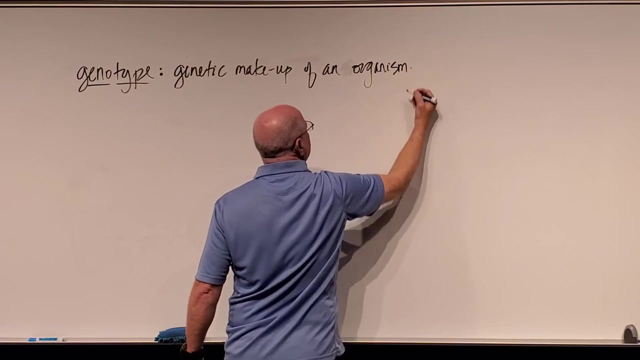 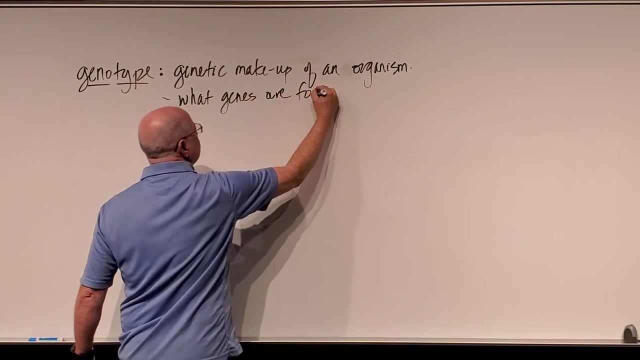 or of any organism if they produce asexually. we're going to talk about what's called the genotype, and I think of this as the types of genes in the organism. the genotype is the genetic makeup of an organism, which is really what genes are found in its genome. 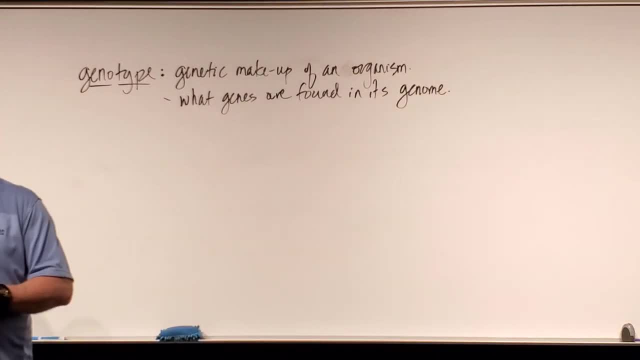 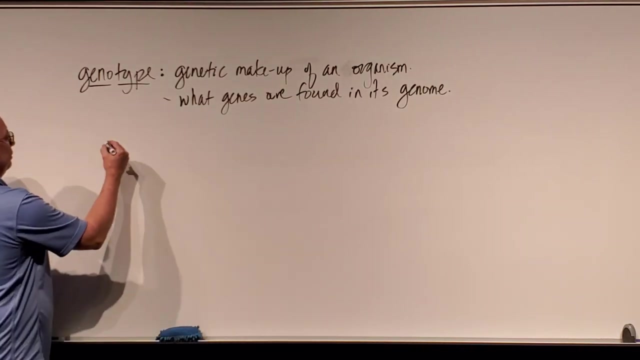 and we'll define what a genome is, but it's the entire genetic makeup of an organism, all the genetic information. but the genotype is what is the genetic makeup of an organism, or what genes does it contain in its DNA or in its RNA, if it has an RNA genome? 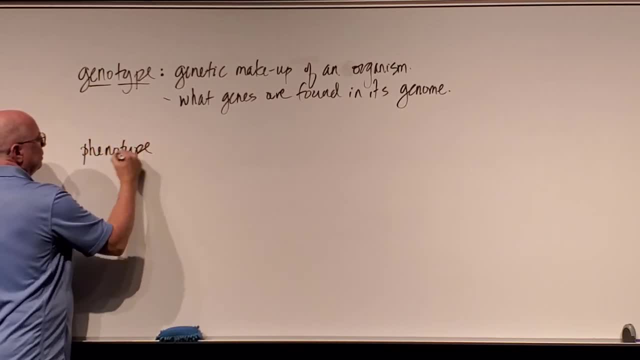 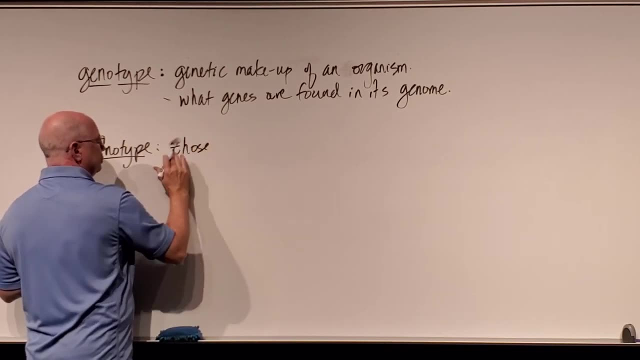 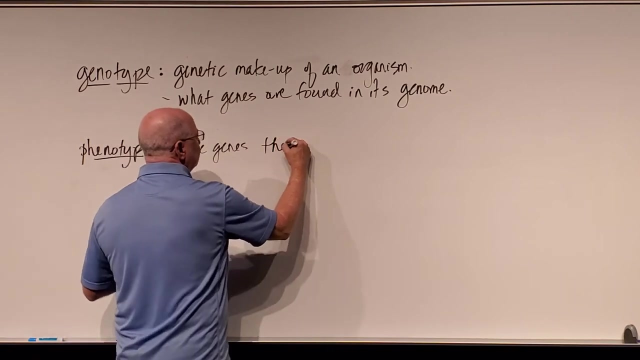 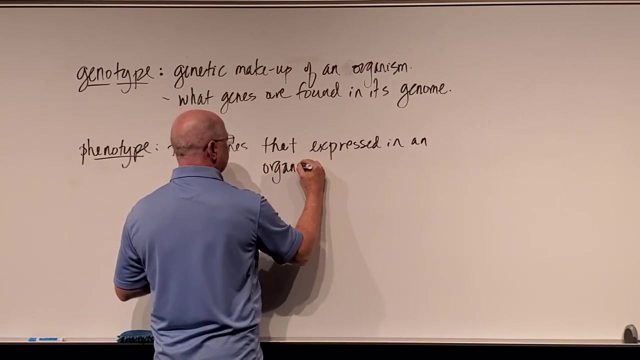 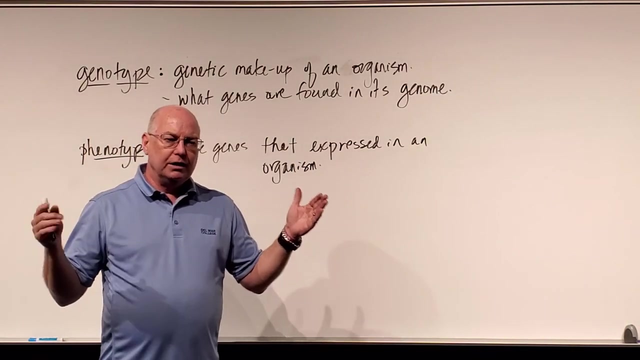 like we're going to learn. the phenotype is those genes- sorry, my pen and chip is a little off- those genes that are expressed in the organism. so when we talk about a genotype of an organism, we're talking about what genes does it contain? not always are those genes expressed. 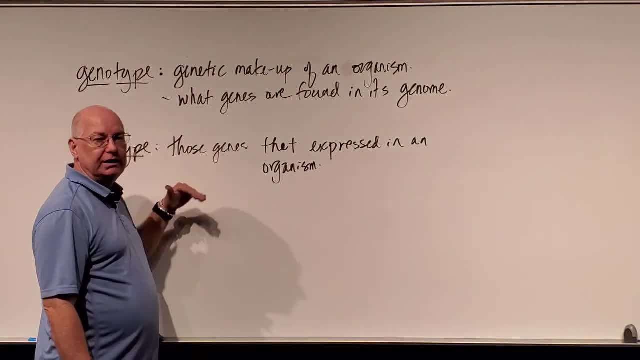 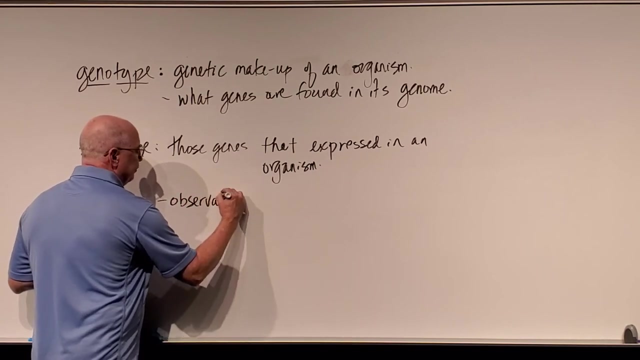 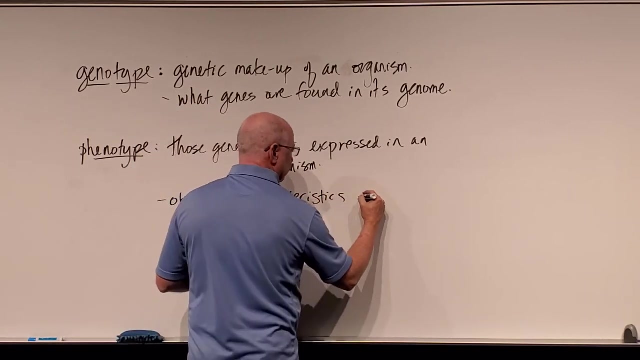 the phenotype is what you see in the organism, which gene is expressed and this gets. this requires us to sort of um go into some complex genetics and I'm not going to do that now. but we also define this as the observable characteristics of an organism. what genes do we see? 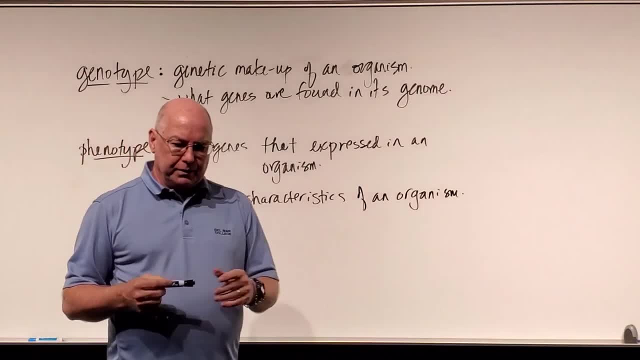 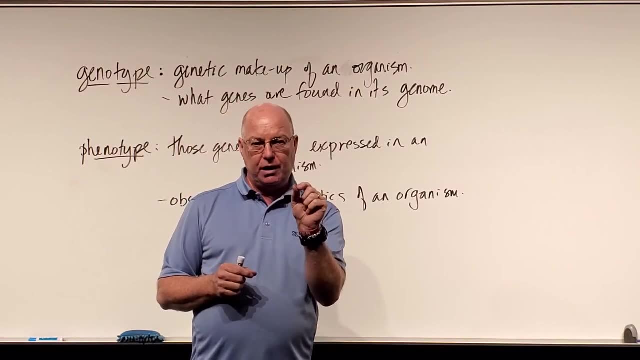 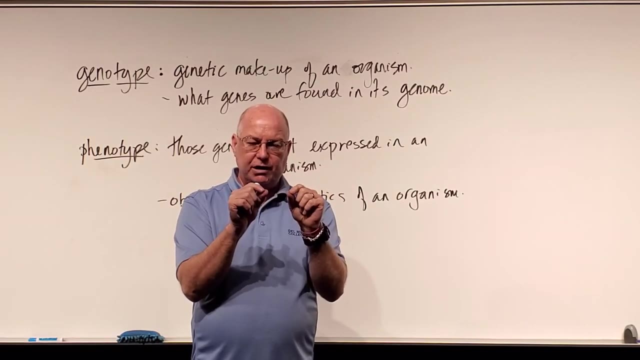 being expressed. for example, if you have a person that has carries, the gene, the allele, the specific version of a gene called an allele for blue eyes and brown eyes, because of the rules of genetics and how genes are expressed and what we call dominance and recession, that person will express. 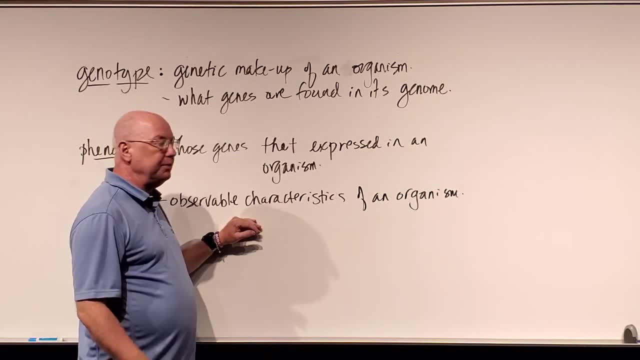 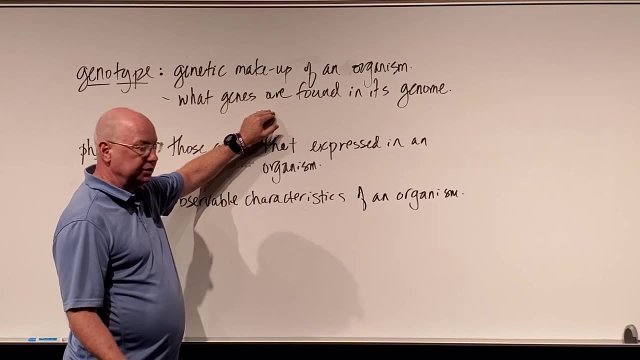 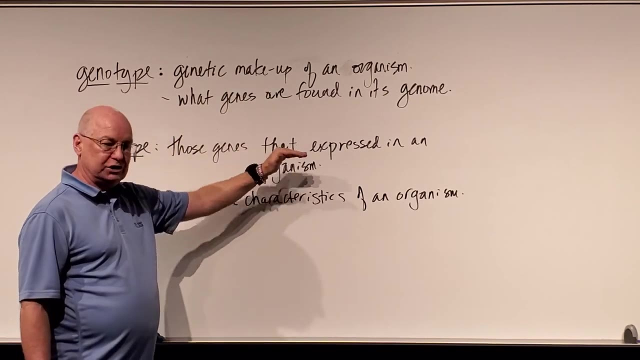 their phenotype will be that they have brown eyes. the genotype would be is that they have the gene for brown and blue eyes. but the blue eye gene is not expressed. it doesn't show up in the phenotype. the genotype is: what genes does it have? the phenotype is what genes are expressed. 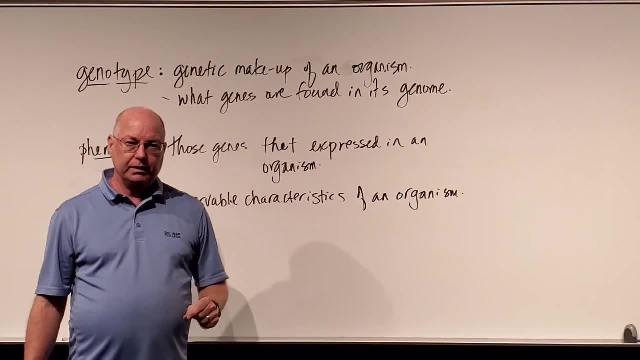 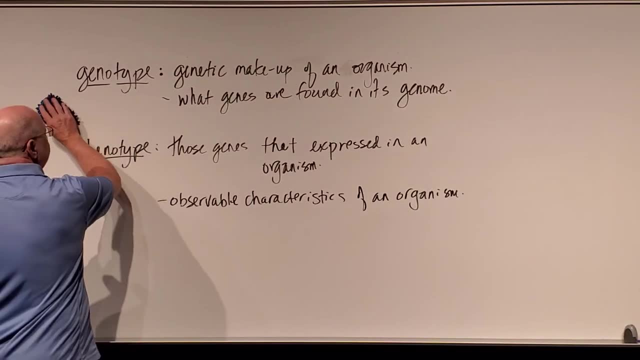 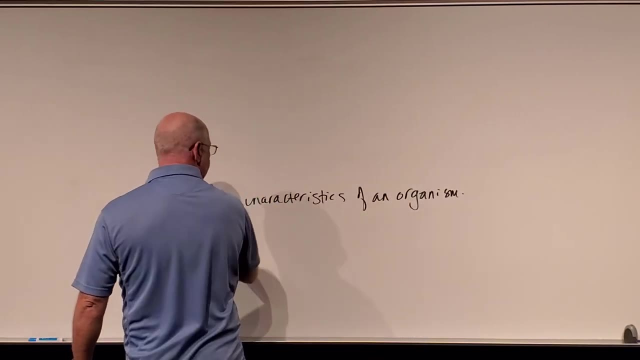 do we see in the organism, okay, so I hope that makes sense. now a couple of other terms that we're going to use, okay, and I'm going to come back to some of these in the near future when we do another chapter, but I'm going to try to tie this up. 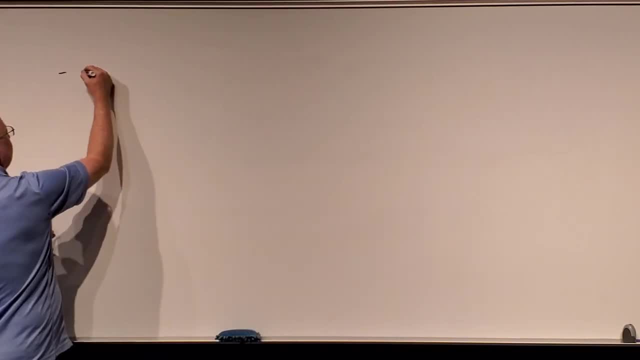 and finish up our definitions. now we're going to talk about a structure called a glycoprotein. okay, we're also going to talk about something called a proteoglycan. now, if you've had any biology or chemistry before, at least at Del Mar, you have to have freshman chemistry. 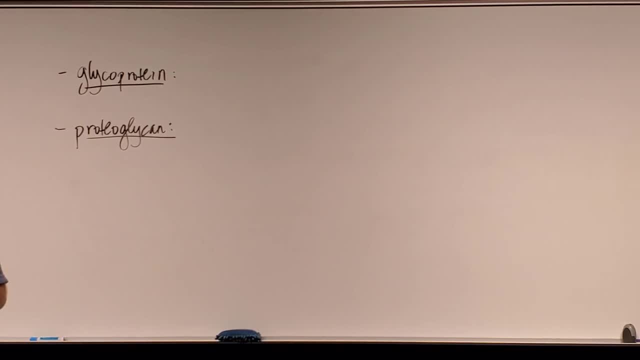 when we talk about a glycoprotein and a proteoglycan, there is a difference between the two. if you look at the name glyco, it always refers to sugar or carbohydrate, gluco and glyco. anytime we see something referring to gluco or glyco. 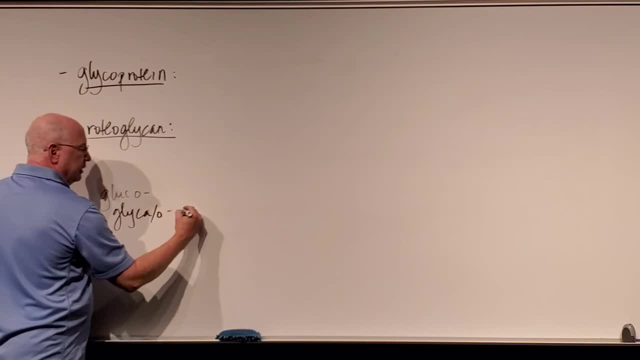 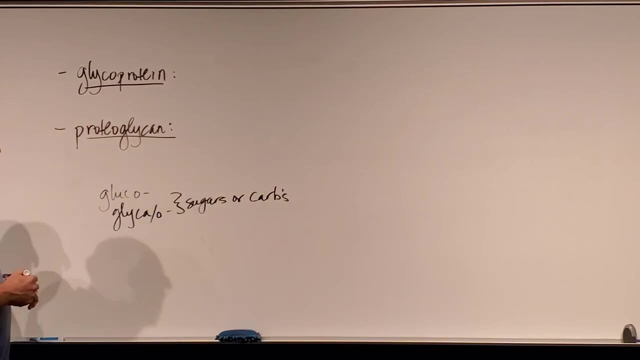 or glyca slash, glyco. it's usually something to do with sugars or carbs, sugars or carbohydrates. anytime we see proteo, we're talking about proteins. well, it turns out that there are some compounds that are made out of sugars and proteins, and they fall under two categories. 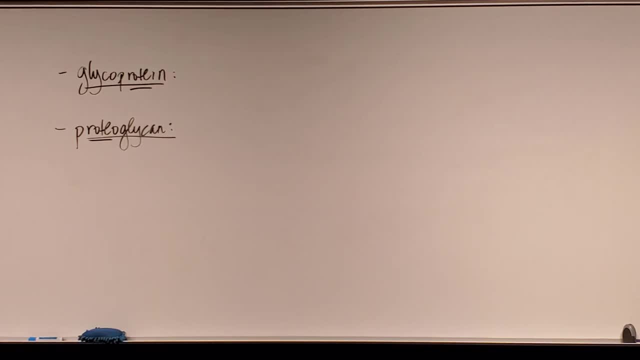 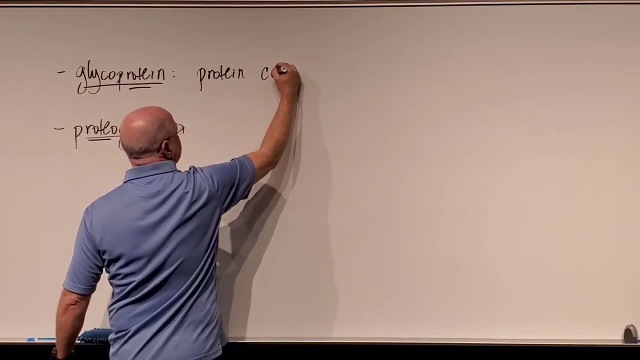 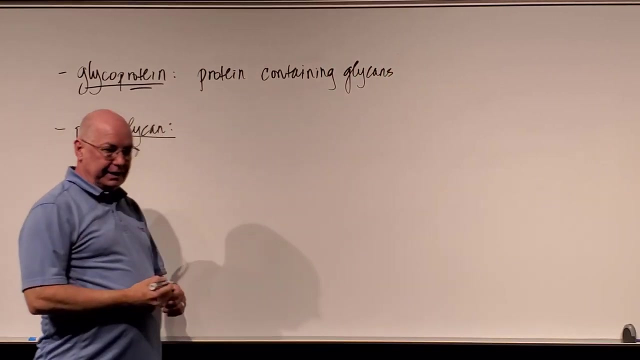 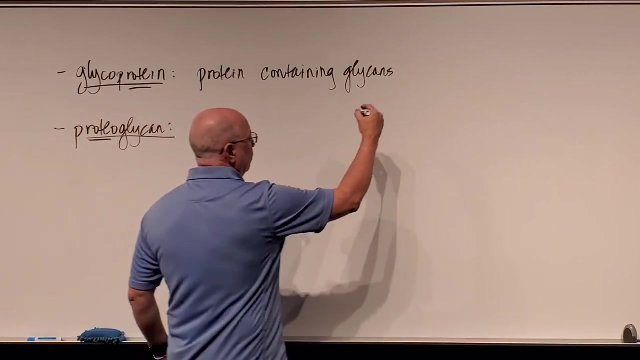 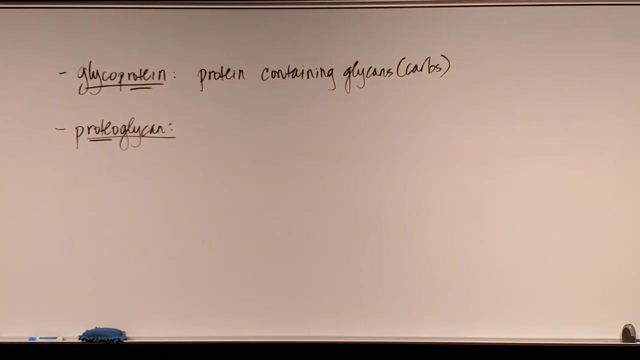 so a glycoprotein technically is defined as a protein containing glycans. okay, now, that's kind of obvious. that's why it's called a glycoprotein. but those glycans are carbohydrates that are associated with that protein in a chemical bond. so proteins that have 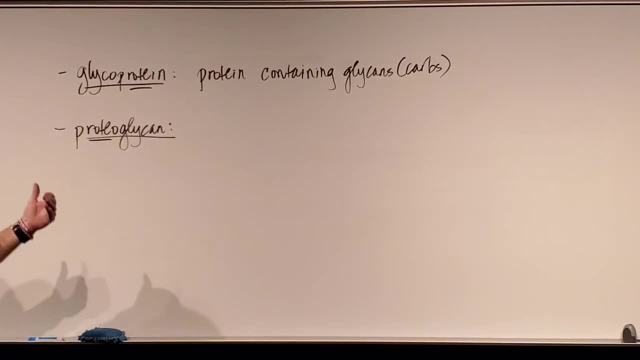 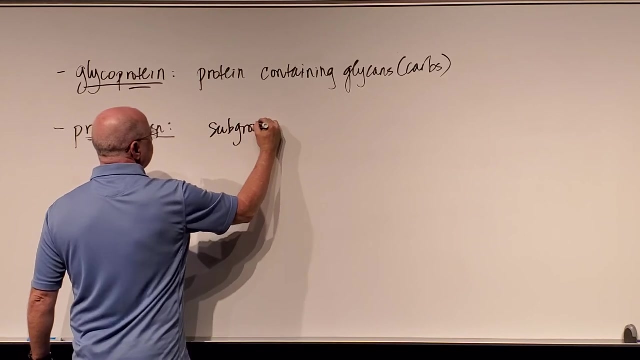 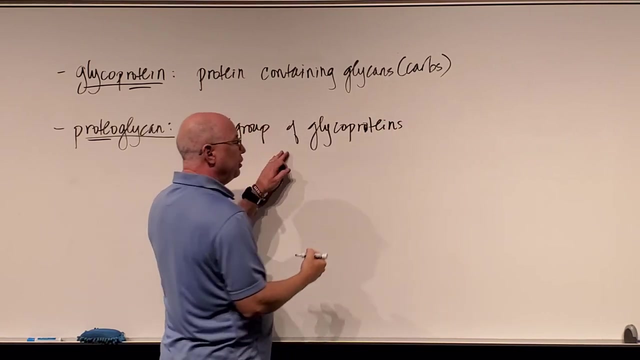 sugars or carbohydrates are called proteoglycans, called glycoproteins. now, the difference between that and a proteoglycan is in a proteoglycan, this is a subgroup of glycoproteins. okay, so these are glycoproteins, but they have 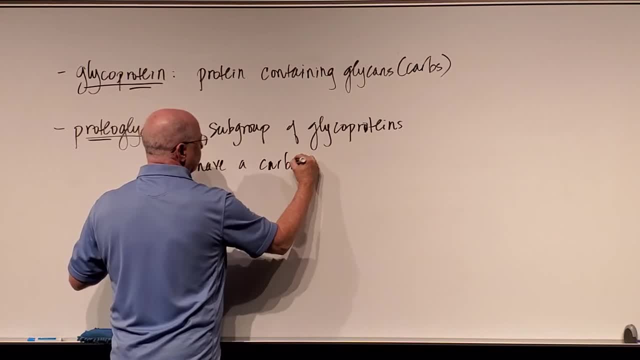 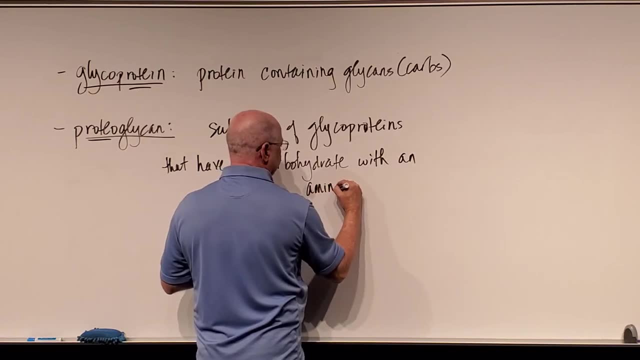 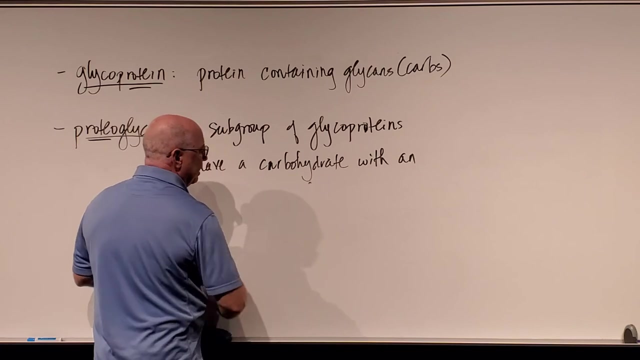 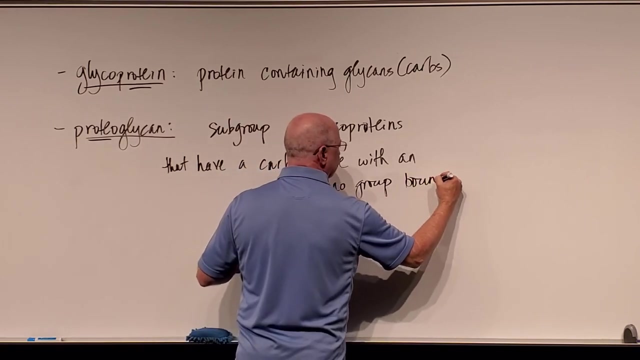 a carbohydrate with an amino acid bound to them. they have a bound amino acid to the sugar. okay, alright, I'm sorry, I shouldn't even say amino acid. you know when I think about it, it really is an amino group bound to them. okay, so a proteoglycan. 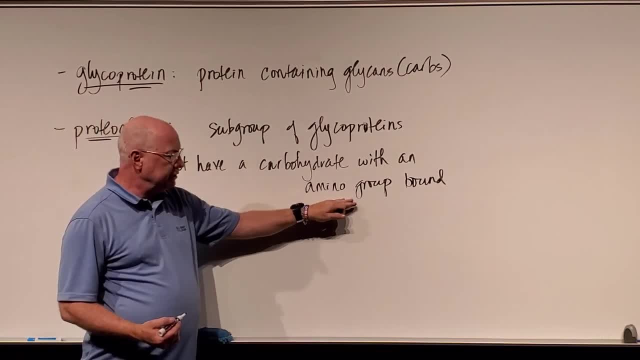 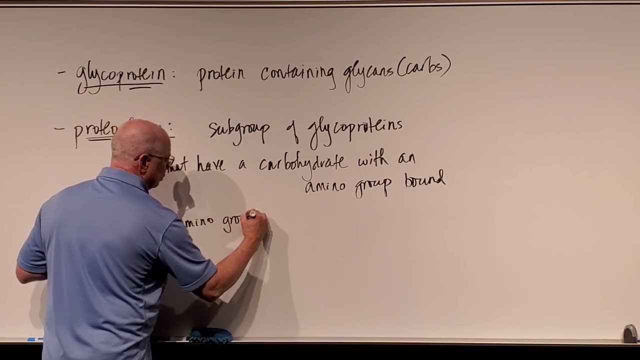 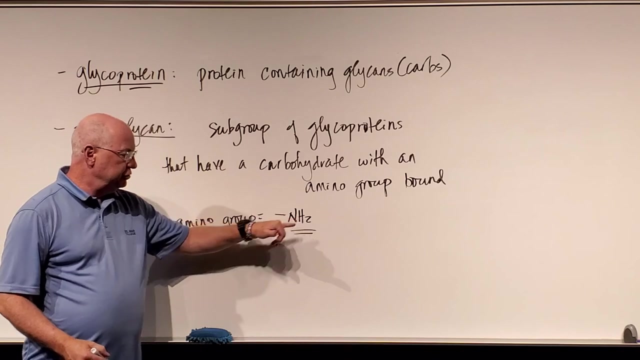 is a carbohydrate or glycan that has an amino group bound to it. so when we talk about an amino group, an amino group to a chemist means anything that has this, an NH2 group associated with it, a nitrogen and two hydrogens is called an amino group. 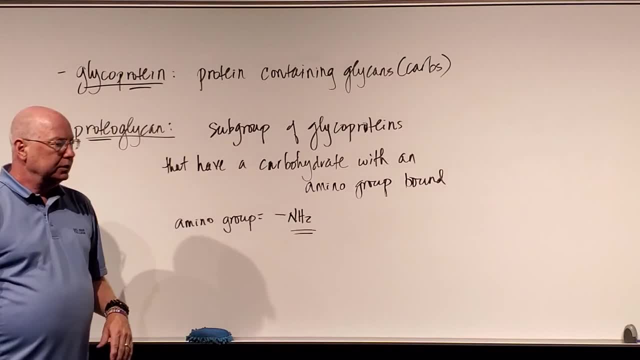 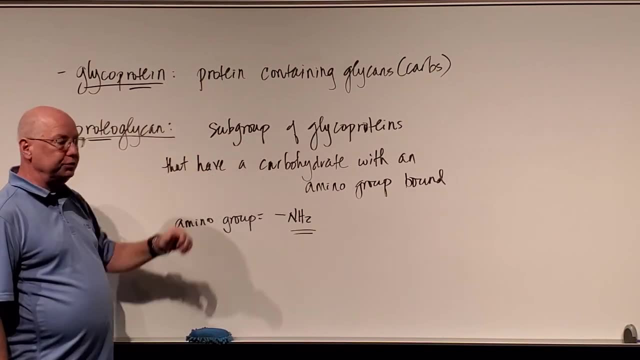 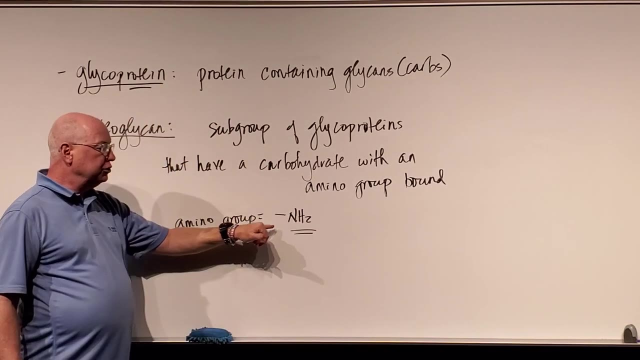 and this would represent where it would be bound to some other molecule. so proteoglycans are carbohydrates with an associated amino group. they are a type of glycoprotein, but there are glycoproteins where we have sugars and proteins associated with each other. 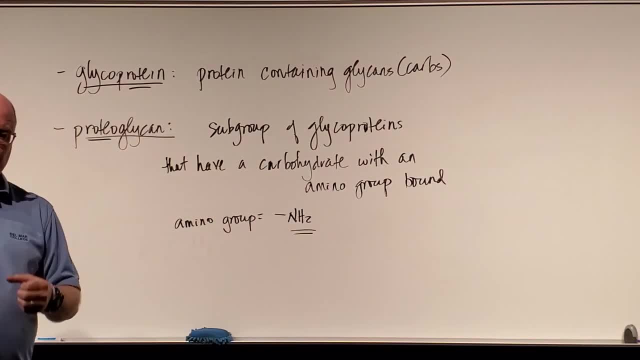 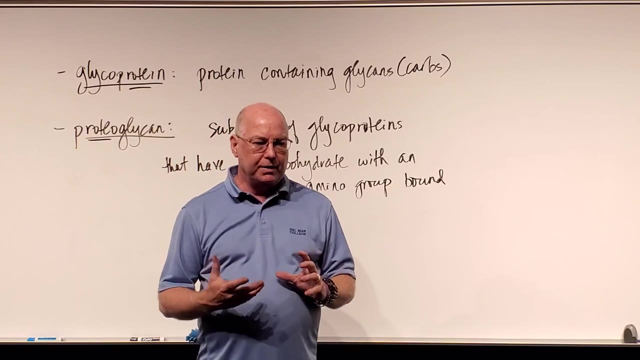 where the sugar does not have an amino group associated with it. it's just a sugar associated with a protein. I know that's a little confusing and very closely related, but nonetheless those are two of the definitions that you need to know, so now I hope that at least you have some definitions. 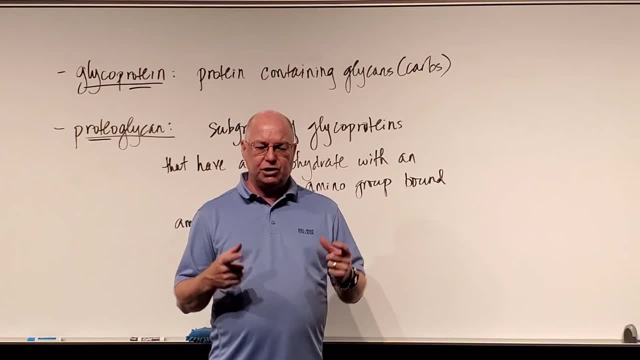 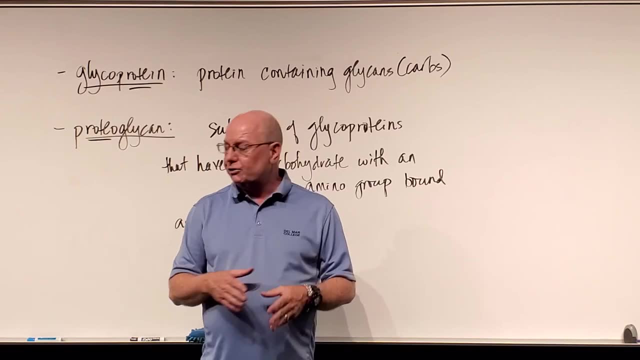 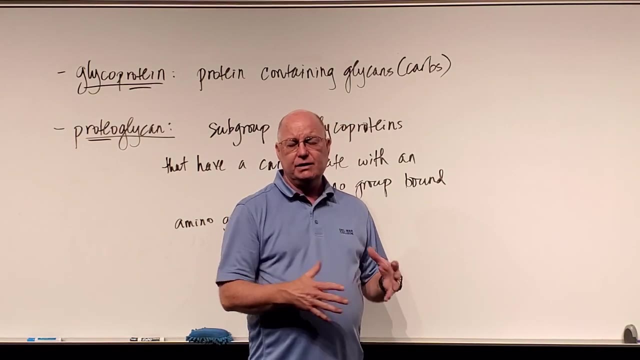 under your belt. you're not just memorizing definitions, but these definitions are going to be essential for when we start talking about other topics. the hard part about microbiology is sometimes I'm going to talk about a subject early on and then later on we're going to make sense of it. 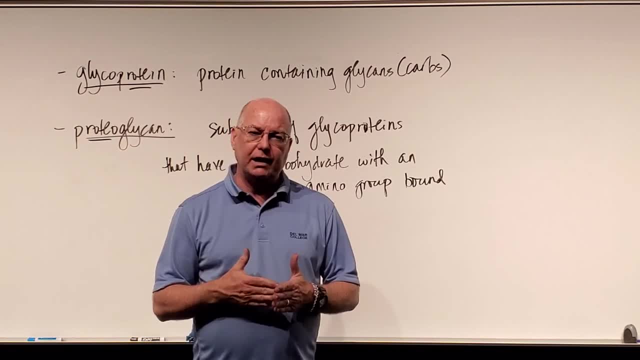 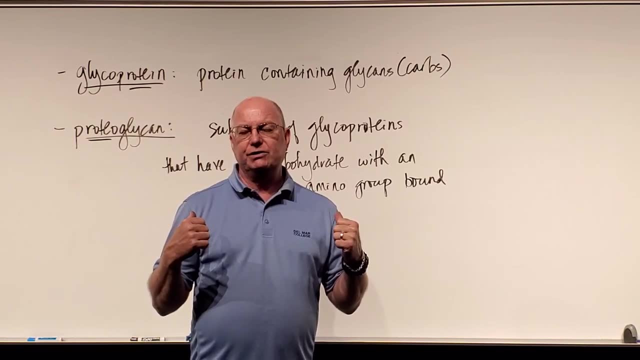 but I wanted to get this list of definitions out. if you're enrolled in my class, or pretty much any microclass across the US- a lot of these definitions are going to appear on your first exam. so I suggest you start learning these definitions and see what the words mean. 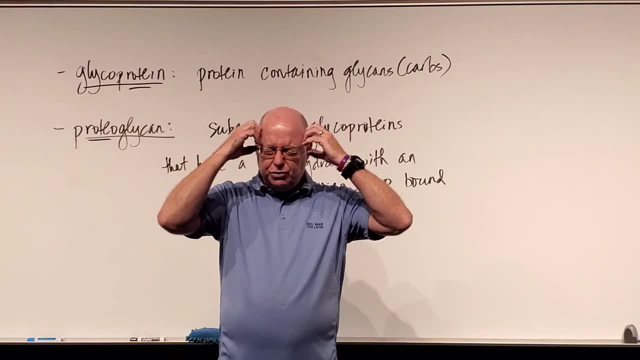 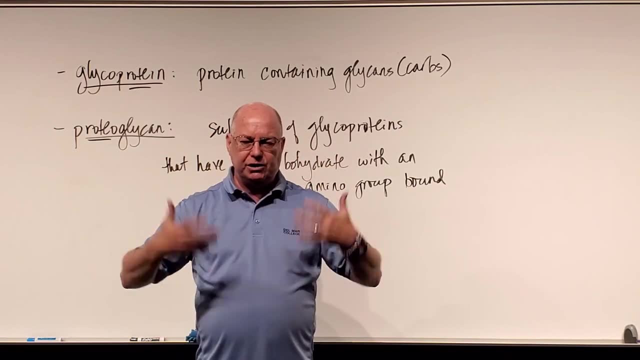 so that in the future, when you see a specific word like genotype, you can picture: oh, it's the types of genes in an organism. when I say phenotype, you picture in your mind: oh, those are the genes that are being expressed, that we see expressed in the organism.